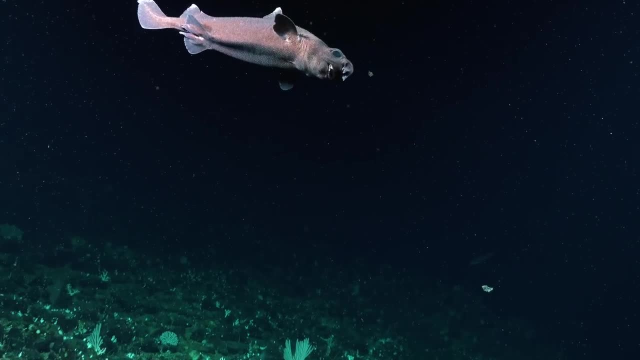 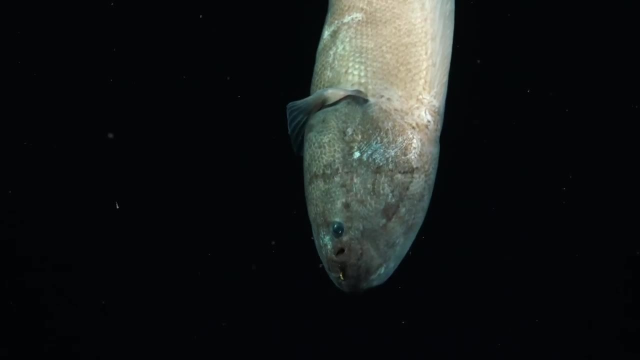 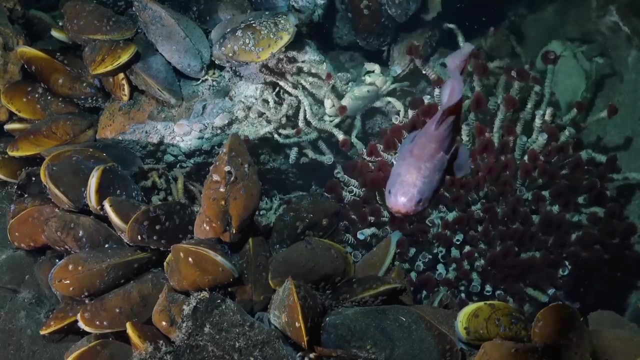 And it may hold the key to understanding our planet's past, present and future. It's a world of perpetual darkness, home to obscurities, adrift in an endless void, or clinging to alien oases where the processes, inhabitants and environments within remain poorly understood. 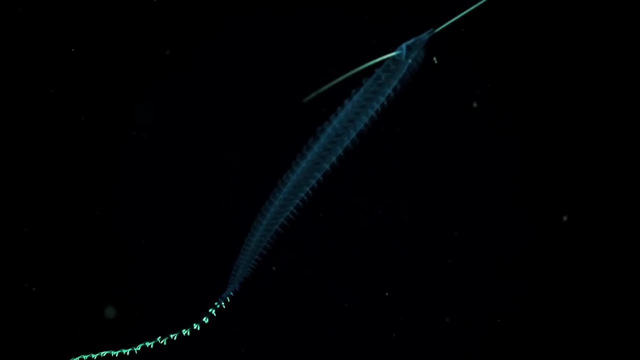 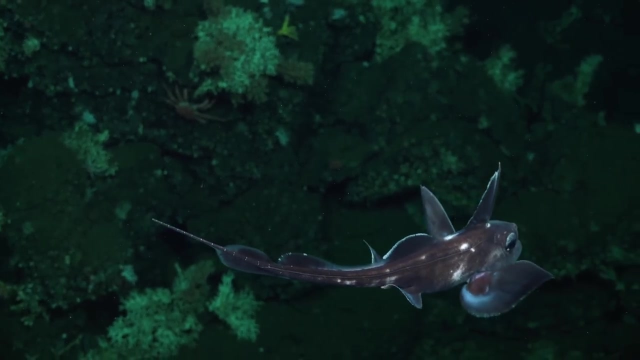 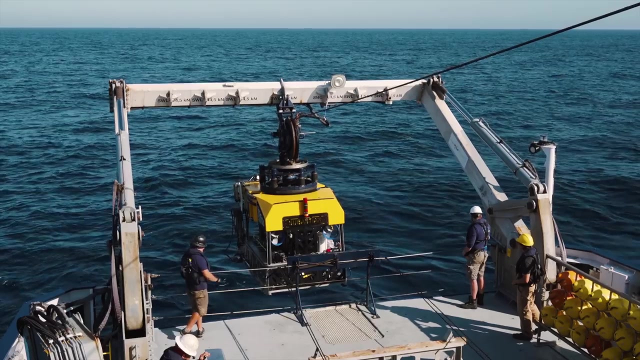 to this day, These are the least known areas of our planet, But this is beginning to change. In 2009,, the philanthropic, non-profit Schmidt Ocean Institute was established with a mission to advance ocean science through the use of state-of-the-art technology. 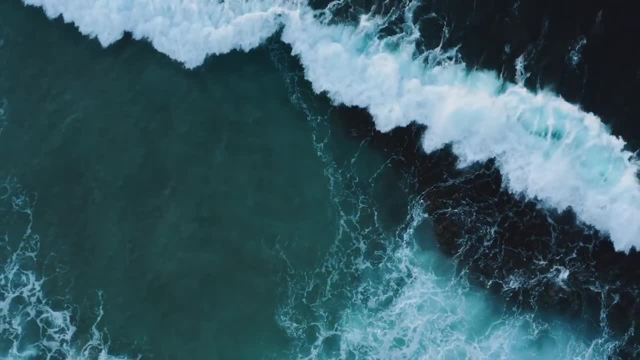 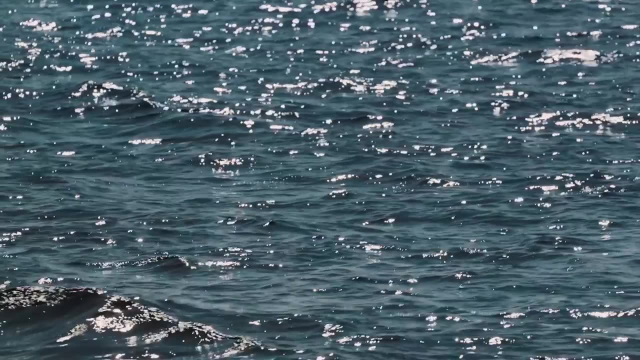 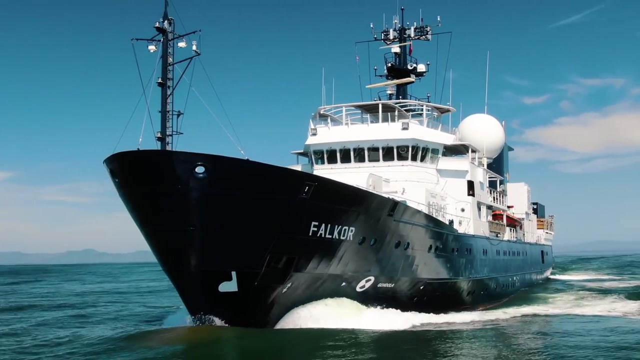 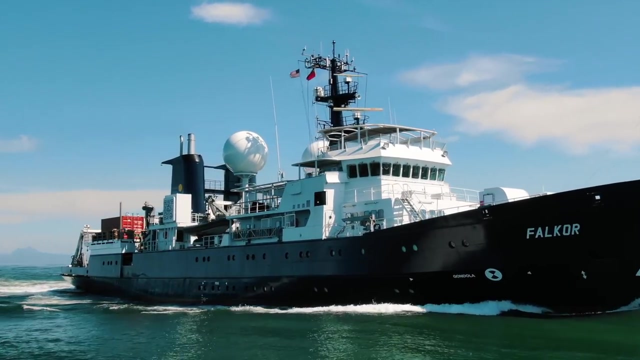 And open sharing of knowledge to foster a deeper understanding of the world beneath the waves. Across eleven years at sea, scientists on board their first vessel, Falcor, discovered never-before-seen wonders throughout the world ocean. But the ambitions of the institute have outgrown Falcor's capabilities, And so, in 2023, the 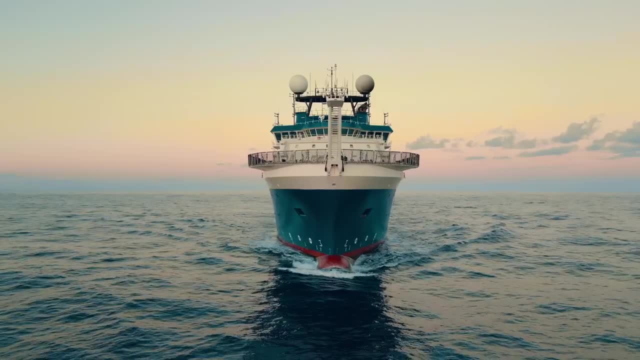 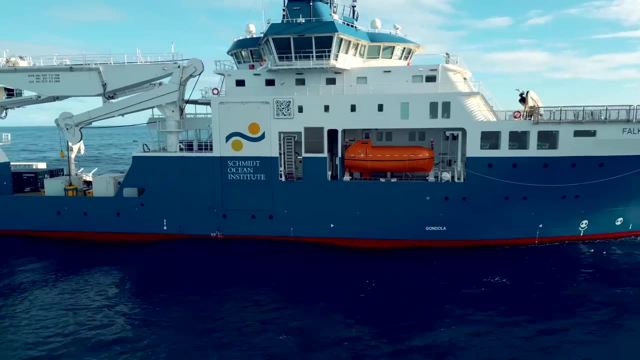 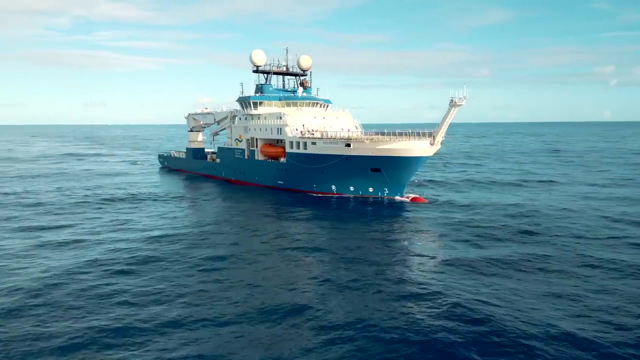 institute set sail its new vessel for their boldest year of discovery to date. This is Falcor II, Their newly refitted 110-metre global-class research vessel, purpose-built to push the frontiers of deep ocean exploration once and for all. 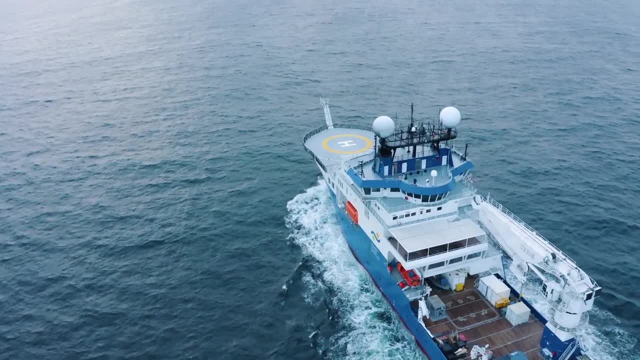 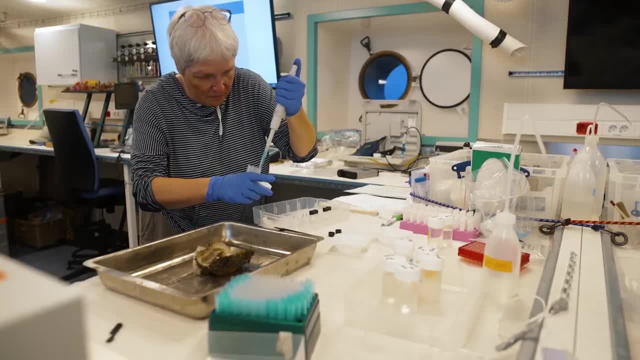 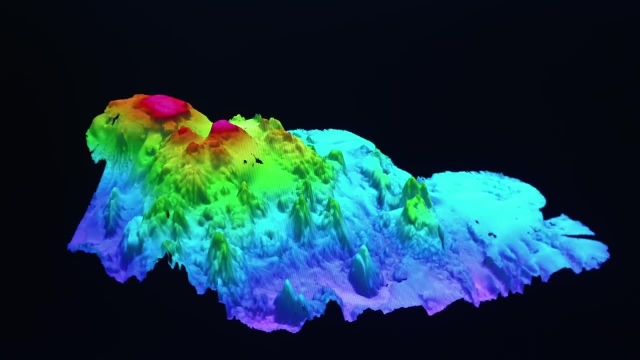 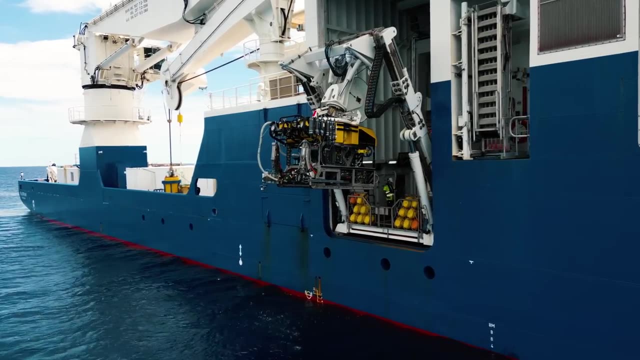 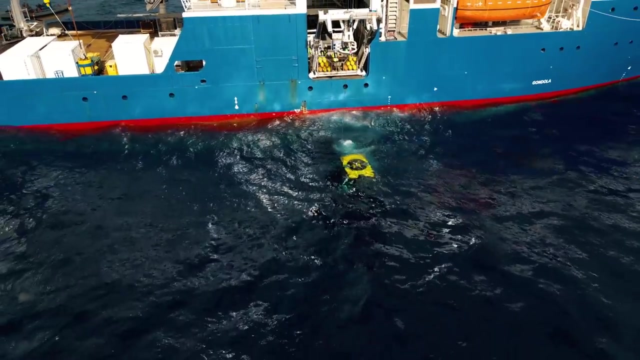 An 150-ton crane, Over 200 square metres of lab space, high-resolution sonars for ocean mapping And a hangar from which the institute's remotely operated vehicle is deployed- ROV Sebastian, A robot capable of diving to 4,500 metres below the ocean surface. 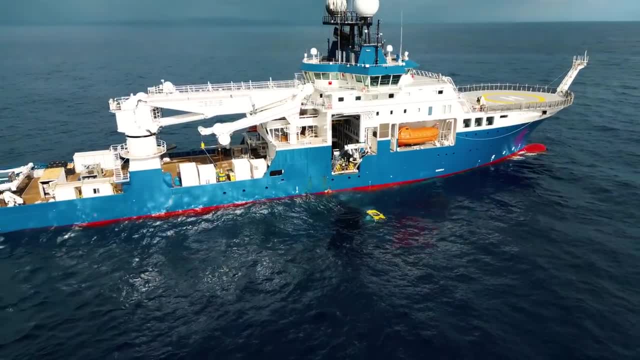 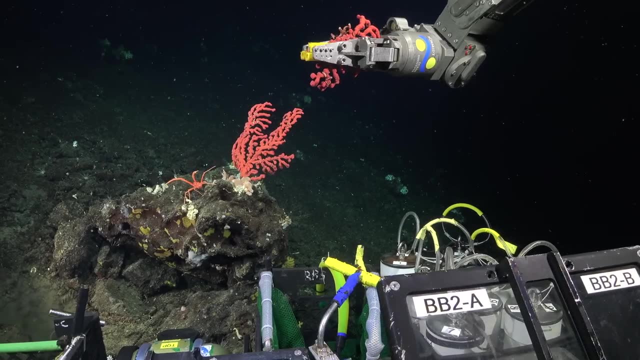 Where, once, the riddles of the depths could only be tackled through trawls and weighted lines, Now a suite of sensors and a 4K camera open a window into this realm for all to see. Manipulator arms. allow the teams to collect samples. 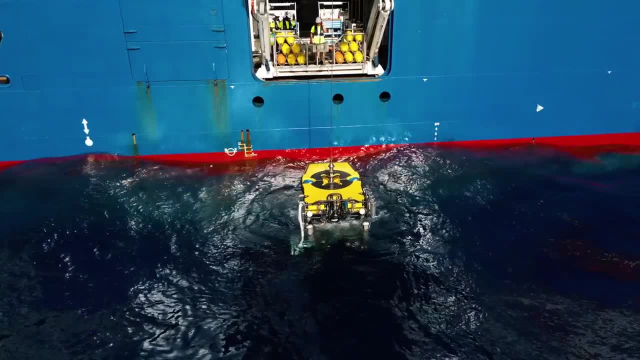 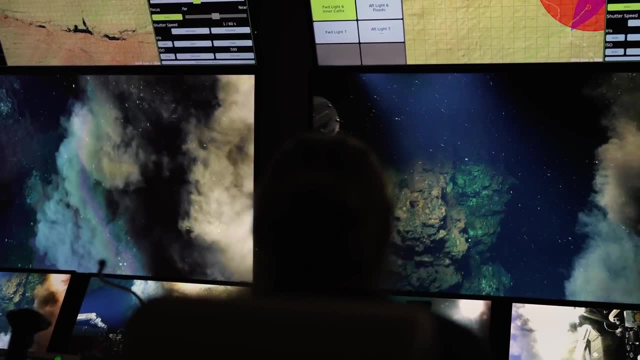 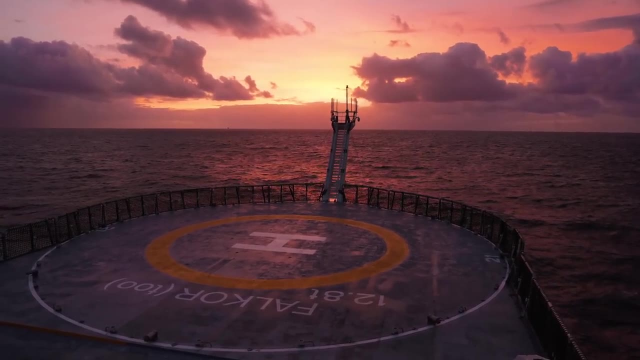 And an umbilical cable tethers the ROV to the ship, supplying power And relaying data and imagery to the surface, where it's broadcast around the world in real time, Inspiring a generation to look to the depths. Throughout 2023, across nine expeditions spanning wildly different environments, teams. 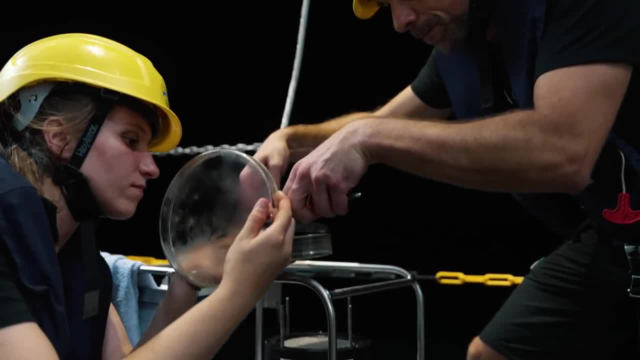 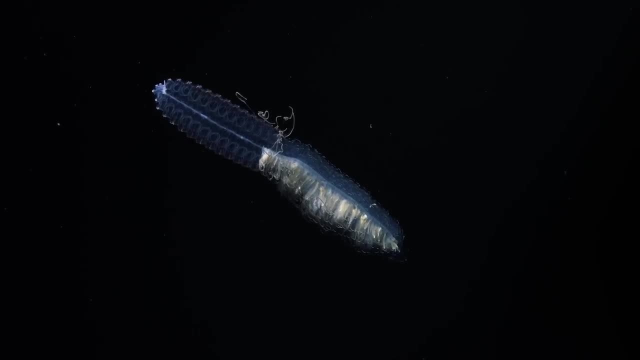 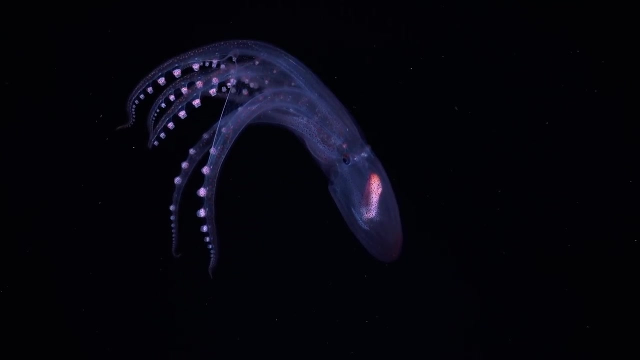 on board FALCOR2 have deployed new technologies, systems and approaches to map the seafloor and uncover new frontiers of biodiversity in the deep's most extreme habitats. In FALCOR2's first year alone, the vessel has already allowed scientists to make ground-breaking 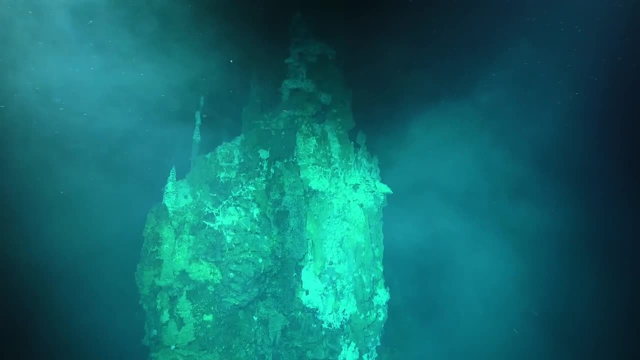 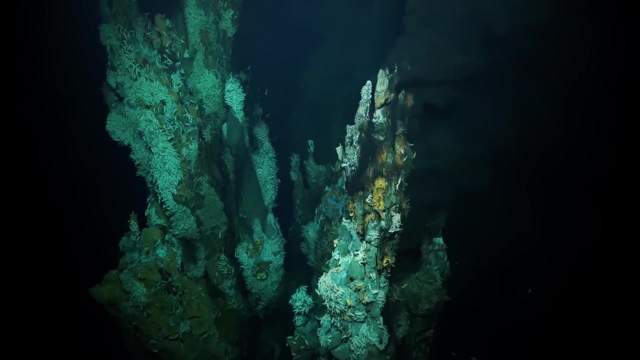 discoveries that are redefining our understanding of life in the deep. In FALCOR2's first year alone, the vessel has already allowed scientists to make ground-breaking discoveries that are redefining our understanding of life in the deep, Living cities at depths of two kilometres or more, never before seen. 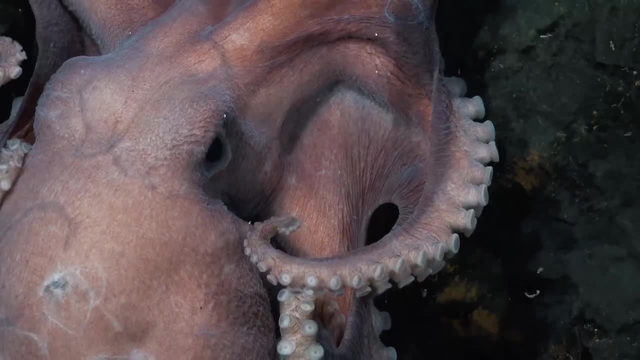 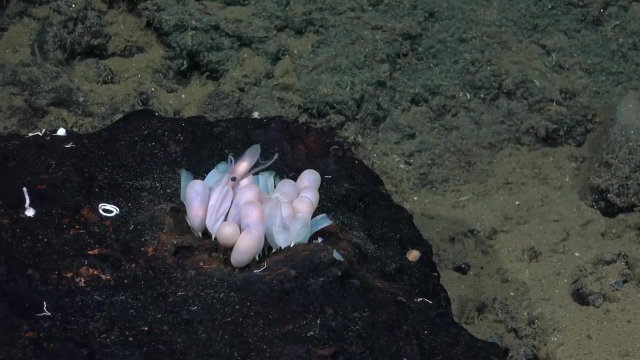 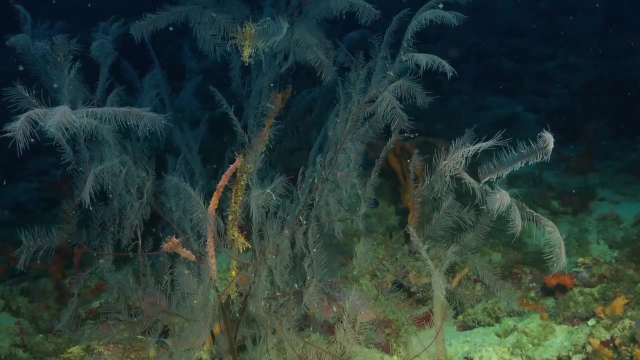 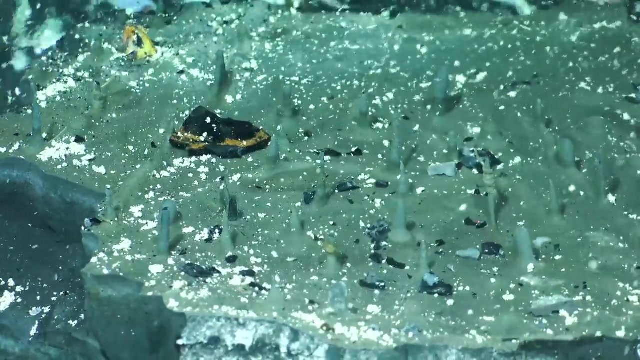 by human eyes, Active nurseries where little-known species gather in great abundance to brood And spawn Elsewhere new species surviving in the dark, And so it's all the same. And an entirely new ecosystem where a sanctuary of life thrives in an underworld beneath the seafloor. 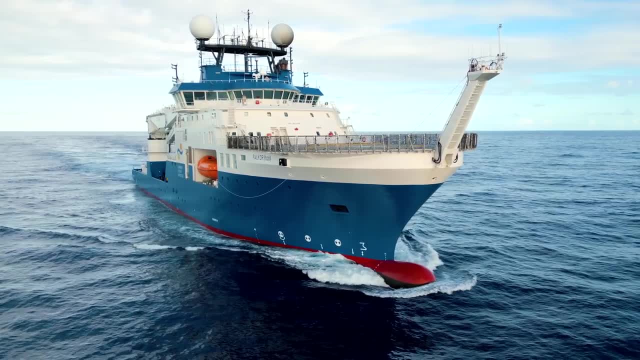 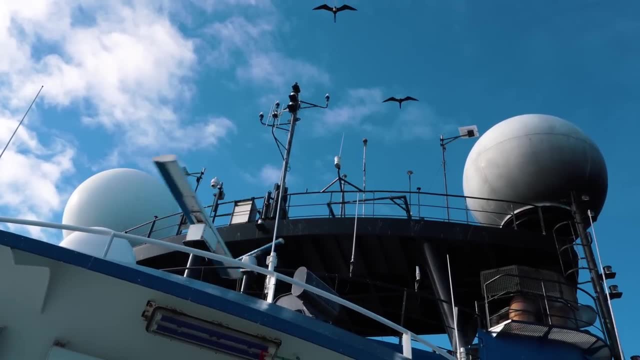 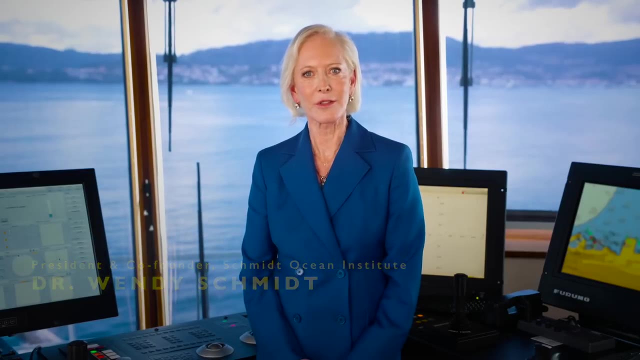 Hello and welcome aboard Falkor II, our dynamic, inclusive and interdisciplinary ocean research and exploration vessel. The mission of this vessel is to foster the discoveries needed to understand our ocean, sustain life and ensure the health of our planet as you boldly explore our unknown ocean. 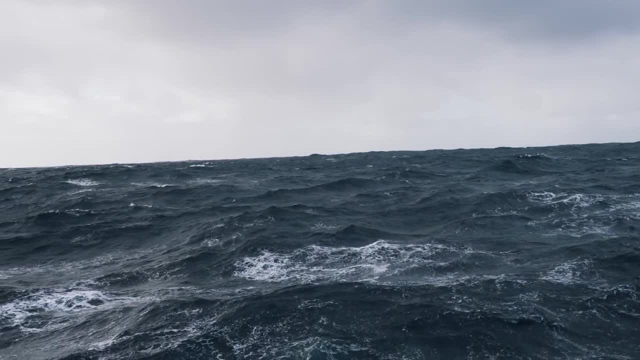 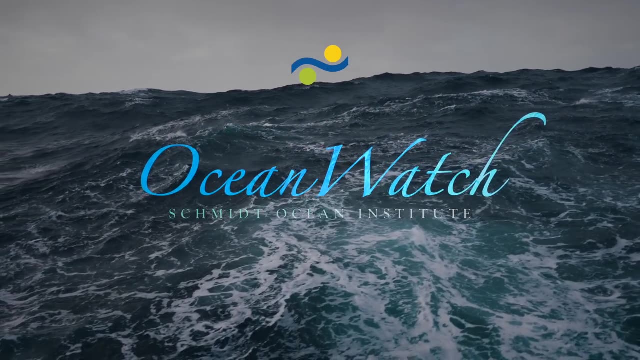 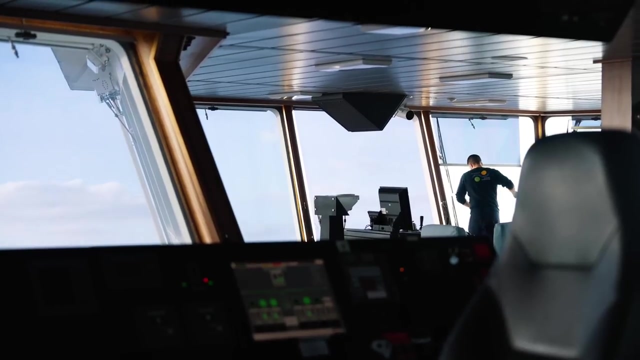 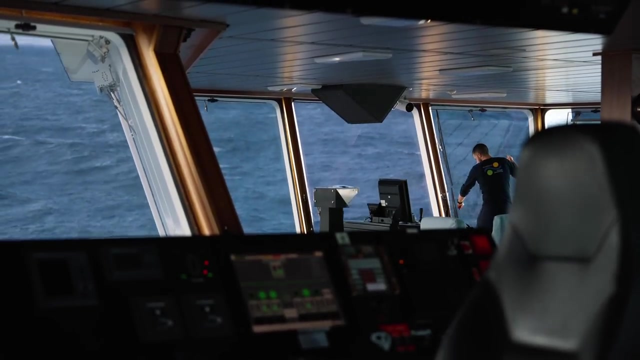 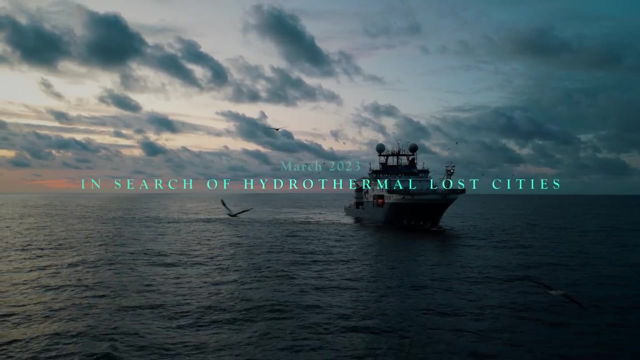 These are the stories of Falkor II and its first chapter into a lifetime of exploration. Falkor II's first tale is one of discovery. It's March and the vessel is bound for the Mid-Atlantic Ridge, a site where, 23 years prior, scientists discovered a system of hydrothermal vents unlike anything seen before. 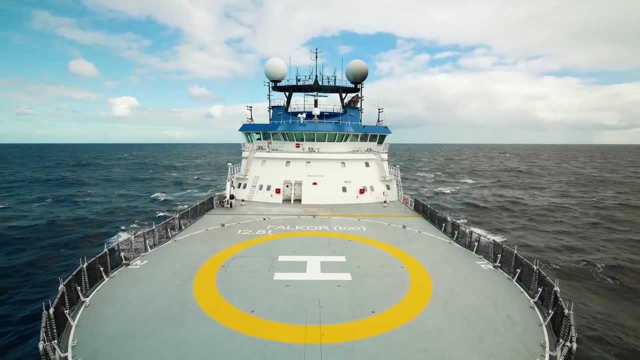 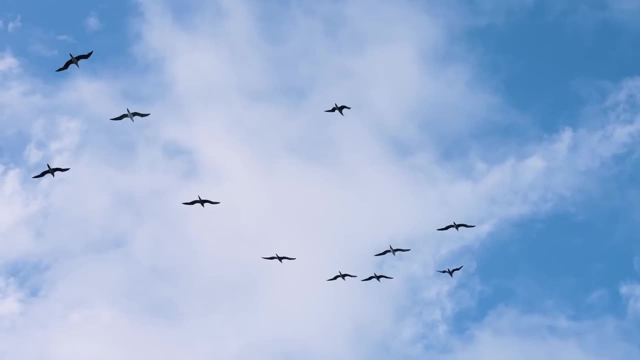 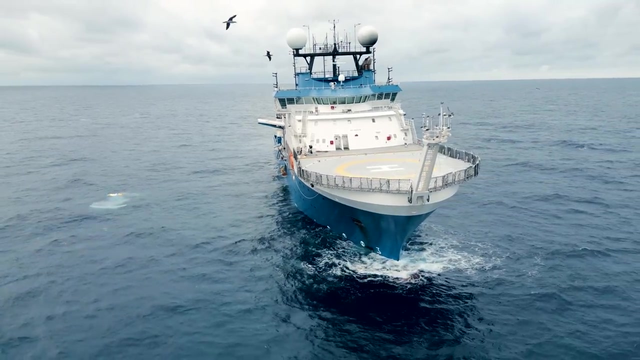 The vent system was named Lost Sea, And the team on Falkor II were on the hunt for more like it, Tracking down sites of potential venting through the combination of several high-tech strategies. The first step is to map with the ship so that we have a base map. 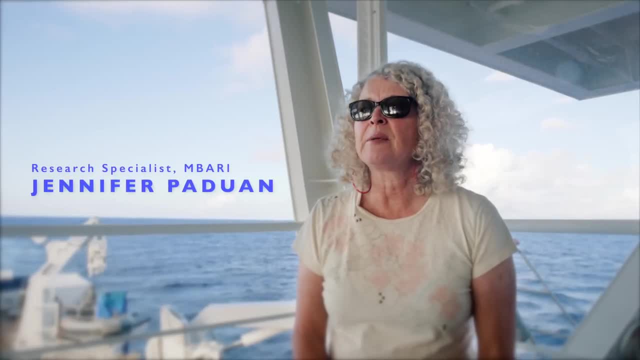 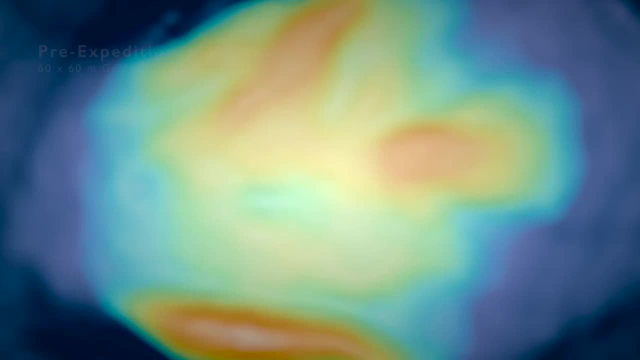 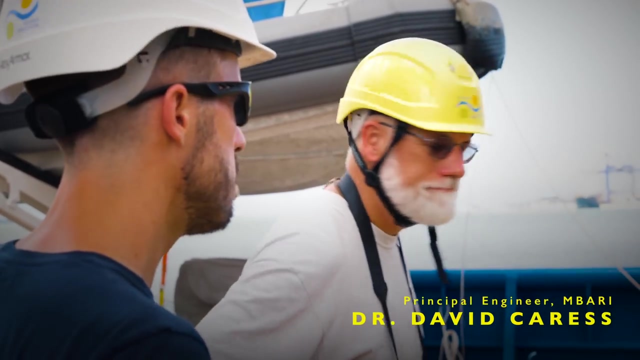 That also tells you where the ridge crest might be, or seamounts or fault zones, Things that create pathways for the hot water to travel from deep within the crust to the seafloor. That allowed us to lay out two AUV survey missions that would cover the parts of the volcano summit that were of interest. 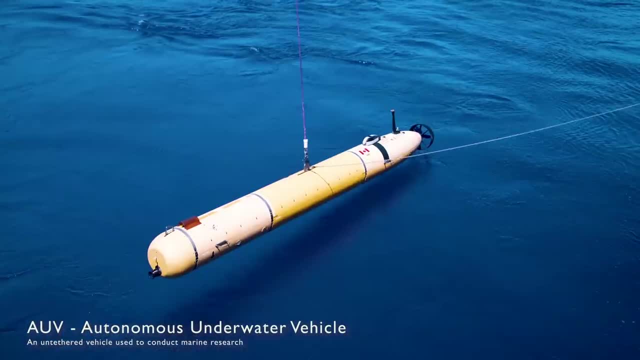 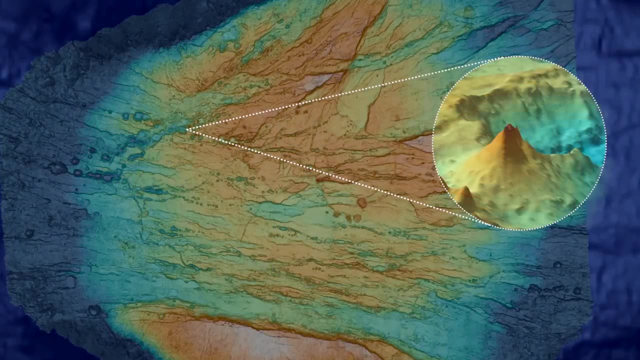 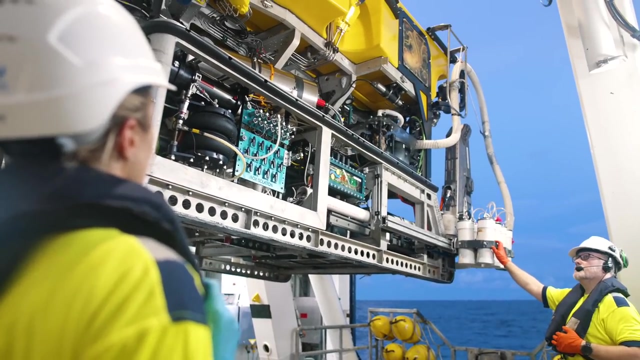 We had to put the AUVs in the water to get the one-meter resolution data. And then these mounds that are pretty broad but not all that tall, those showed up in the AUV data On Sebastian's very first dive from Falkor II at a previously unexplored portion of the Puy-de-Fols seamount. 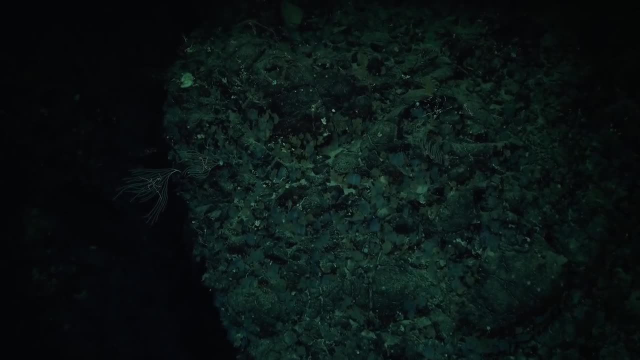 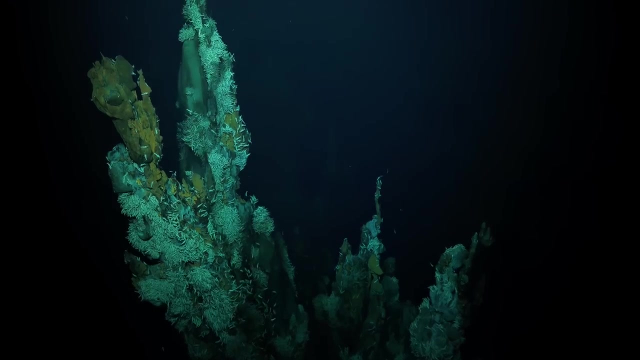 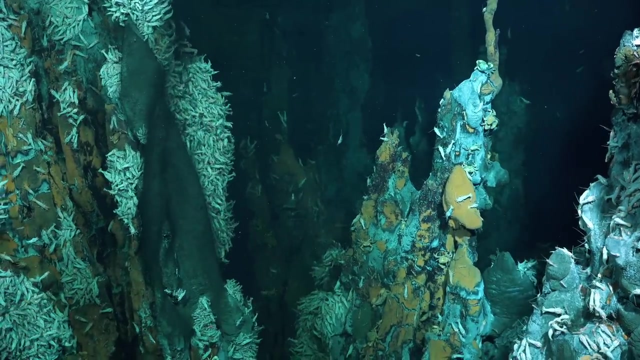 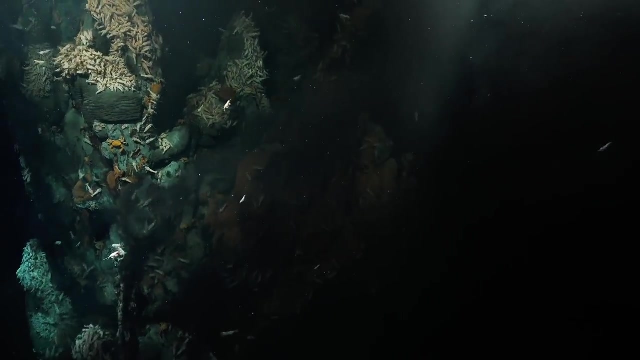 where the seafloor mapping data had pointed at the existence of vents, a set of silhouetted structures emerged from the gloom, Chimneys spewing thick plumes of dark smoke formed from the precipitation of sulphides. These are black smoker vents, ones that had never been seen before, and hosting vibrant life. 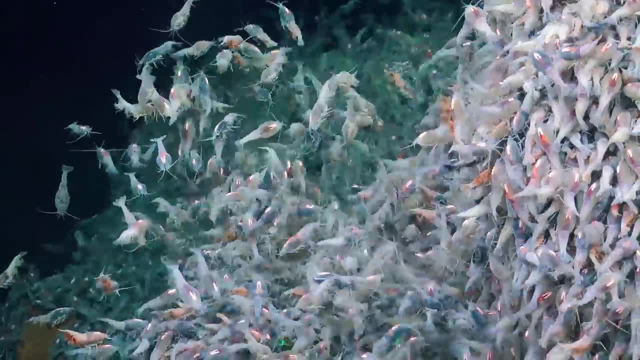 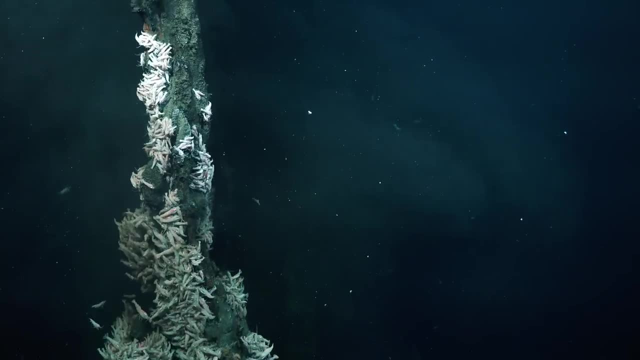 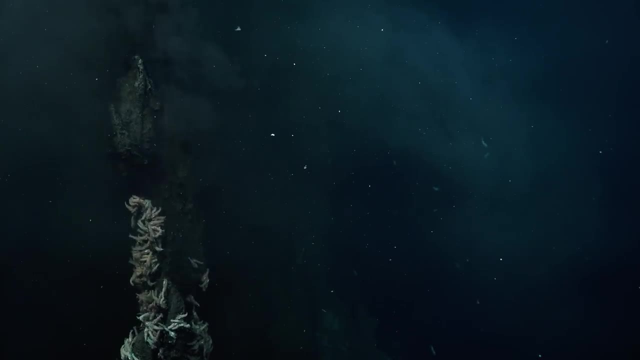 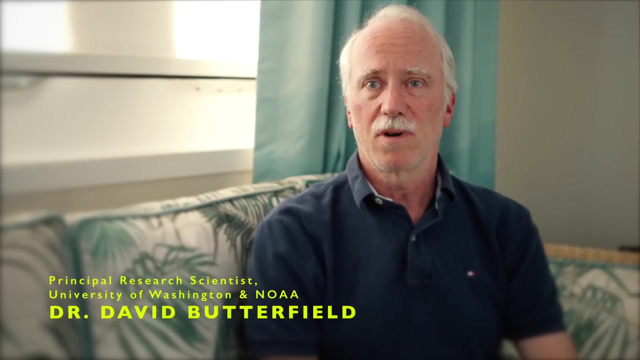 Hordes of swarming shrimp and hairy white yeti crabs, farming bacterial colonies on their shells, coexisting among chimneys of minerals and cathedrals of basalt. Every time we go down, we find not just one, but multiple high-temperature smoker vents. 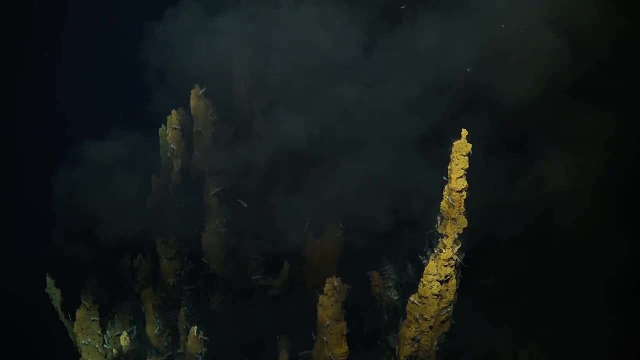 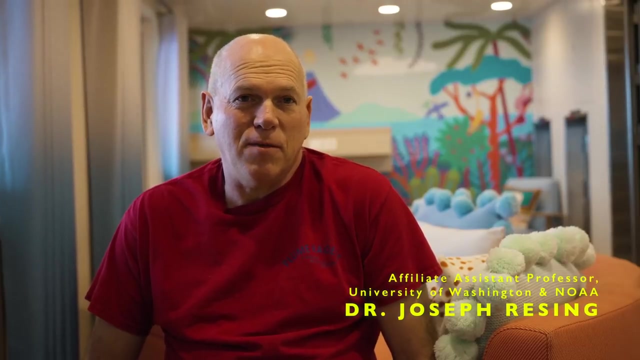 This place is obviously quite remote. That's the oceanography. You're just out here, seemingly in the middle of nowhere, But below us the seafloor is teeming with activity, teeming with life and features. You have the mid-ocean ridges, and they're big, They're huge. 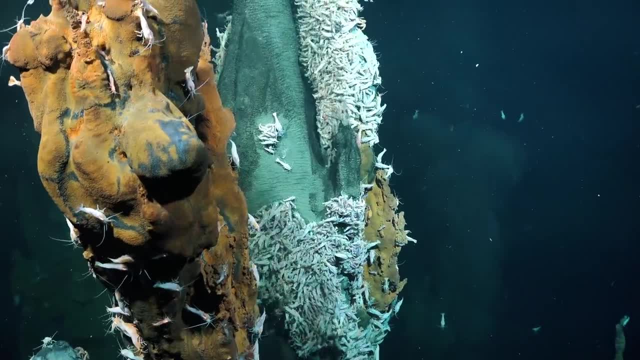 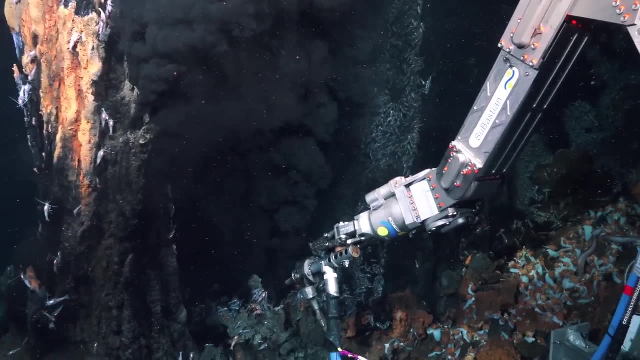 They're like some of the biggest mountain ranges on the face of the Earth. When we got on board, we felt like, as far as the ship was concerned, we could do any operation at any time of day or night, And we did. 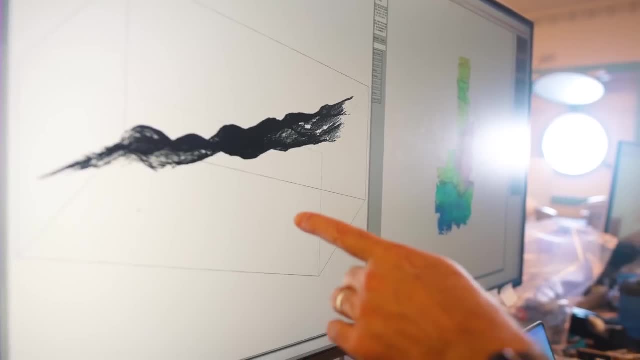 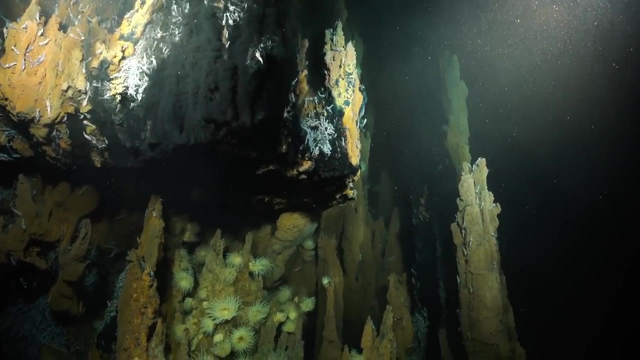 One of those dives. we got the map. Dave Kress looked at it and says, right, there, put the ROV down. We went 15 minutes and there we were. So yeah, no, that's not common. The chemical composition found at vents is thought to closely resemble the conditions. 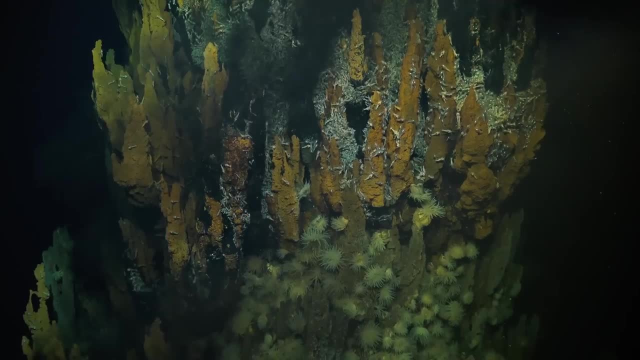 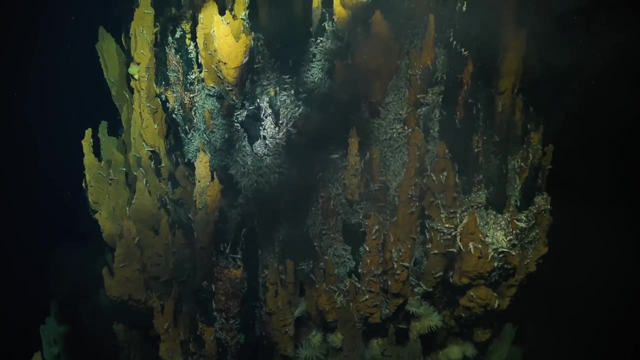 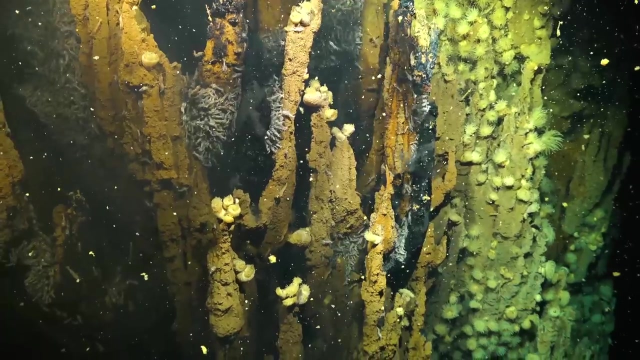 that facilitated the dawn of life on Earth. Unlocking their secrets might provide an avenue to understanding the possibility of life on other planets or moons, Water worlds that may play host to vents of their own. Vents like these form as the rifting of tectonic plates. 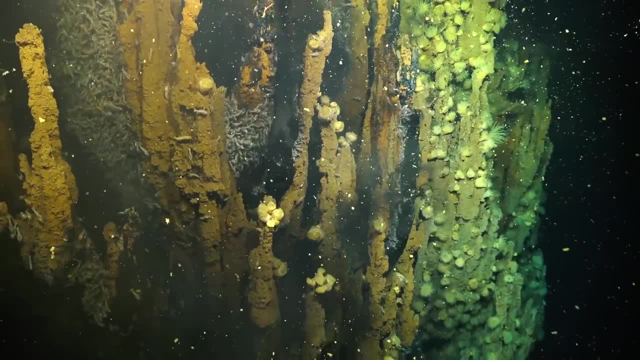 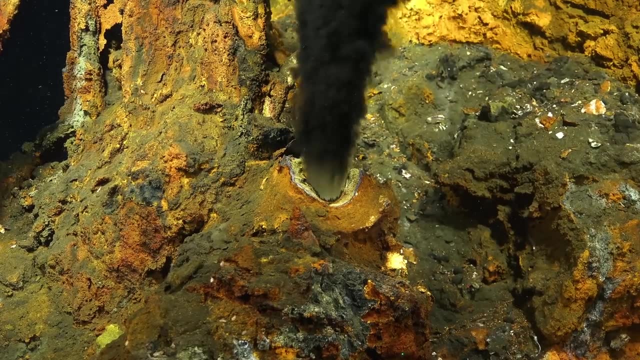 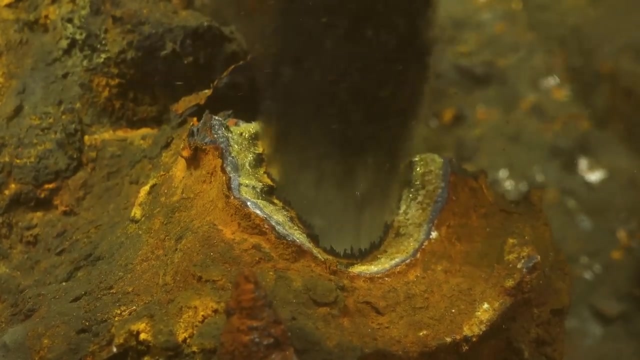 allows hot magma from deep within the Earth to rise closer to the seabed, where seawater becomes superheated and takes up minerals from surrounding rocks. This mineral-rich fluid jets back into the ocean at extremely high velocities and temperatures exceeding 400 degrees Celsius. 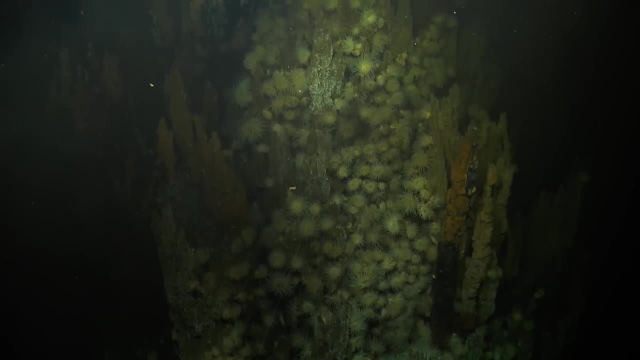 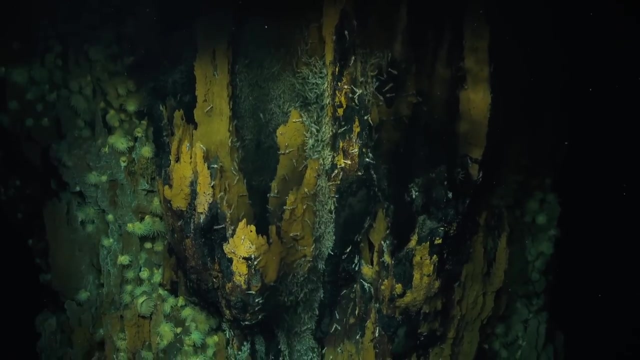 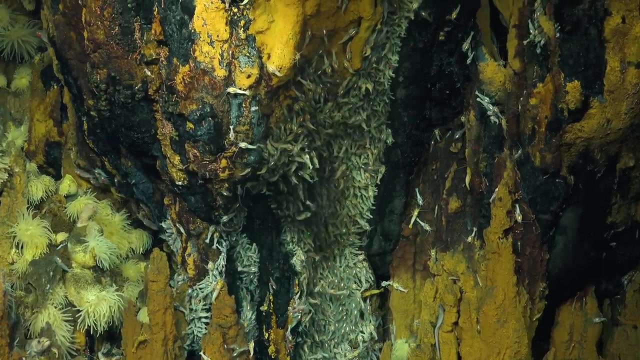 mixing with cold seawater and precipitating dissolved minerals out in smoke-like billows. The chemicals here incite a process that mirrors photosynthesis, where chemical energy, instead of energy from the sun, enables primary production via chemosynthesis. Because of this, life doesn't just survive here. 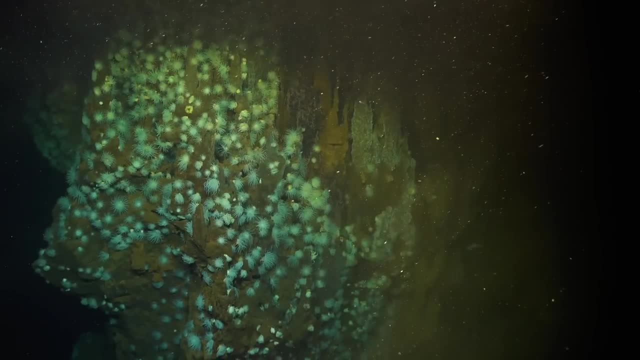 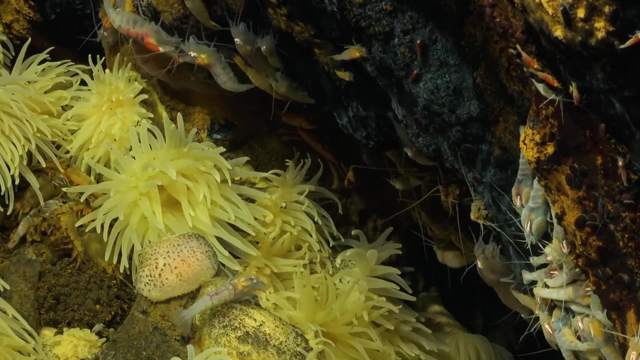 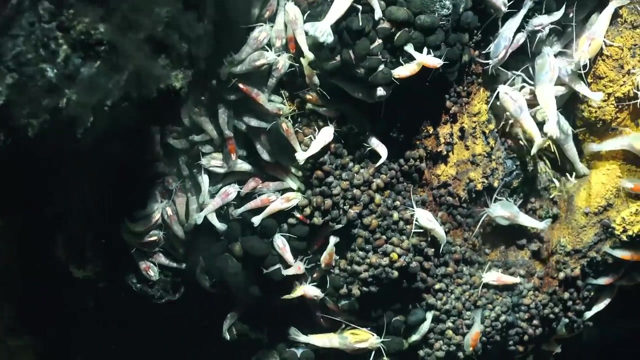 It thrives In the depths. vents stand as otherworldly oases, offering a glimpse of the resilience and adaptability of life on Earth to even the most extreme environments. In all, three entirely new vent fields were discovered during Falcor II's inaugural expedition. 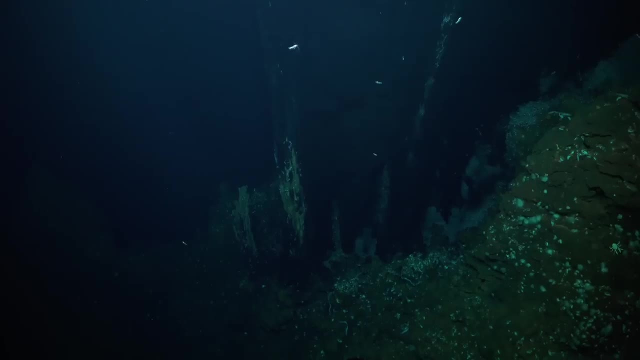 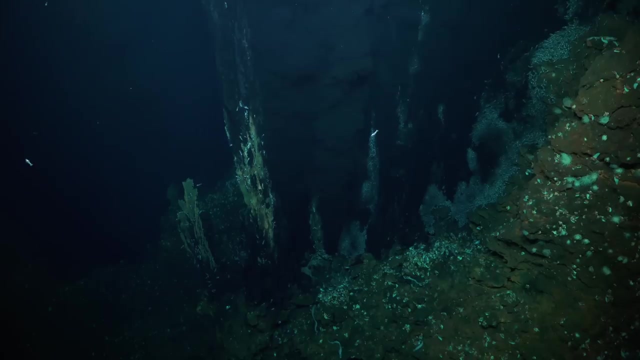 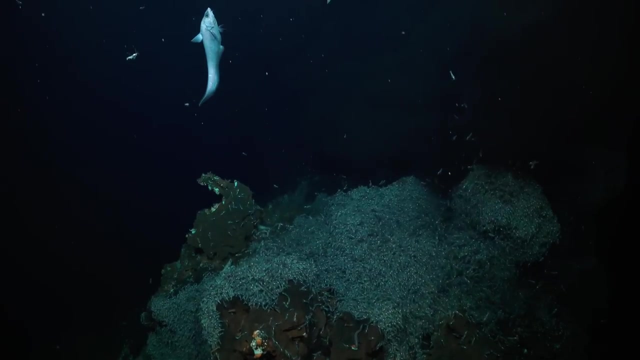 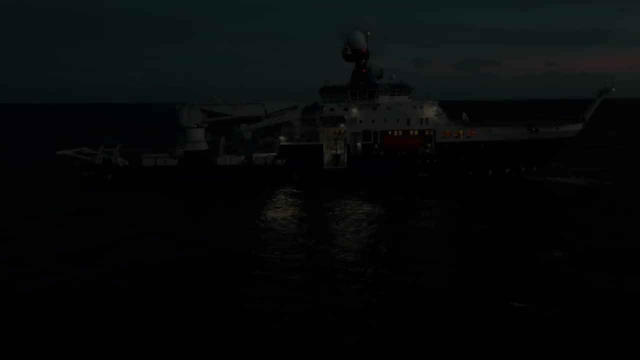 These may not be the type of vents they sought, but when it comes to exploring a place as mystifying as the deep ocean, you might not always find what you're looking for, But you're bound to discover something just as remarkable. Hydrothermal vents have been known to science since 1977,. 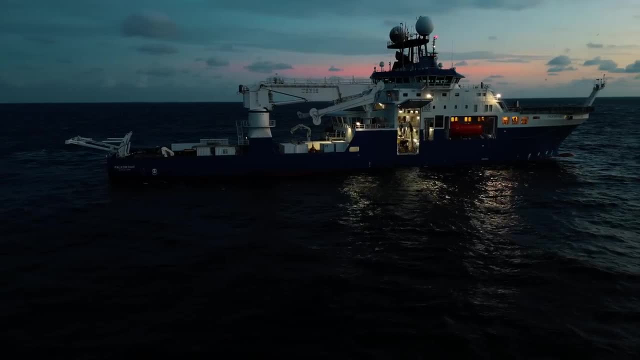 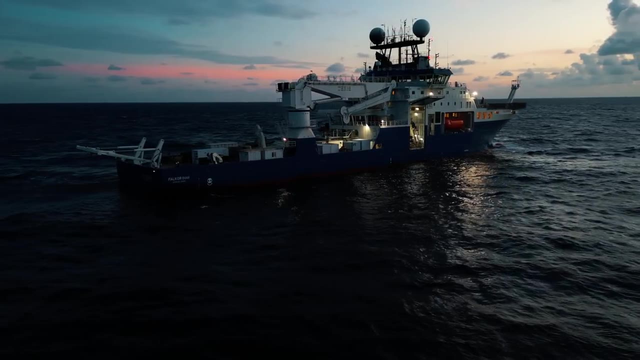 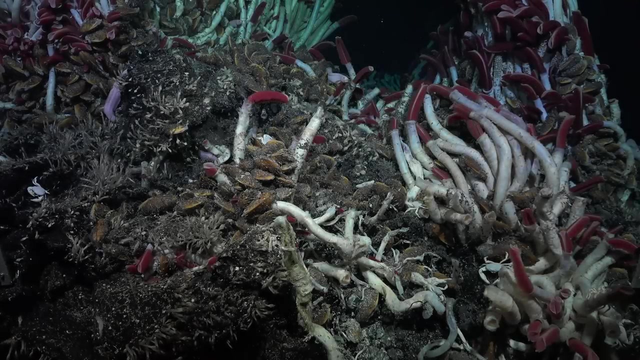 but a number of mysteries endure surrounding the origins of their communities Over geological timescales. they are ephemeral Bound to the destructive influence of eruptions and earthquakes. So how can it be that, no matter where they form, a diverse biological hotspot almost always follows? 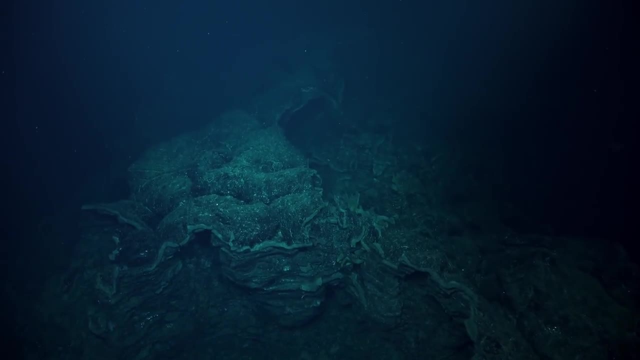 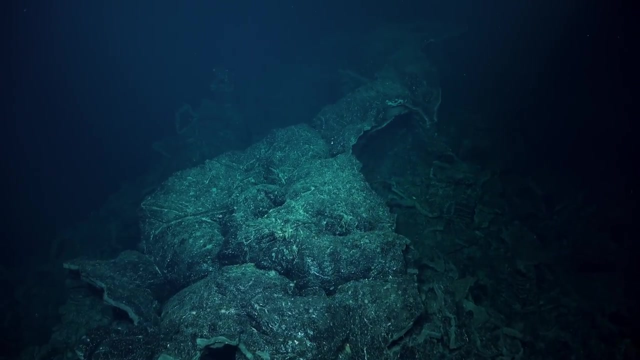 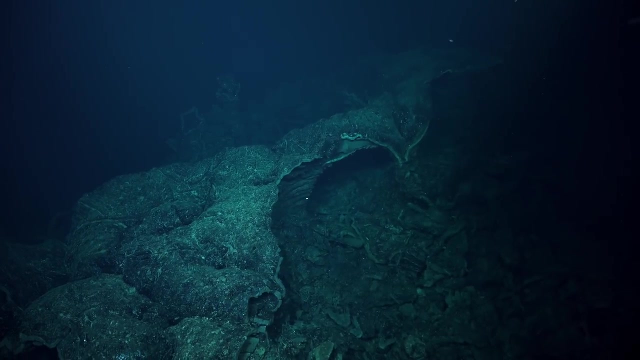 Dr Monika Bright of the University of Vienna hypothesized that the answer lies beneath the sea floor, where the existence of a proposed subsurface ecosystem, hidden from view, might allow animal larvae to pass between vent fields and colonize these puzzling worlds. 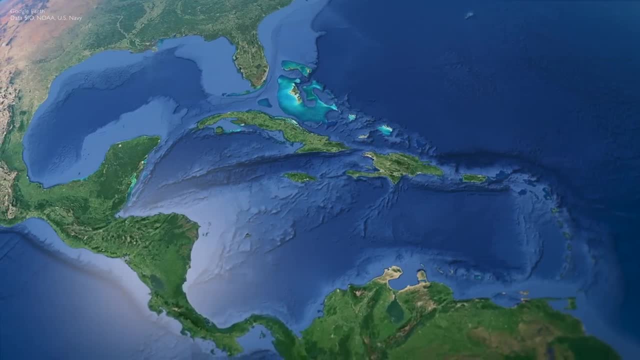 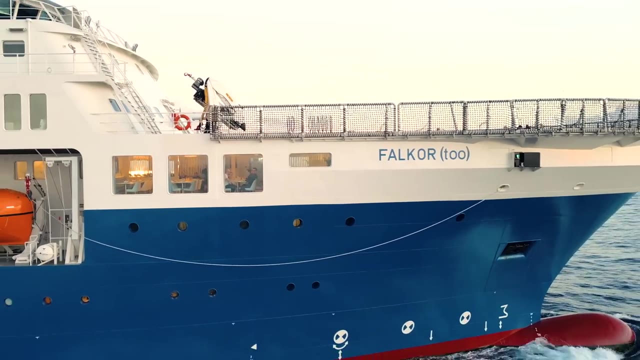 We journey now from the mid-Atlantic ridge to the East Pacific rise where, in August, Monika and her team set out on Falcor II to test this hypothesis and seek out the proposed underworld of hydrothermal vents, should one exist at all. 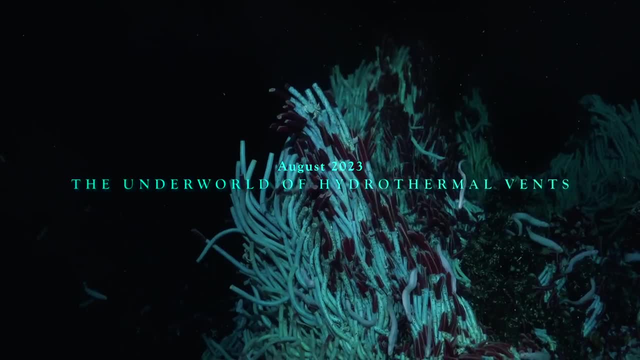 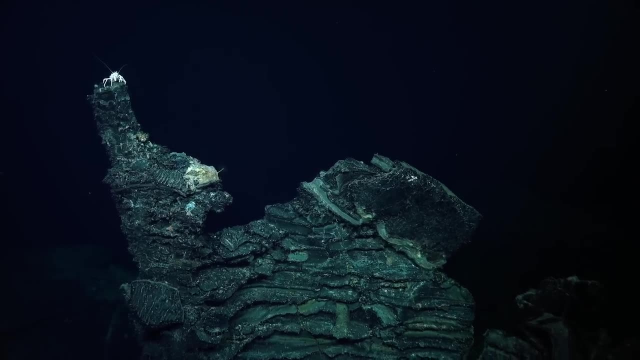 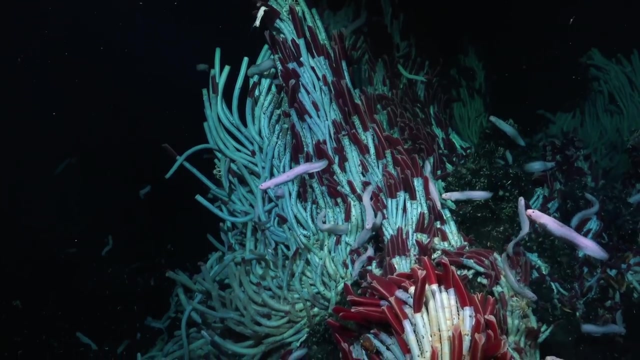 This is the Tikka vent site, one of the most studied in the world. In 2005, it was destroyed by a volcanic eruption, But in the years since, follow-up expeditions began to investigate the recovery and primary succession of animal communities at Tikka. 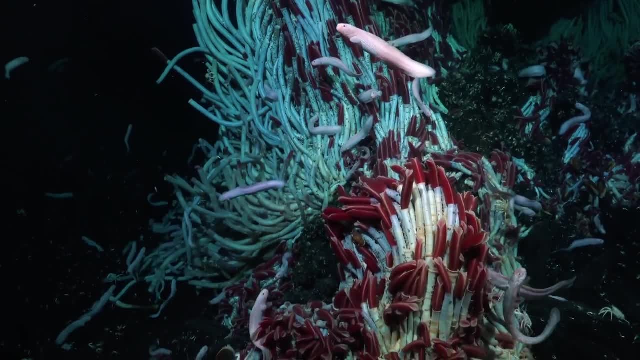 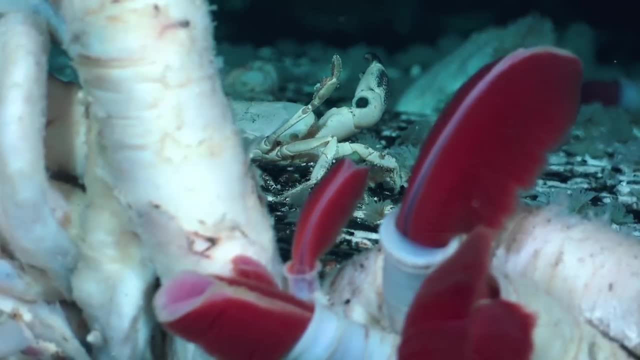 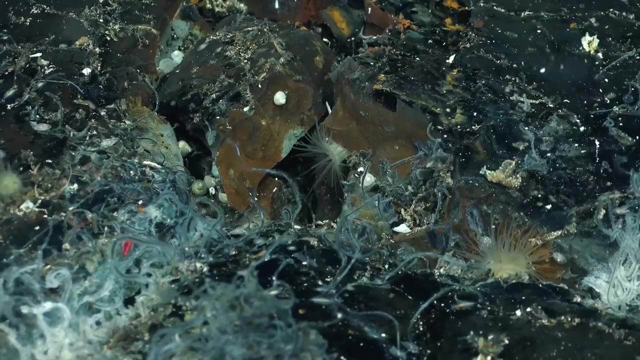 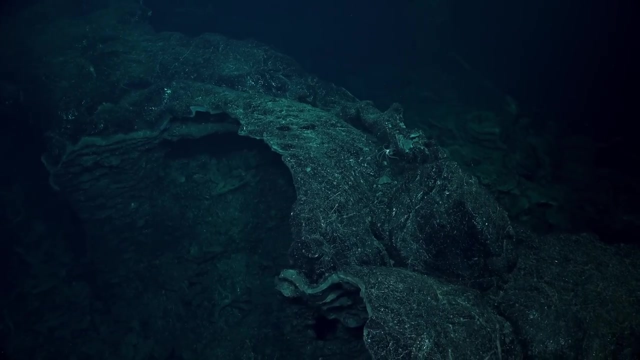 following such a large-scale ecosystem reset, Recovery had been quick. Tube worms, mussels, stalked barnacles and more had already recolonized and established themselves among the mineral spires. Now the team leading the 2023 mission with Schmidt Ocean Institute, 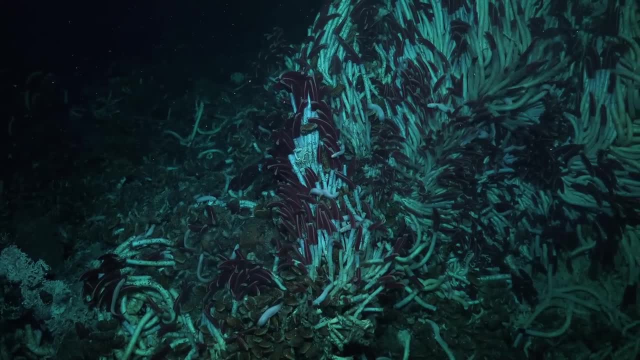 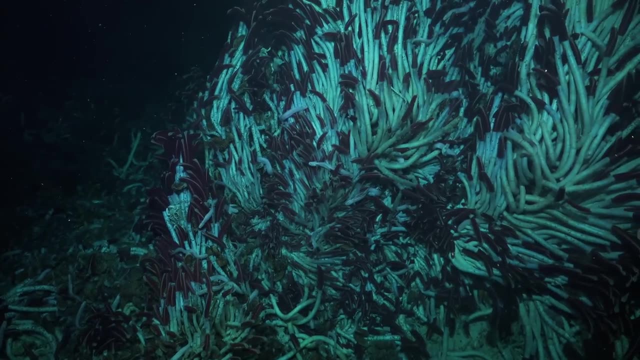 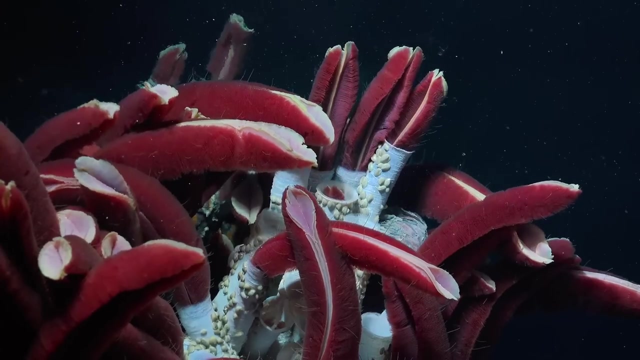 hoped to find out how life had returned after the devastation. Vents at Tikka are home to a species that embodies all that is weird and wonderful about these alien habitats: Giant tube worms of the genus Riftia. They stand up to three meters tall. 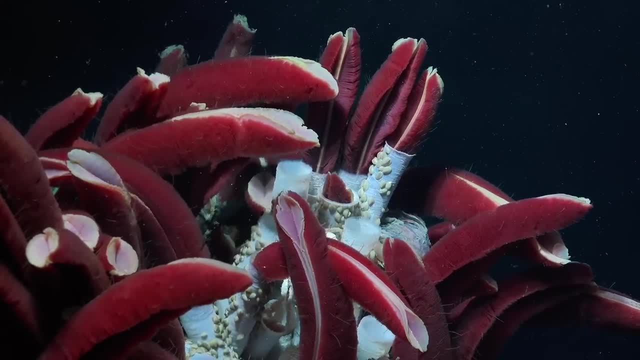 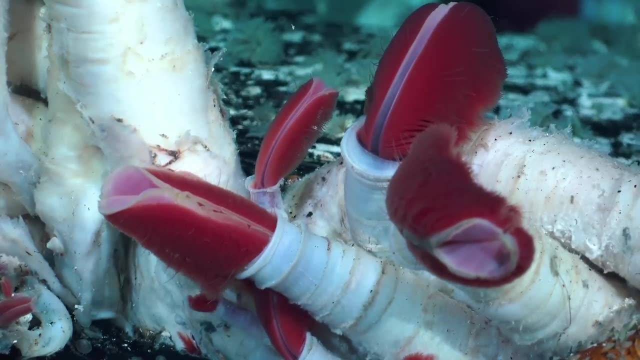 with a bright red branchial plume that channels chemicals from the vent fluid to colonies of bacteria that inhabit their tube or trophosome. The bacteria in turn convert these chemicals into food that sustains the worms. A perfect symbiotic partnership. 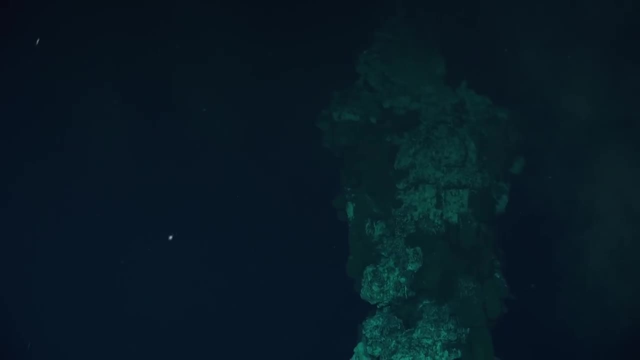 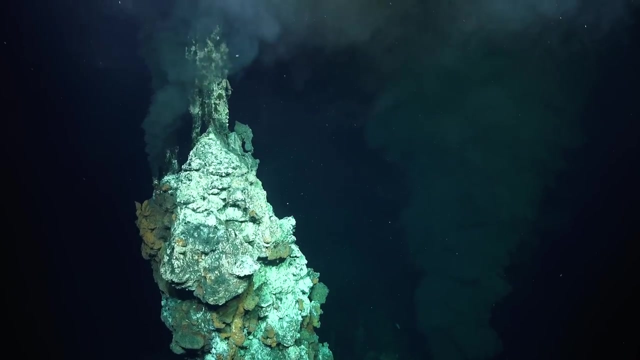 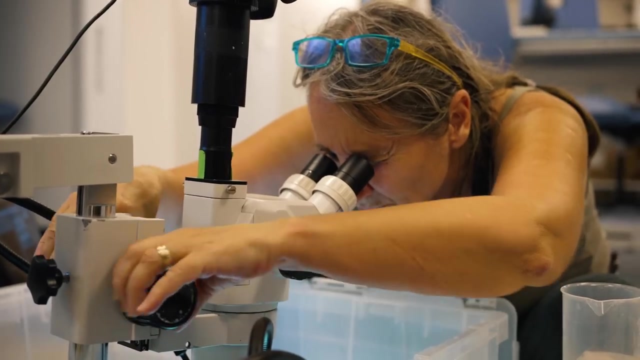 While larvae of mussels and barnacles had been found in the seawater around the vents, the larvae of Riftia had never been sampled, pointing to a different method of dispersal so far undiscovered. Over the course of the expedition, Monica and her team dug deep to uncover the mystery of the subsea floor around Tikka. 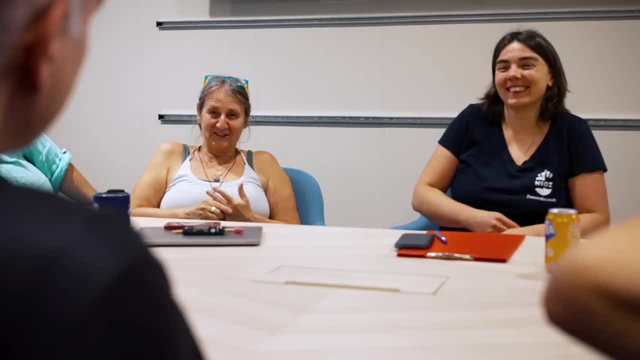 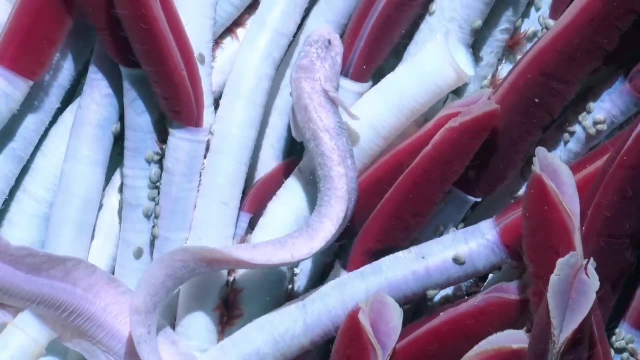 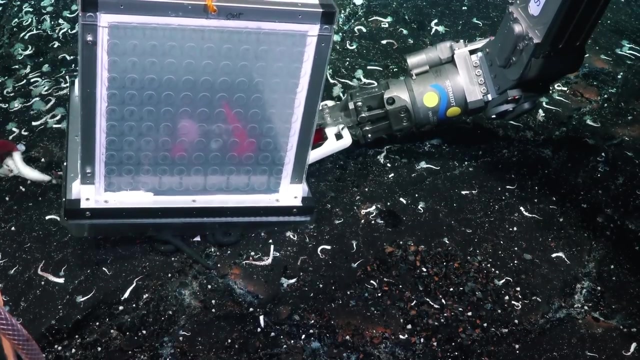 and what they found redefined our understanding of life and succession at deep-sea hotspots. We do not really fully understand how the animals that live there actually find this place and can come to this place. We look for the first time into the subsurface life. 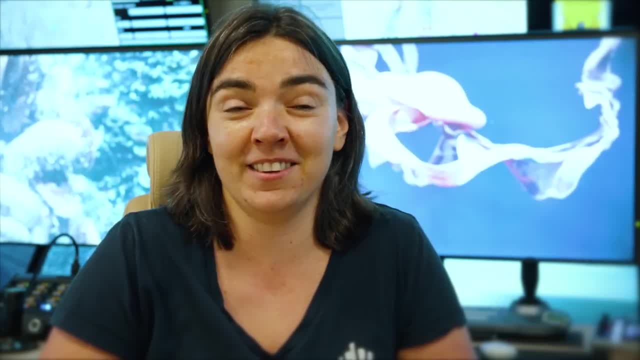 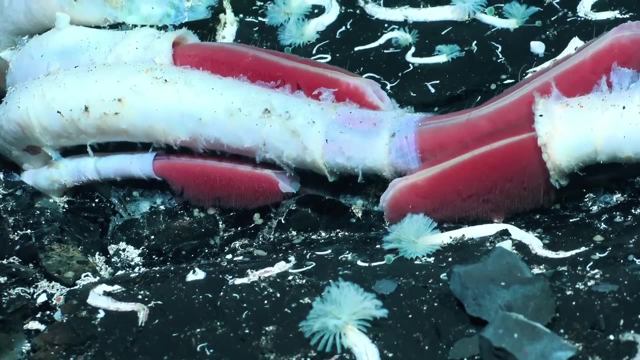 Animals are able to live below height of male vents and this is, I think, mind-blowing. Now we know that, for example, tube worms- they can colonize vents by traveling through the subsurface. This is the first finding. 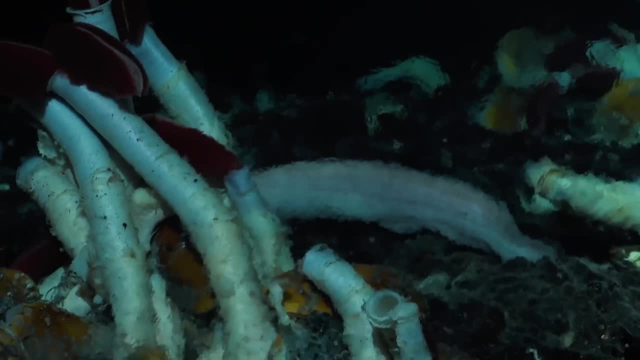 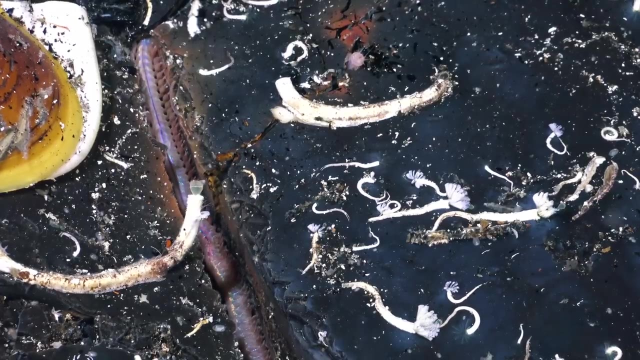 We know that these tube worms, they can live in this cave system. That's the second finding. The third finding is that also the mobile fauna, mobile vent fauna, can live in these subsurface areas. Such a method of dispersal is completely new to science. 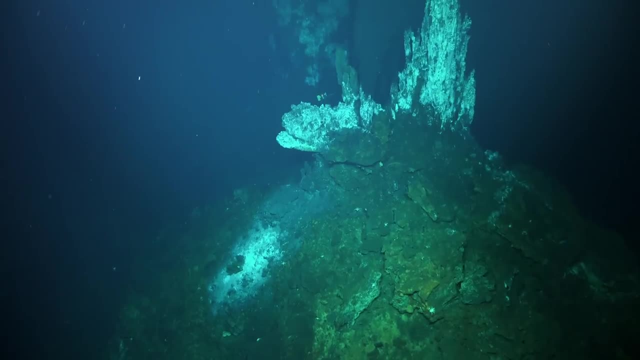 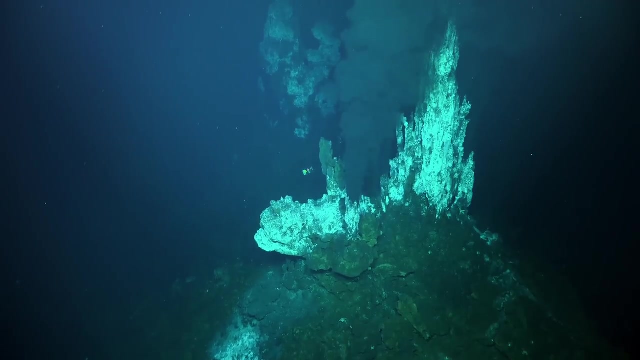 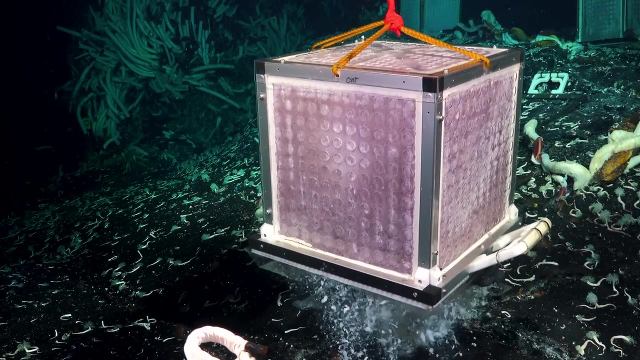 and it challenges the idea that most vent larvae rely on open-ocean currents to disperse their young. But what the team discovered went above and beyond what had been hoped for. The beauty of all of this is also that the experiment itself was not even working so well. 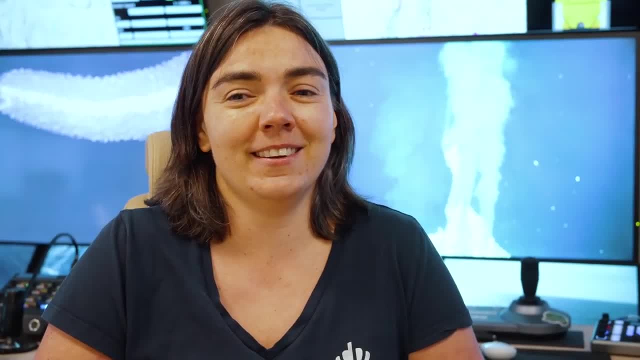 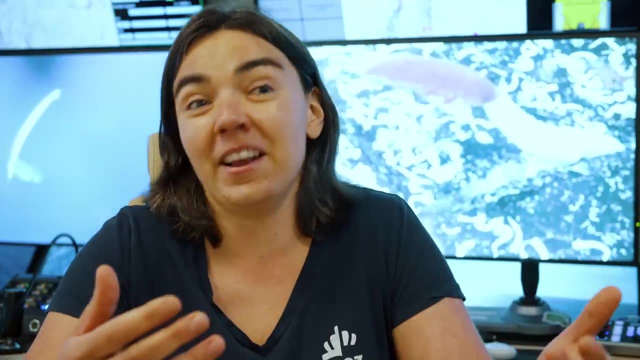 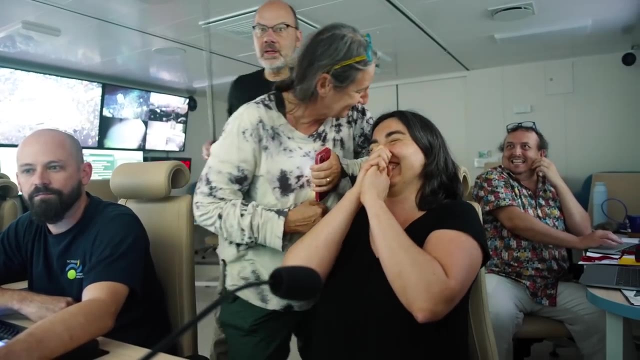 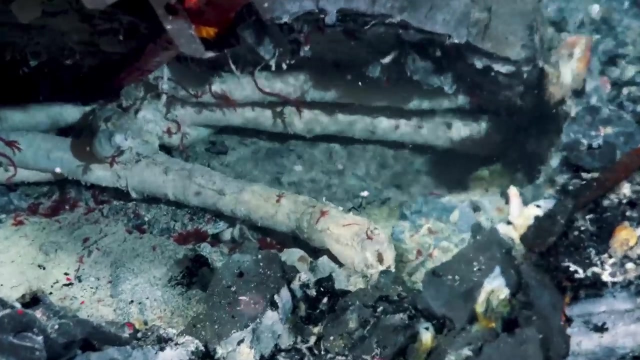 We kind of needed to be creative and, you know, apply basically a new method. Flipping around the rocks opened our view into the underworld of height, of male vents. What we found was that we found even animals living below the surface. This expedition marked the discovery of a dynamic habitat entirely new to science. 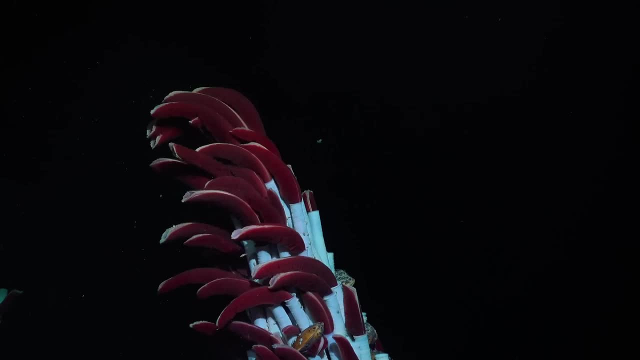 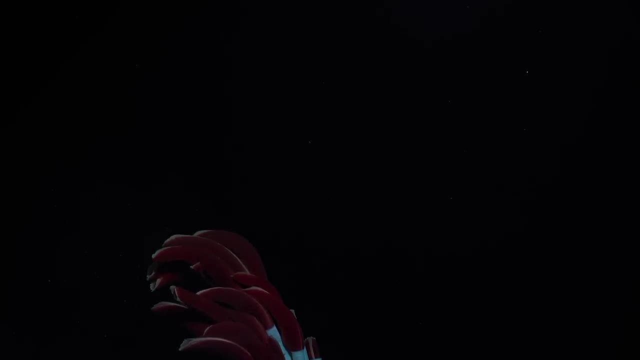 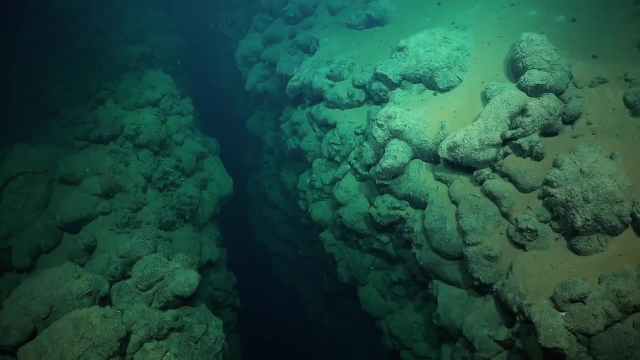 existing in delicate unison with the vents above. If there's one thing the deep ocean has taught us in the relatively short time since the scientific community first plumbed its depths for life, it's that frontiers of biodiversity exist even in the places you'd least expect. 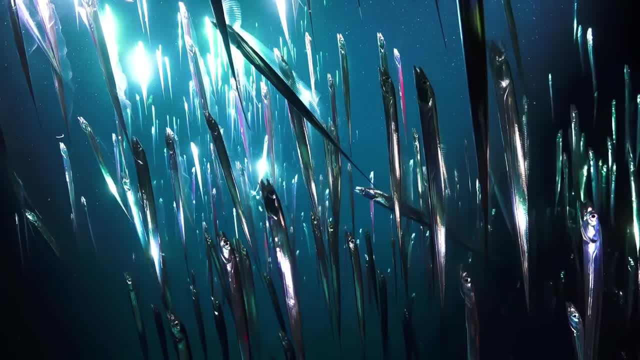 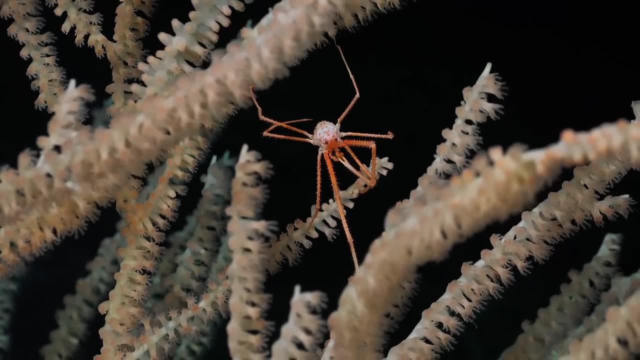 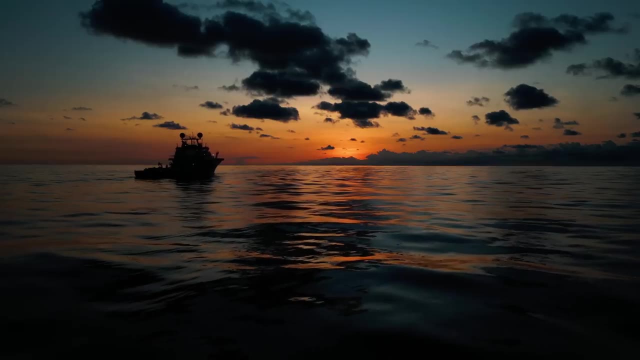 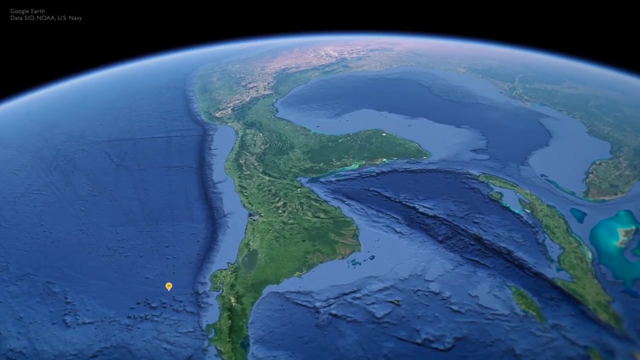 Our oceans are home to countless species Across divergent worlds, And yet much of their biodiversity is unknown. This knowledge gap stands in the way of fully comprehending the awesome power of life on Earth or the extent of human impact. In June, FALCOR2 arrived in Costa Rica to investigate the biodiversity of an unprotected seamount. 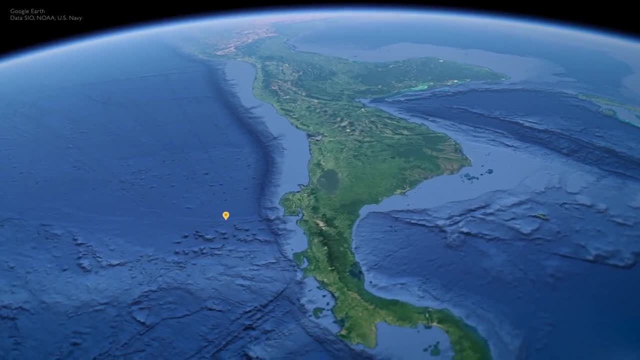 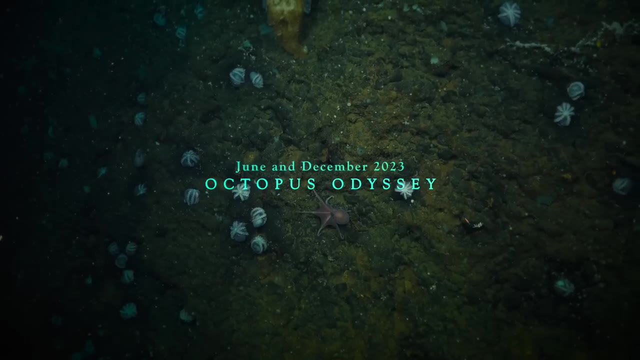 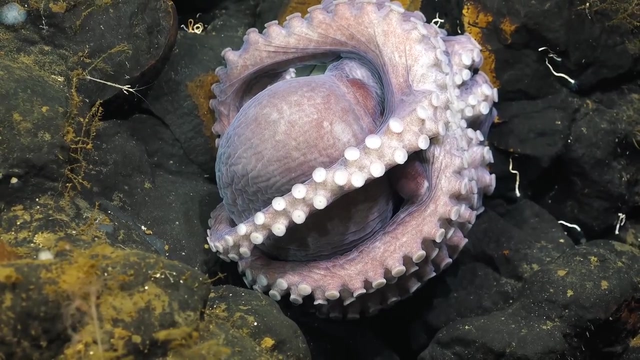 where, in 2013,, an unusual discovery had been made: An estimated 100 female octopuses gathered at a small outcrop to brood their eggs. It became known as an octopus garden and hinted at the potentially rare and life-supporting role of seamounts such as this. 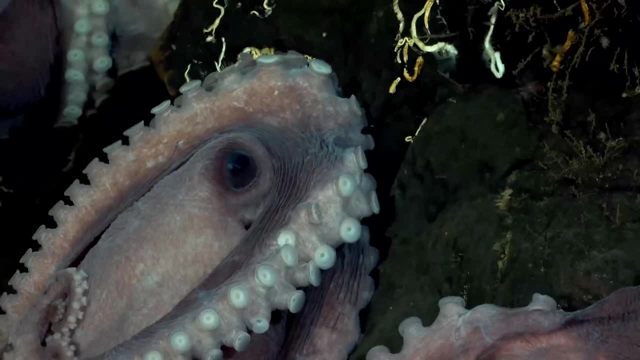 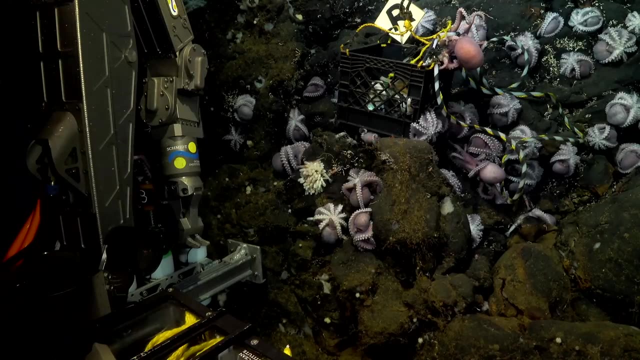 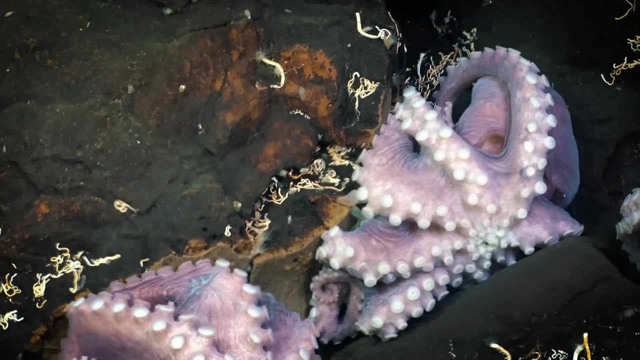 where low-temperature venting might provide the perfect conditions for eggs to develop, But so far no viable embryos had been found, leading scientists to wonder whether the site truly supported octopus development at all. If this phenomenon could be verified, it would make this nursery a feature worth protecting. 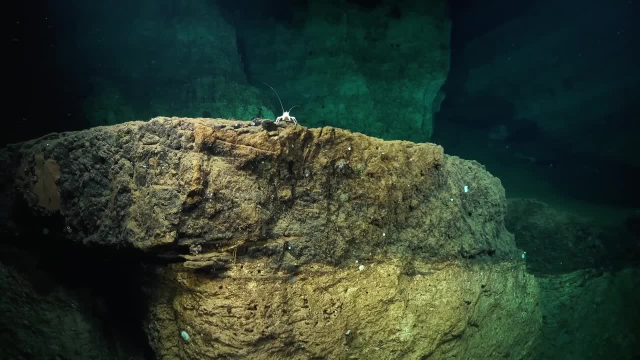 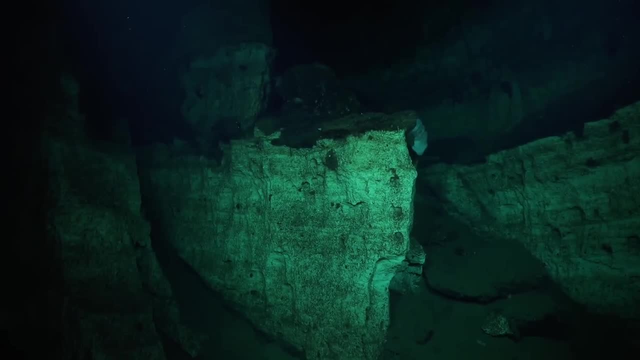 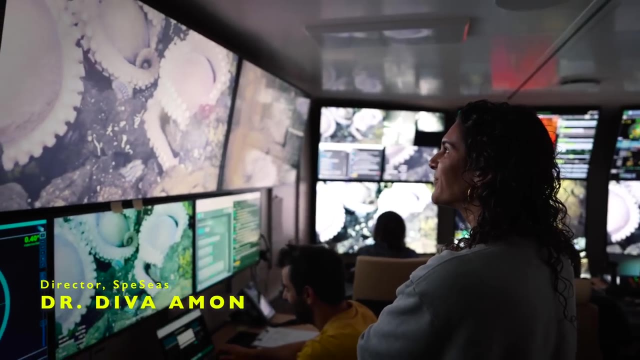 Costa Rica is about 90% deep sea and most of it has never been explored, So this expedition has been really critical on local levels, on regional levels and on global levels. Costa Rica is actually going to be hosting, in 2025, the United Nations Ocean Conference. 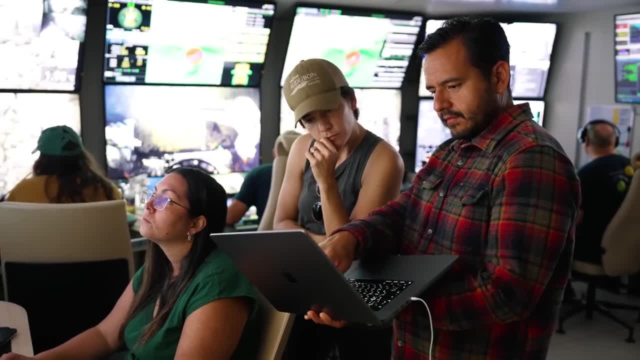 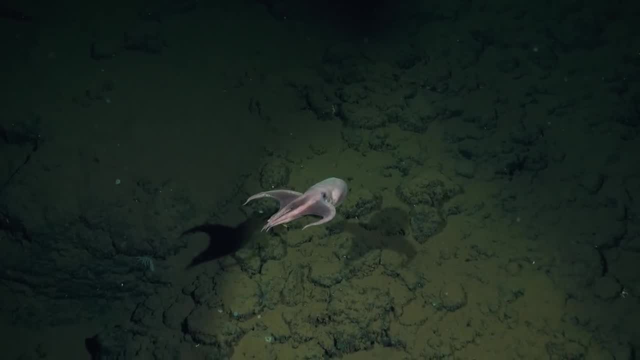 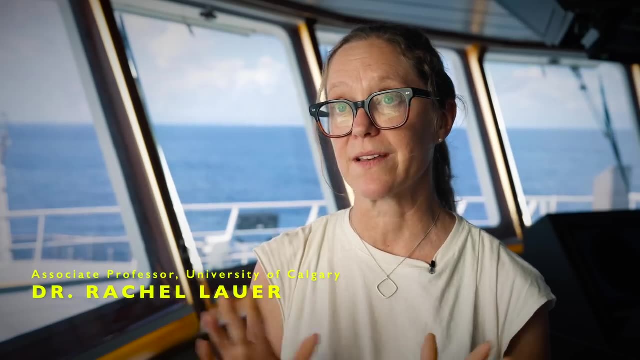 With Costa Rica in that leadership role. this cruise provides a brilliant opportunity to really allow us to take the science to decision makers at that forum and really put the deep sea center stage. And for us this cruise has been just an incredible success from day one. 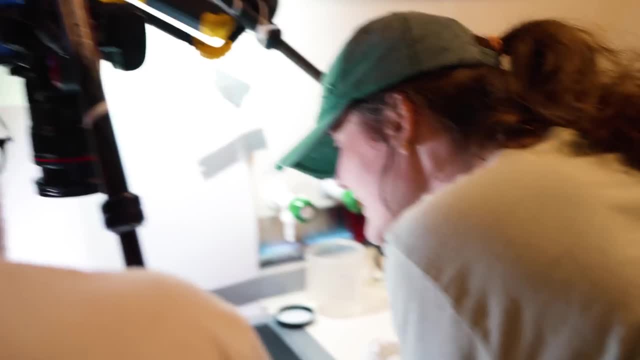 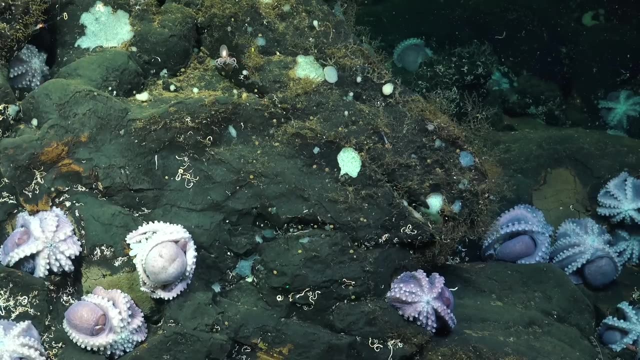 Verified a few of our hypotheses and then a few more within days after that, which I can't say. how rare that is in deep sea exploration. The eggs were viable, which has just been mind-blowing. We found things we weren't expecting. 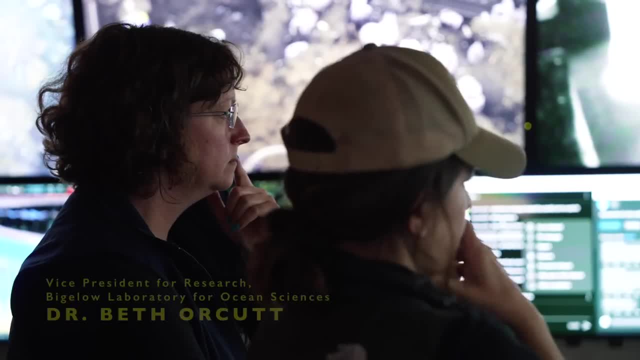 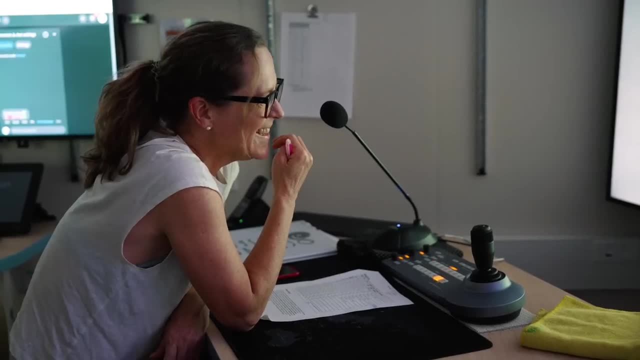 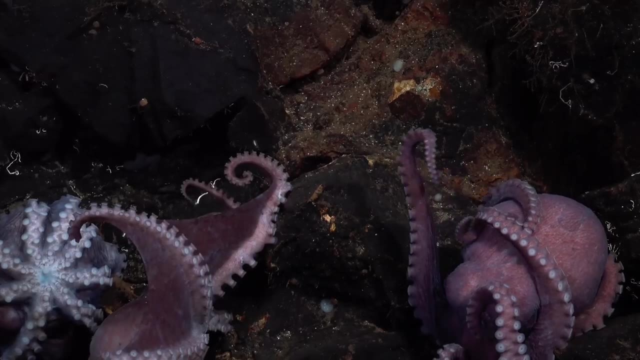 Like a skate nursery. We discovered a new low-temperature hydrothermal vent. It also has octopus brooding their eggs there. I was so excited. Beth was like Rachel: go outside and scream. I was bouncing off the walls. Brooding in this way is a labor of love for the females. 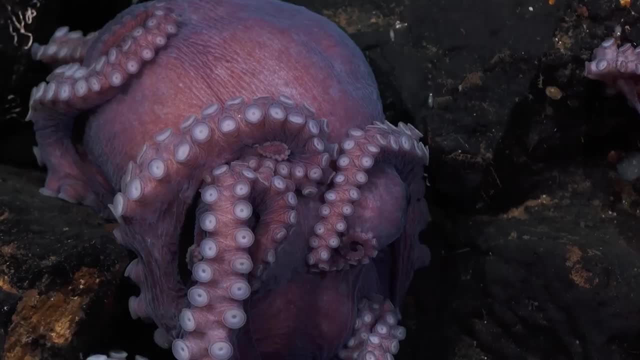 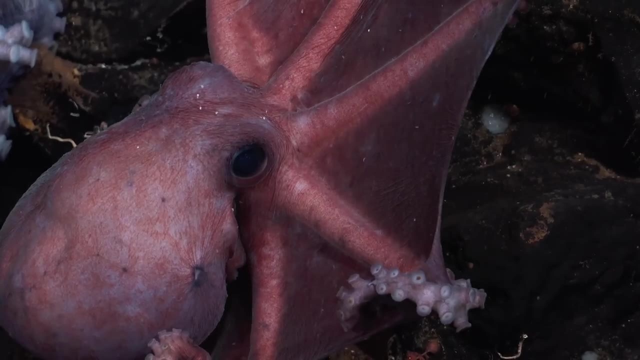 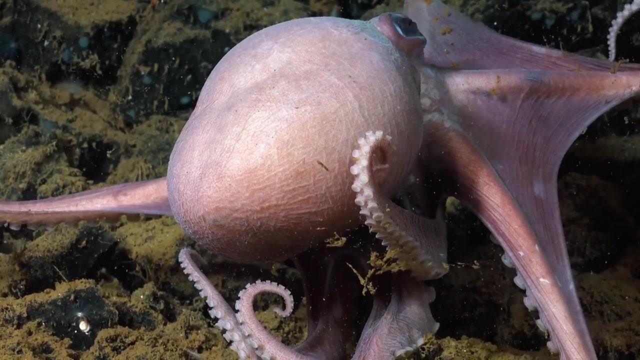 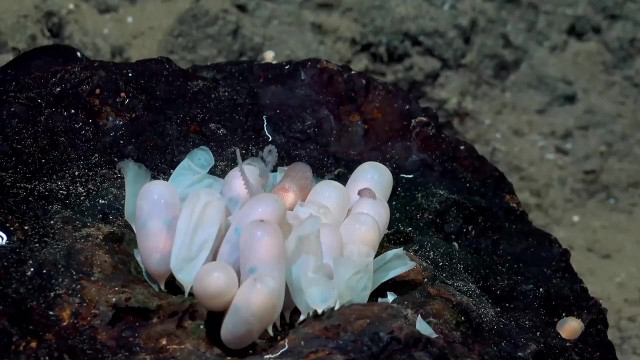 It can take up to five years, And during this time they don't seem to feed much, If at all. It's thought to be their last mission, Guarding their eggs to the very end of their life, But it's not in vain. 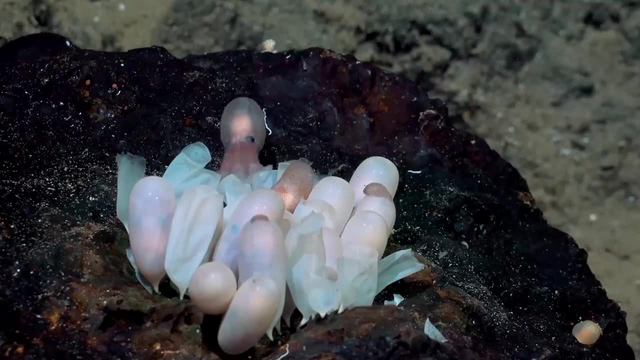 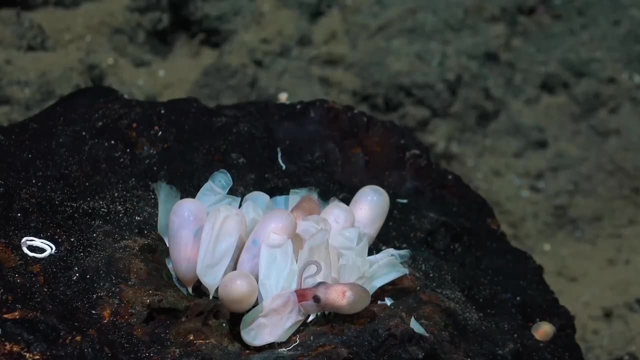 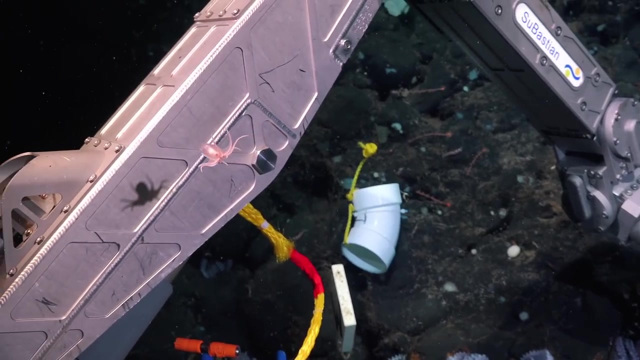 They're racking their brains. Witnessing babies hatching in real time confirmed to the science teams that the dorado outcrop is indeed an active nursery. We just hatched And we're looking at a brand new baby octopus- Amazing. 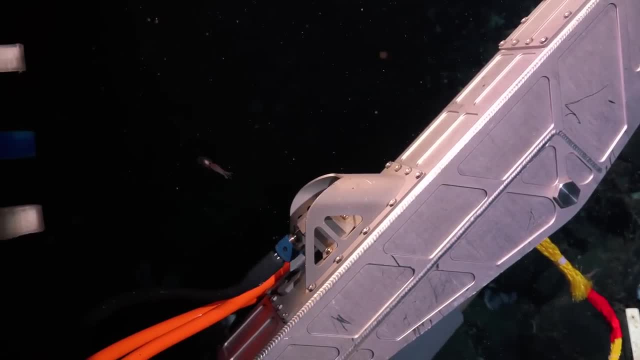 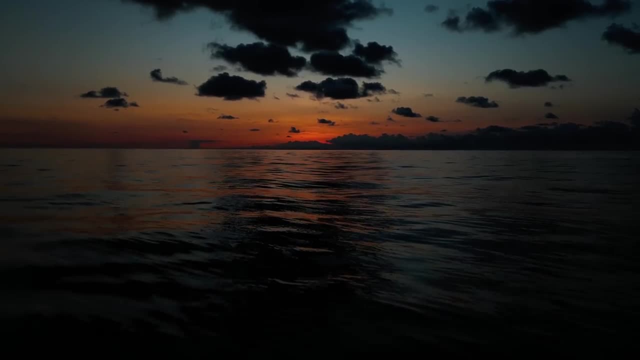 Happy birthday. Happy birthday, Oh look, we got an octopus shadow. This might be the only time in that octopods life that it gets a shadow. Their findings at the site unveiled a deeper understanding of the level of activity, understanding of the life history of these octopuses and the ecological 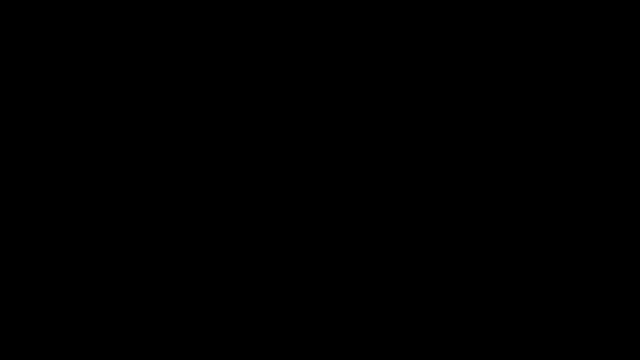 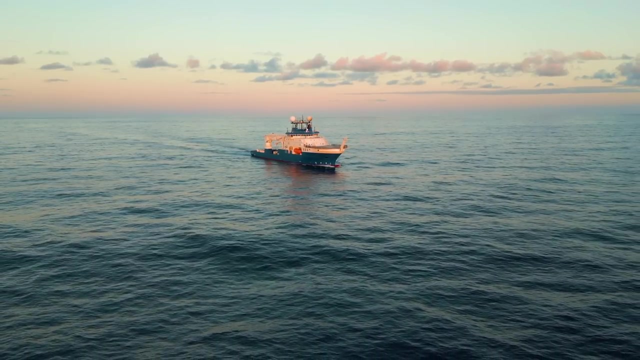 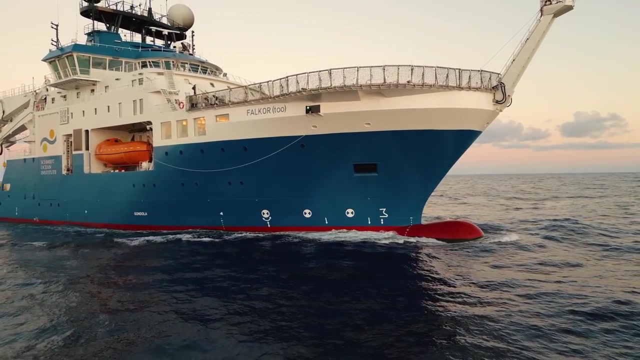 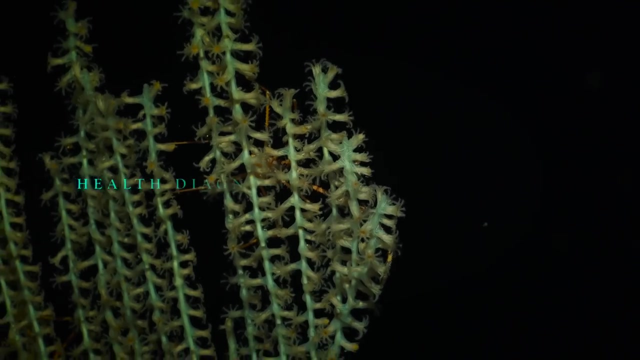 significance of seamounts. Technological innovation can unlock new ways of understanding the human effect. Since it was established, Schmidt Ocean Institute has offered up its facilities and resources to the international scientific community at no cost to test new technologies and conduct groundbreaking research. In April, scientists aboard Falkor 2 set out to 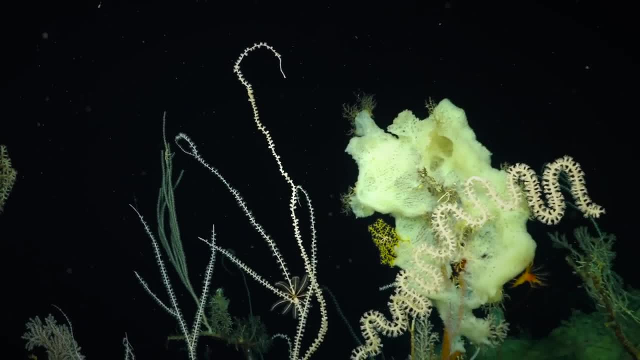 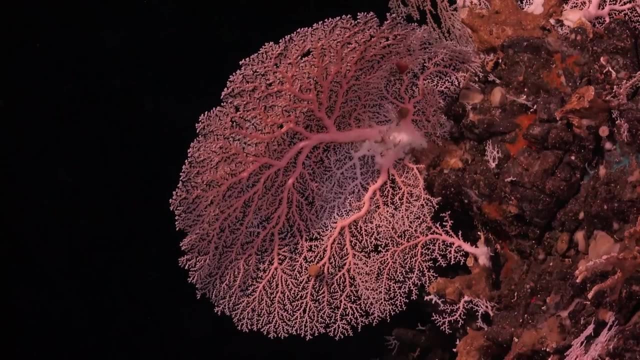 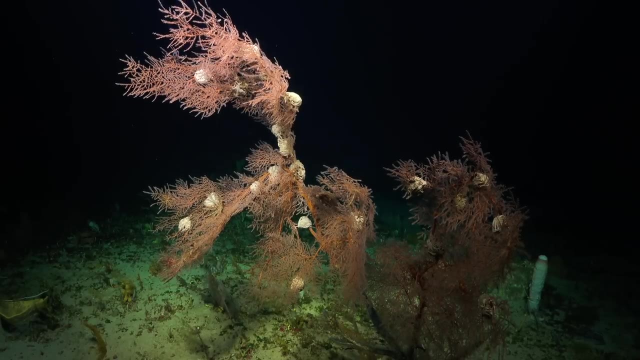 study the impact of climate change on deep-sea corals using a new technology called Solaris. These reefs are cities of life in the depths, hosting biodiversity akin to that which flourishes near the surface, though hidden away in the ocean's twilight zone. 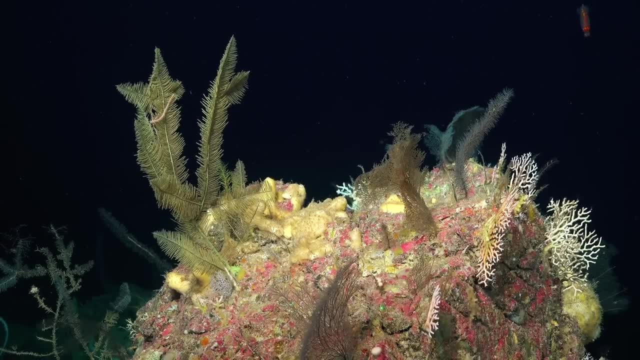 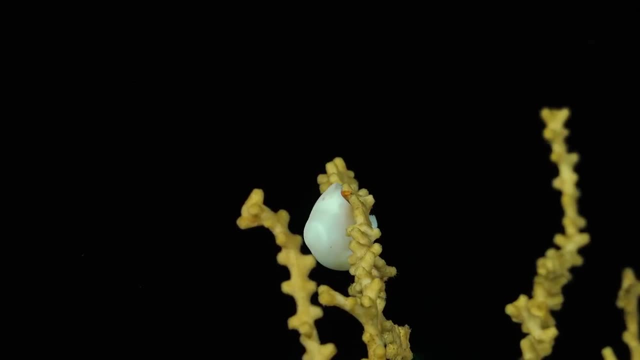 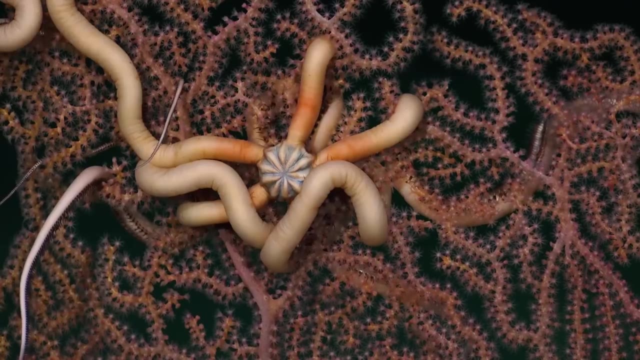 In these ethereal secret gardens where sunlight dwindles to a mere glimmer, an array of corals and sponges build a complex home where other animals can shelter and find food. Squat lobsters cling to the coiling corals alongside brittle stars, making the 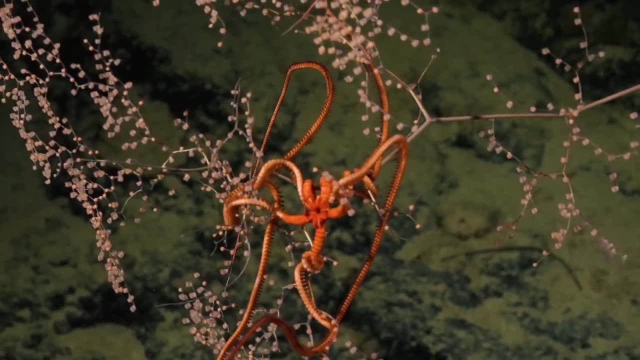 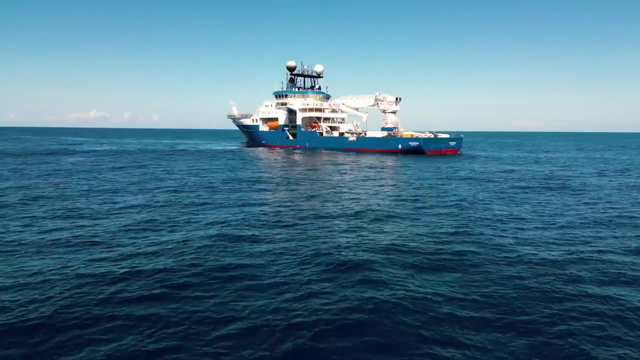 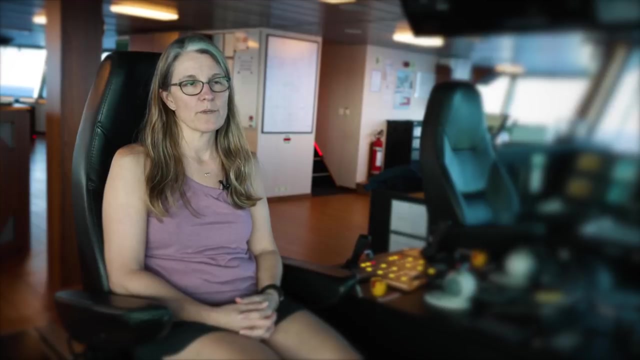 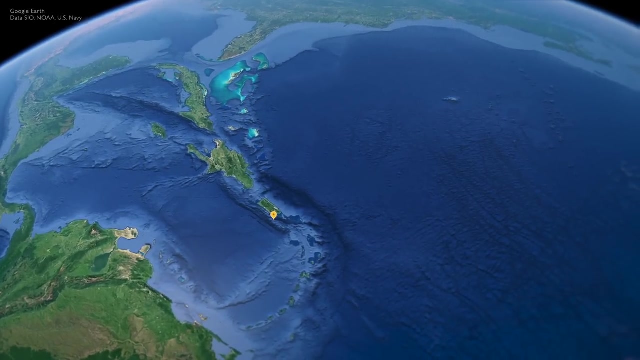 most of these branching structures to reach into the flow of current, where faster-moving waters bring a feast of plankton and organic debris towards them. So we are off of the coast of Puerto Rico right now and we're gonna be exploring mesophotic and deep-sea corals along the west and southwest portion of Puerto Rico. 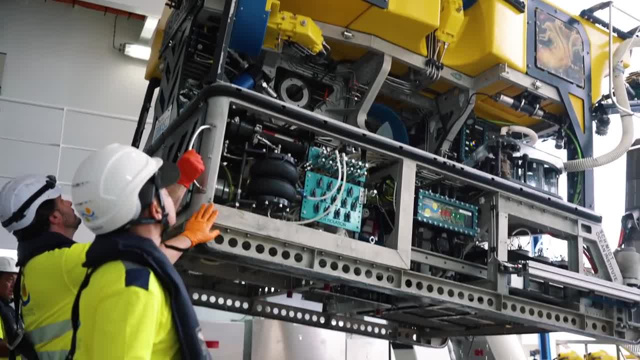 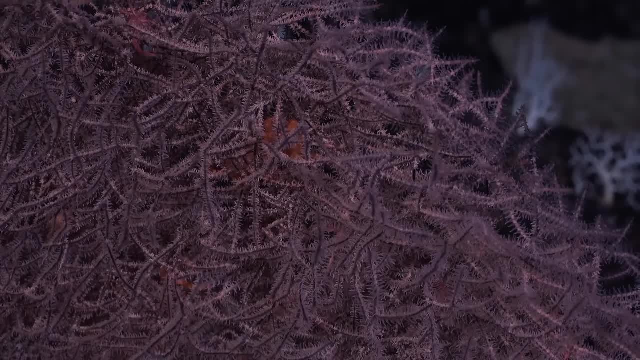 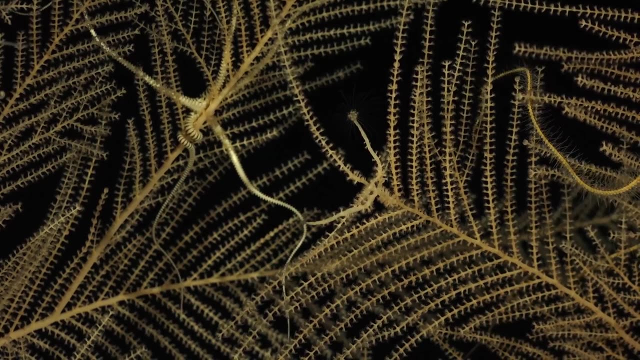 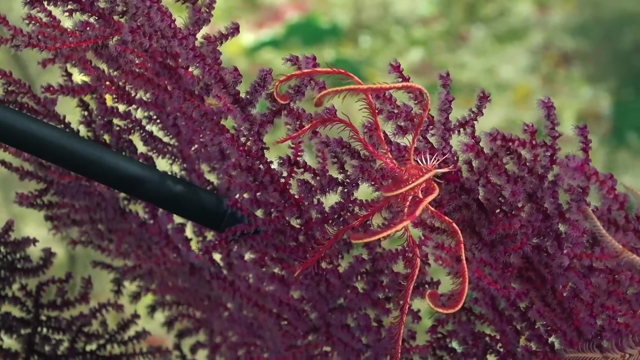 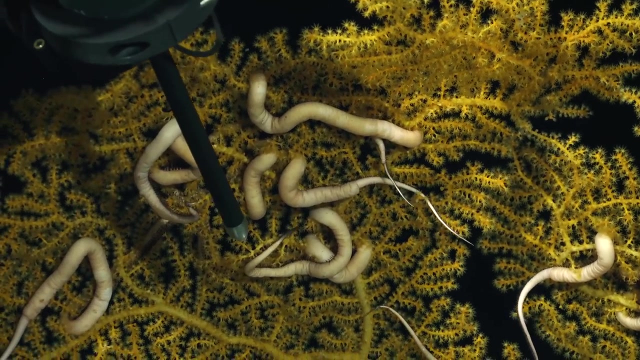 My group studies a group of chemicals called the reactive oxygen species. We call them ROS or raw objectives, And ROS are oxygen intermediates, so you can think of them as a really reactive forme of oxygen. What we have seen in shallow reef environments is that coral species that tend to be more resilient towards thermal stress- empathogen infection- have much higher concentrations of superoxide. 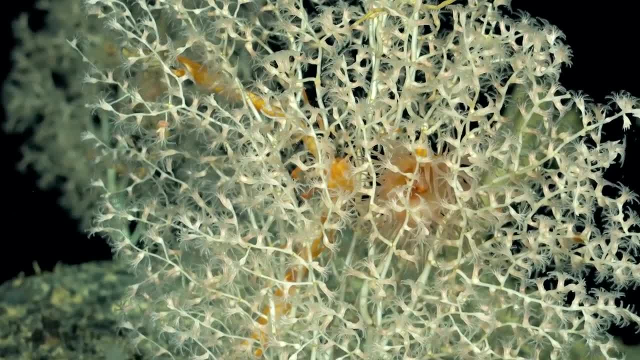 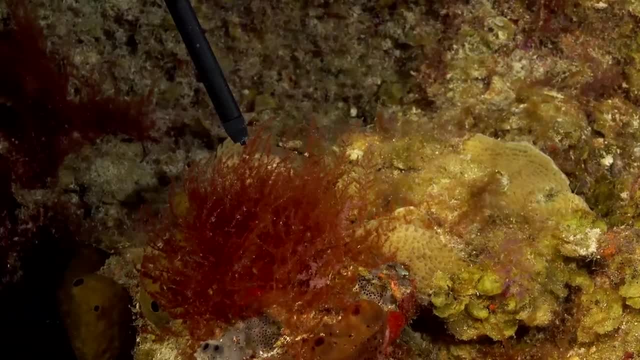 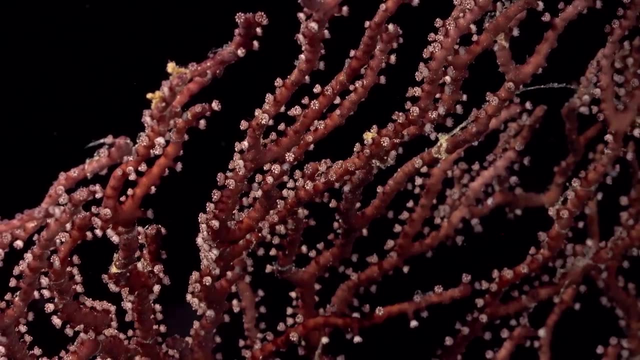 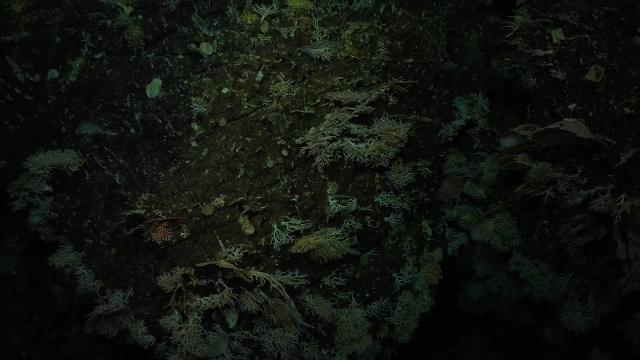 And so we believe11. So we believe that this is serving kind of like an armor. If these chemicals are in fact protecting corals, then we may be able to help corals armor themselves from stress by better understanding the controls that promote their formation. 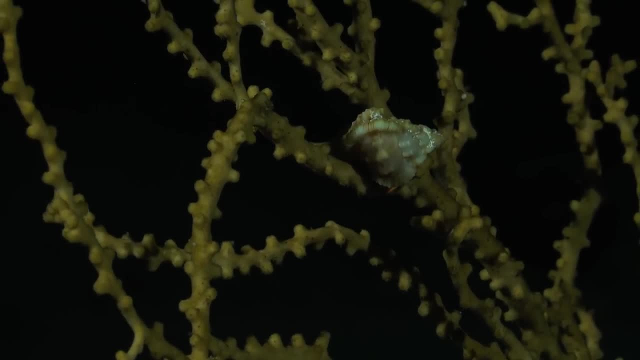 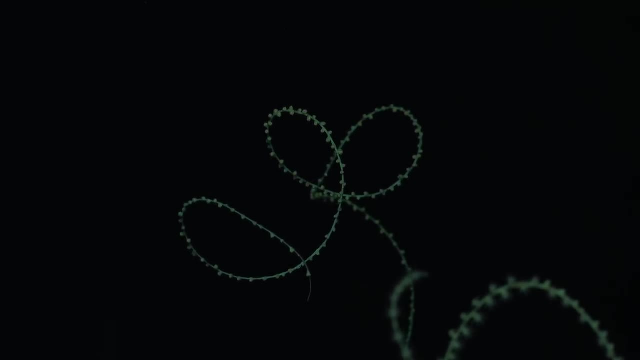 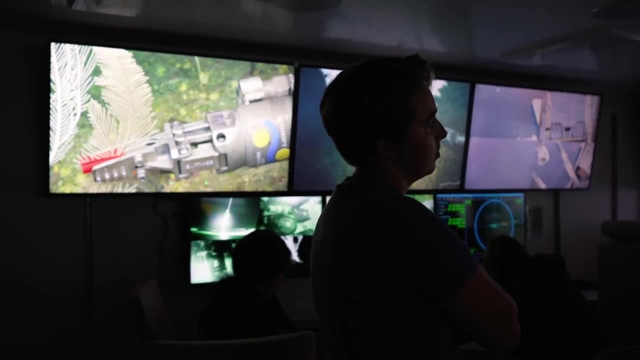 We have very few measurements of these chemicals within the ocean because they have a really short lifetime, So we don't really know why these corals are making them. when do they make these reactive oxygen species? at what concentrations is it toxic? at what concentrations is it beneficial? 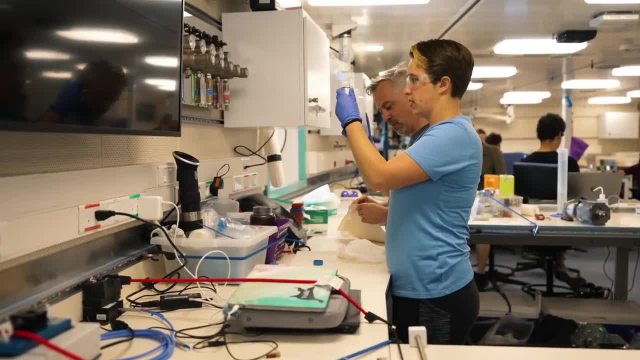 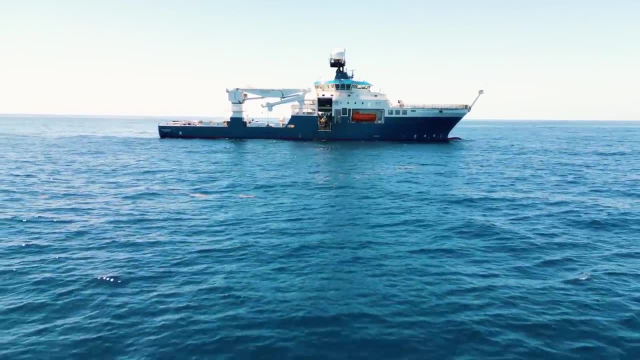 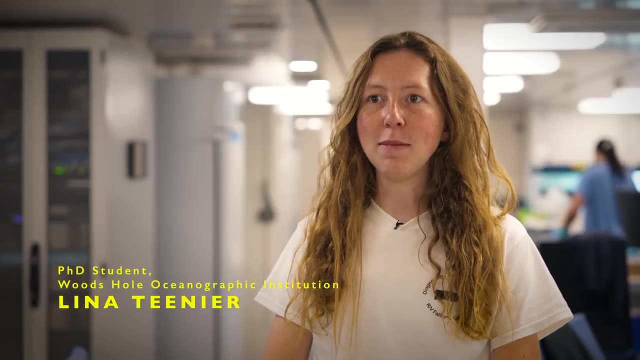 And we have this wonderful team of chemists and biologists and engineers all working together to try to understand this process that we know nothing about within the ocean. So, with the funding of Schmidt Marine Technology Partners, Colleen Hansel's lab has been developing the first kind of series of in situ reactive oxygen species sensors. 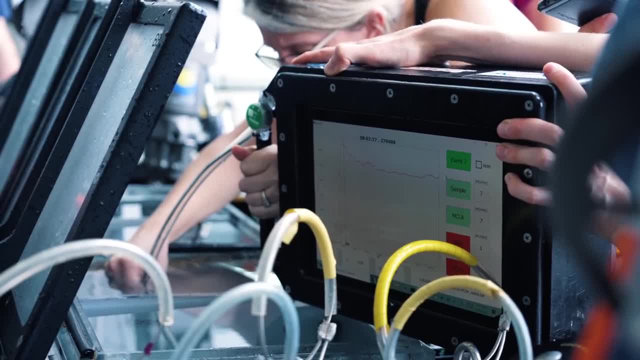 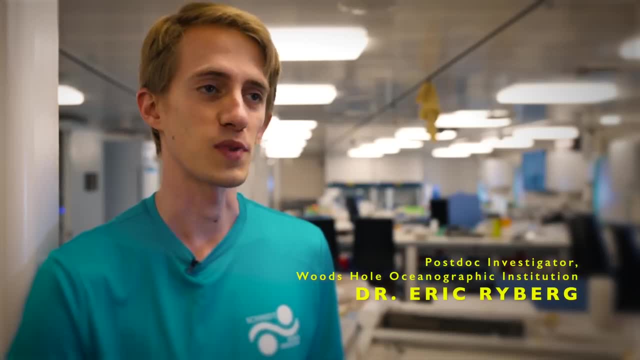 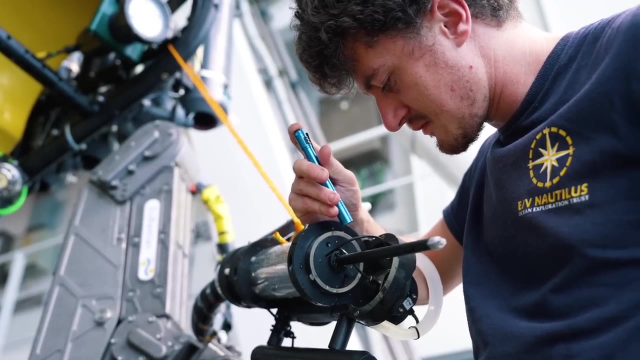 that can be used in aqueous environments. The way that we're monitoring the health of these corals is by using a sensor called DISCO. It measures these reactive compounds that these corals produce. In order to reach those deep sea corals, we need to develop a whole different type of 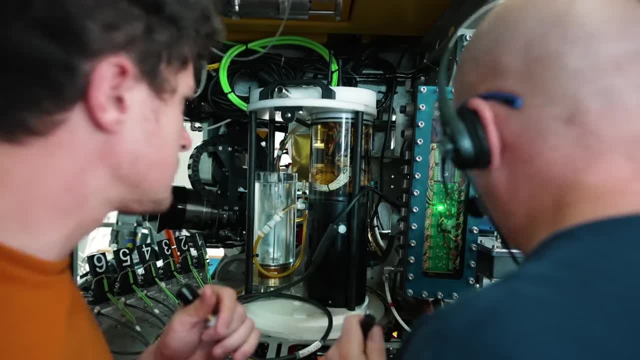 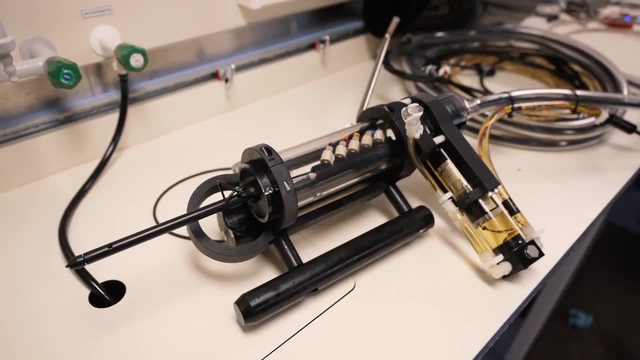 instrument. We couldn't take DISCO down to the bottom of the ocean. It doesn't have the right pressure. It doesn't have the right pressure tolerance. It doesn't have the right kind of robust body to be strapped on to a submersible. 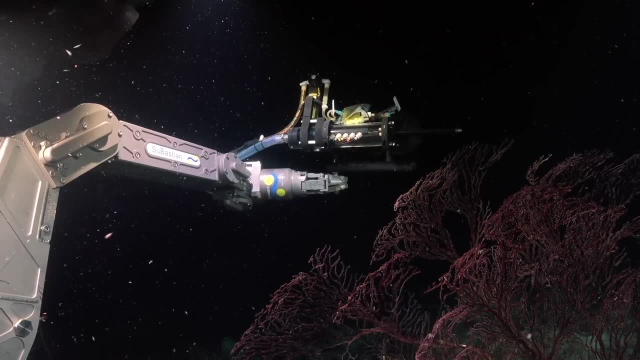 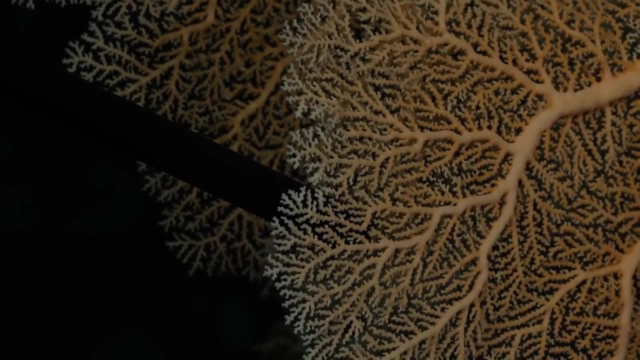 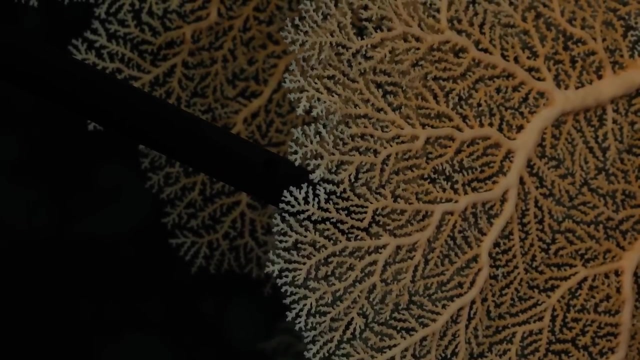 And, as a result, Solaris was born. This has been a really great deployment of Solaris in highlighting its capabilities, being able to span deep ocean, research in deep ocean environments and ecosystems, And so I think what's really exciting is that this is going to springboard us into a whole 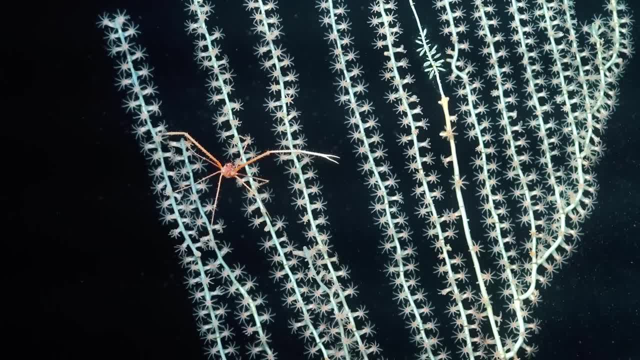 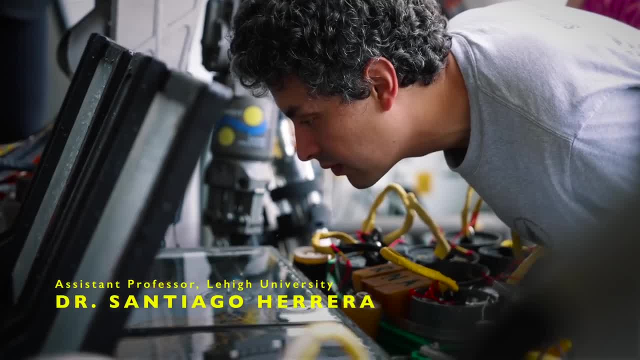 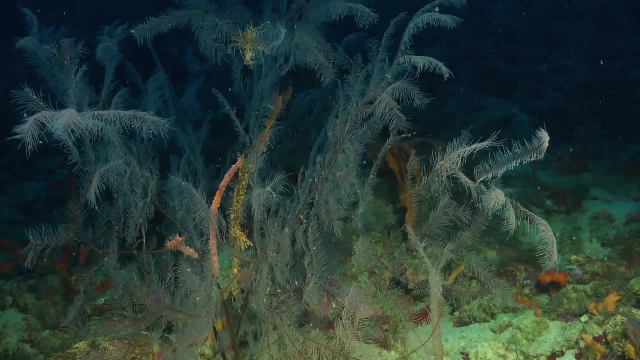 new area of understanding the biogeochemistry of corals. It's been a really successful cruise. We've collected, I think, something around 300 specimens of corals and associated animals. We've actually collected six out of the seven black coral families, probably somewhere in. 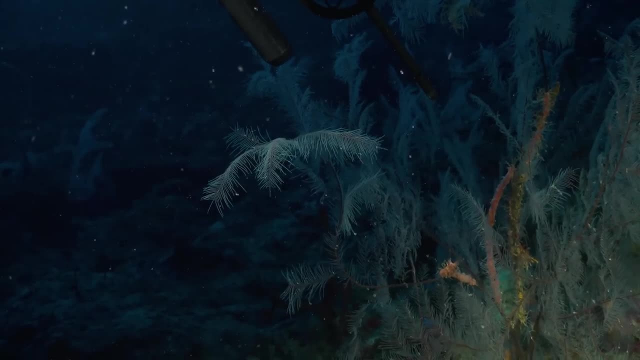 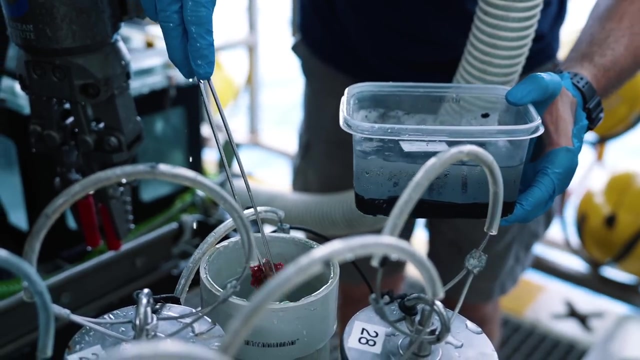 the realm of 15 to 20 species, and some of which are absolutely going to be new to science. I think so We haven't seen one like this yet. Some of the really interesting things that we've found that come to mind. 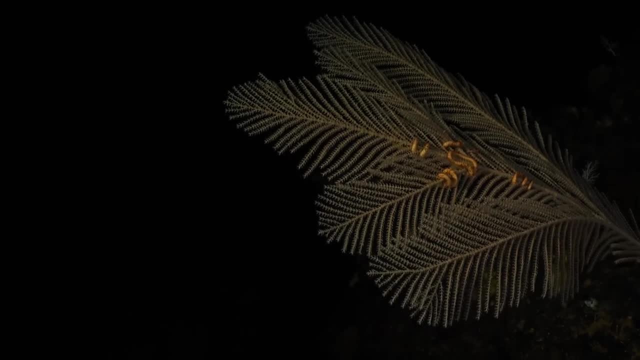 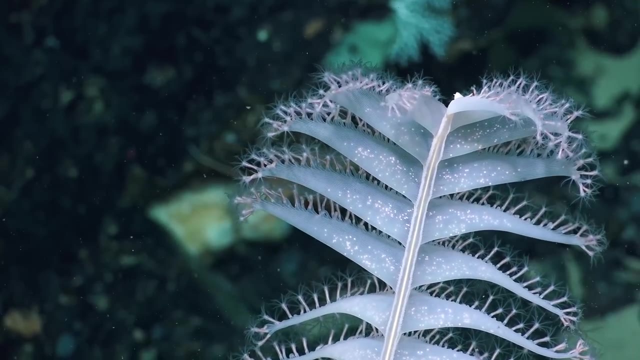 Some of the really interesting things that we've found that come to mind. We've had this super high density of corals at the Desachio Ridge. We had this spectacular discovery of hydrocorals and stony corals. that was just super coral-full. 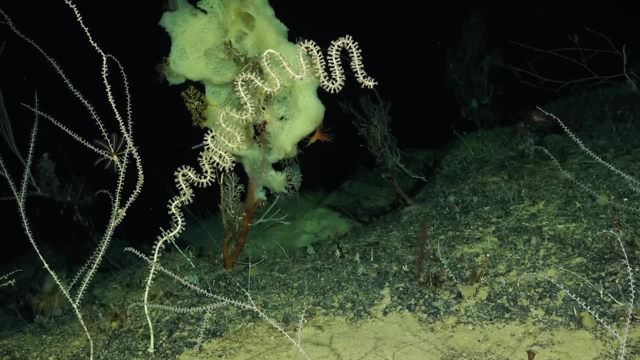 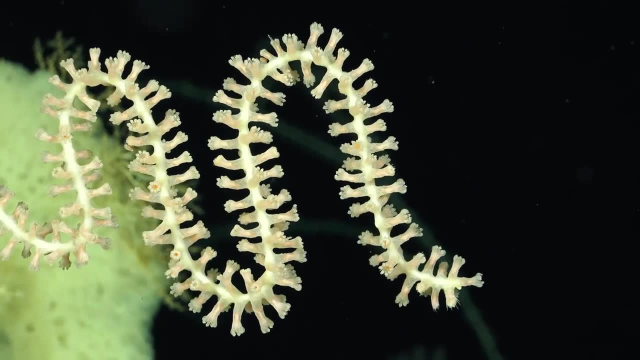 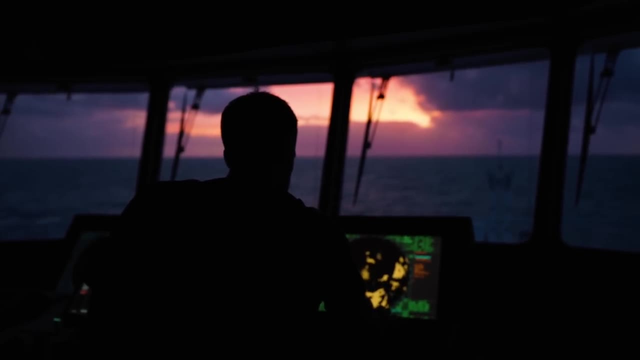 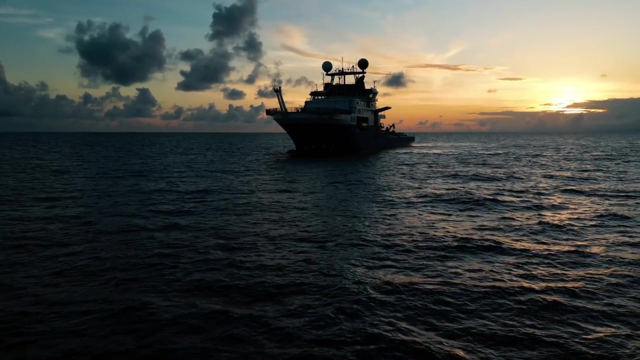 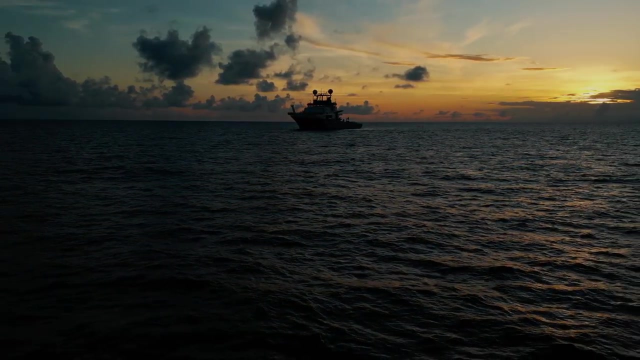 and totally unexpected. It's likely that we have multiple new species to be described, as well as information that could be very useful for proposing new marine protected areas. Of the numerous cold-water reef sites known to science, there are some that stand out for both their complexity and the challenges they pose for research. 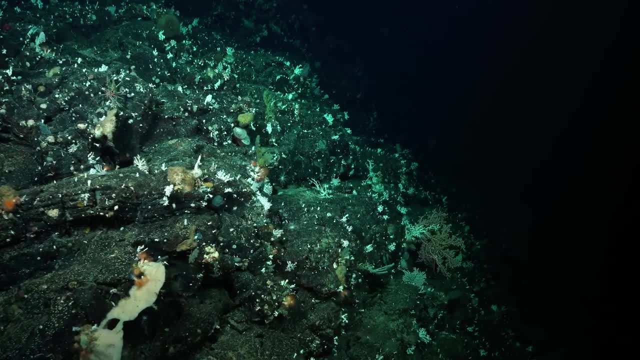 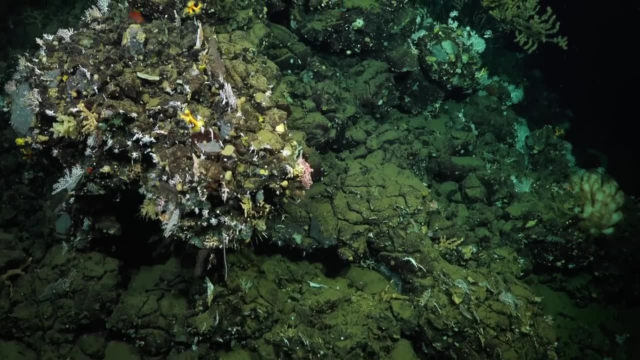 In the Galapagos, vertical reefs cling to undersea cliffs and support abundant life. However, their orientation is different. It's not always the case. It's not always the case. The depth of the ocean and depth makes them inaccessible to downward-facing ship-based. 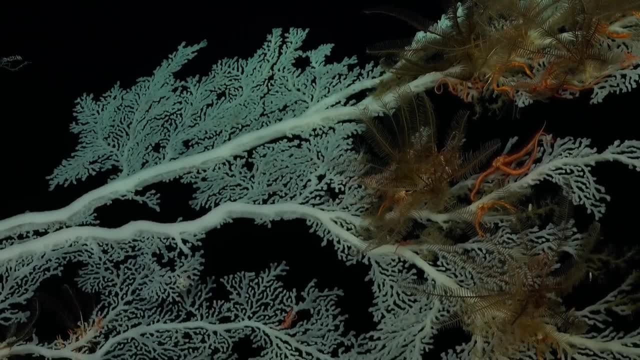 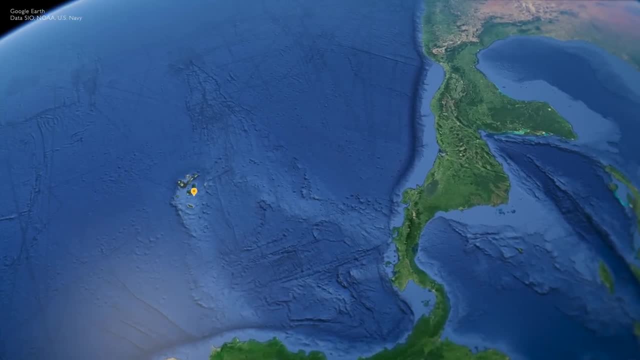 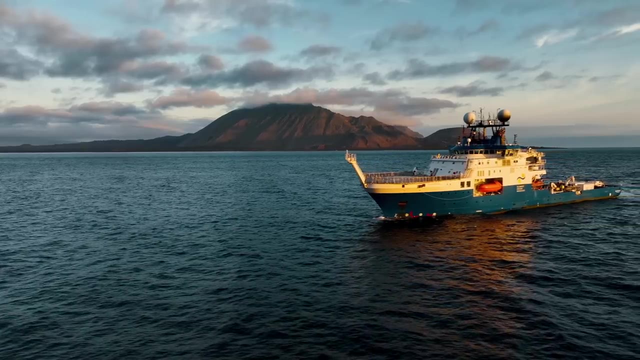 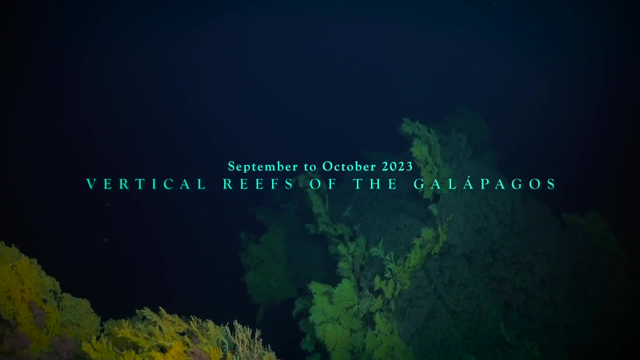 sensors that scan the sea floor horizontally. A multidisciplinary team led by chief scientist Kathleen Robert took FALCOR2 out to overcome these challenges and map the vertical oases of the deep Galapagos marine reserve. It's important to study deep sea corals because they tend to be oases of diversity. It's important to study deep sea corals because they tend to be oases of diversity. Very often when we go down to see these corals, the more we look, the more species we find. The more we look, the more species we find. 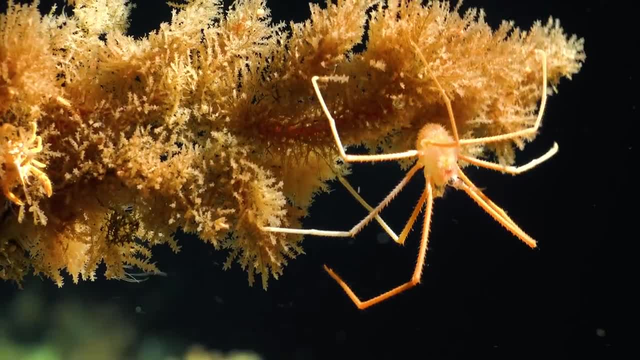 Vertical deep-water coral reefs are areas where, essentially, corals live on the side of an underwater cliff. You're walking in a forest and then suddenly the whole forest just flipped up on its side. So everything in that forest that lives on those trees were still there, but they were. 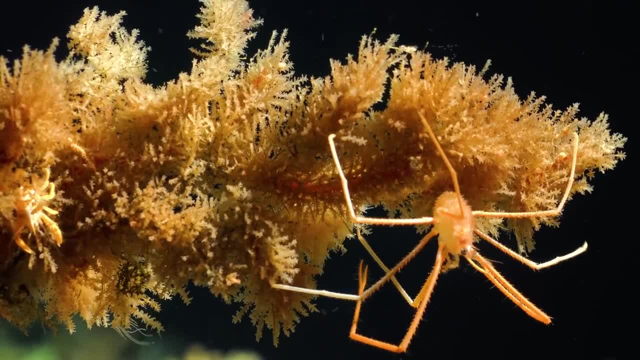 completely turned around And that's pretty much how corals are organized. And so we're going to look at the deep water coral reefs and we're going to look at the coral reefs that are located in the deep water coral reefs. We're going to look at the deep water coral reefs that live on the sides of an underwater. 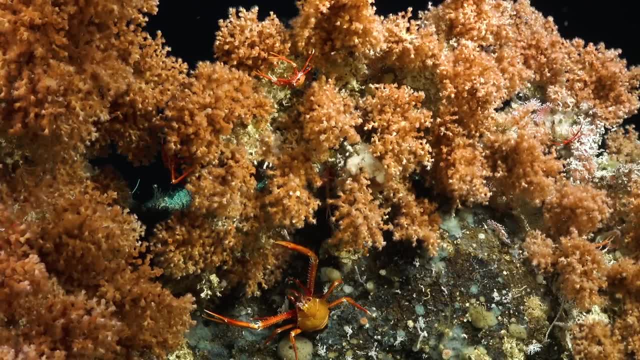 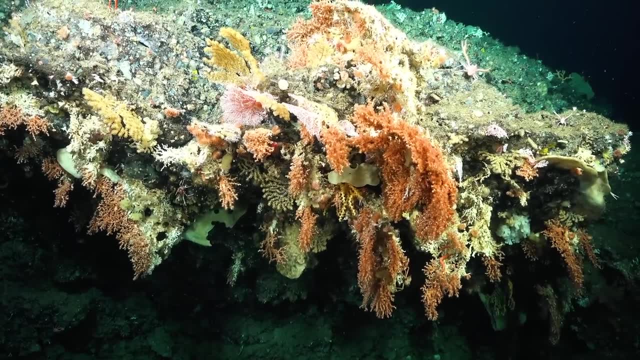 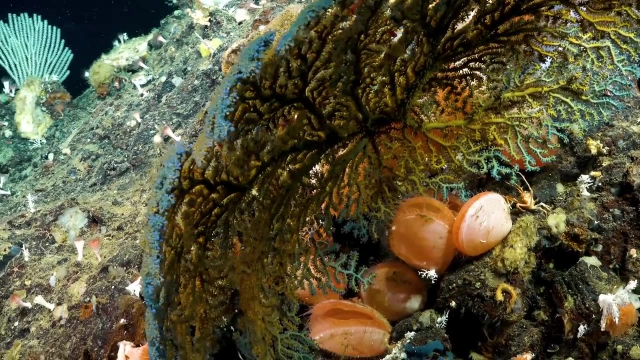 cliff, underwater cliff. You're walking in a forest and then suddenly the whole forest just flipped up on its side. So everything in that forest and lives on those trees were still there, but they were completely turned around, and that's pretty much how corals are organized along some of these underwater cliffs. 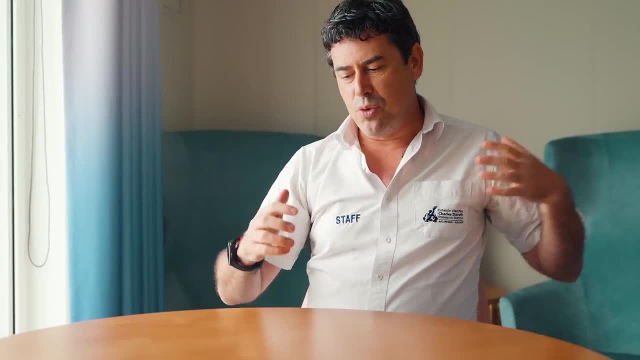 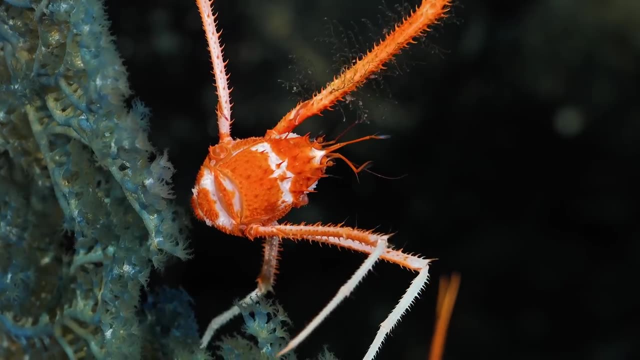 And then if you could imagine that in that forest there was a wind which was always blowing, That's like the current that we have underwater and that current is what brings food and supports the animals and the corals which are living across those vertical reefs. 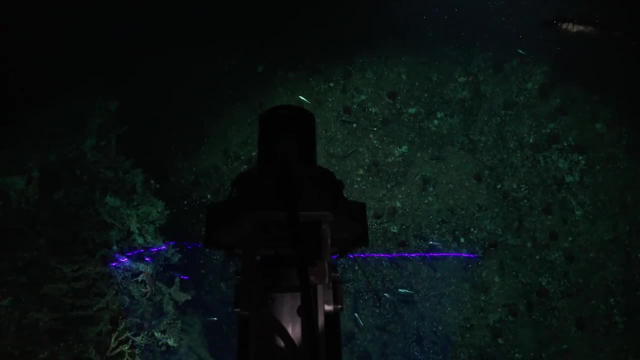 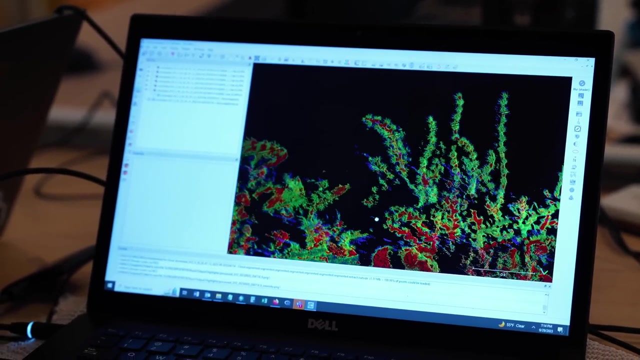 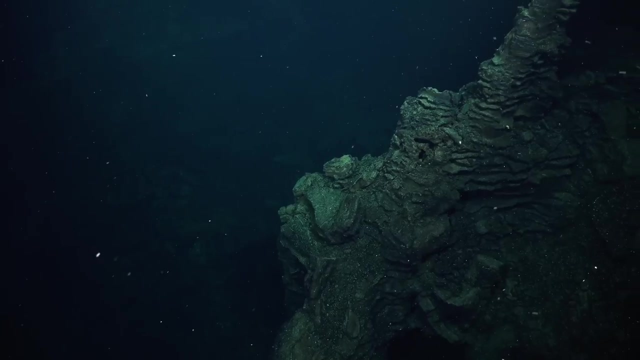 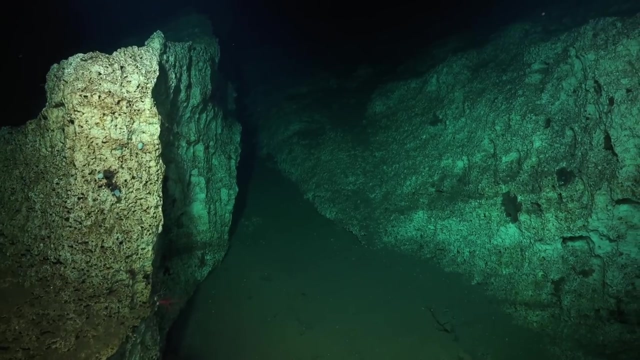 New advanced laser scanning technology allowed the team to produce highly detailed three-dimensional maps of the reefs at a resolution of two millimeters, in association with the coral. What we don't sometimes realize is that under the water we have this amazing topography. So you have valleys and hills and mountains, ravines, crevasses. You have. 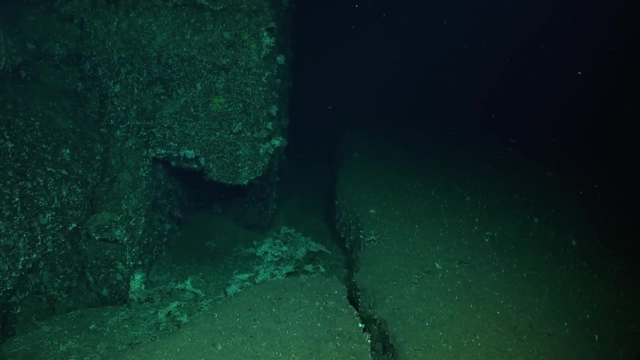 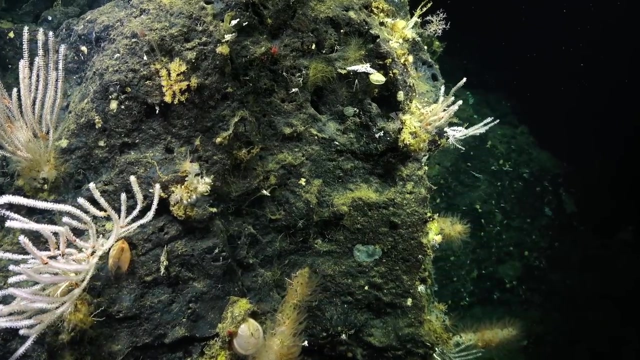 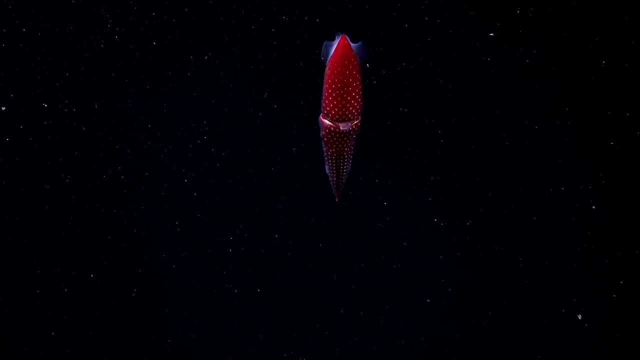 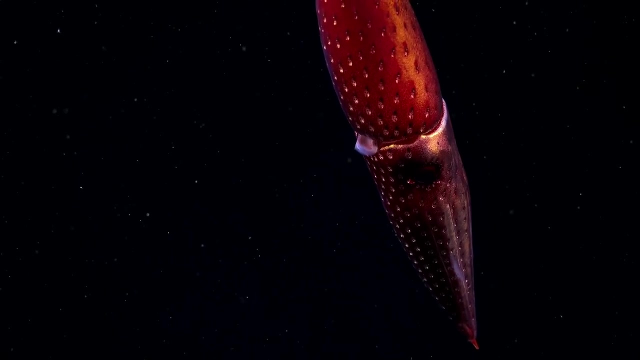 places where continental plates are rubbing against each other and that creates an entirely new space. So it's a big three-dimensional connected area. I'm amazed that every time we put instruments in the water and we have a chance to be able to go deeper than we've been, we always find something new. 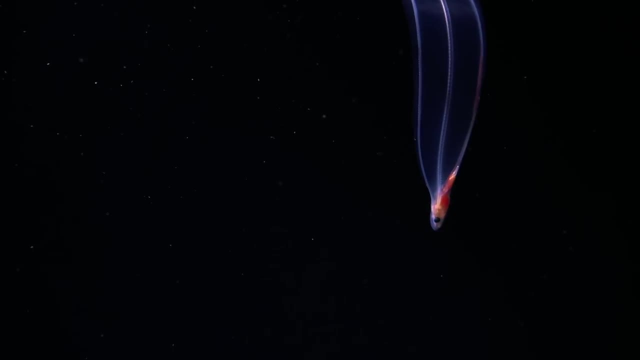 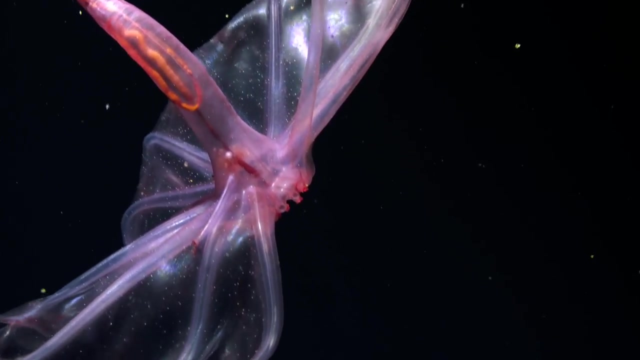 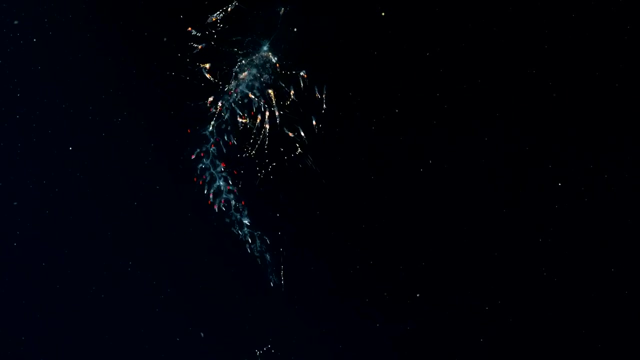 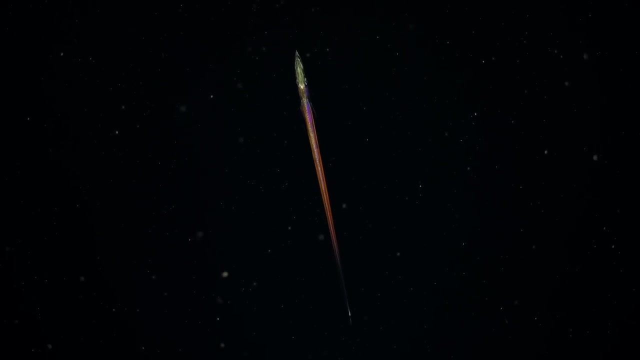 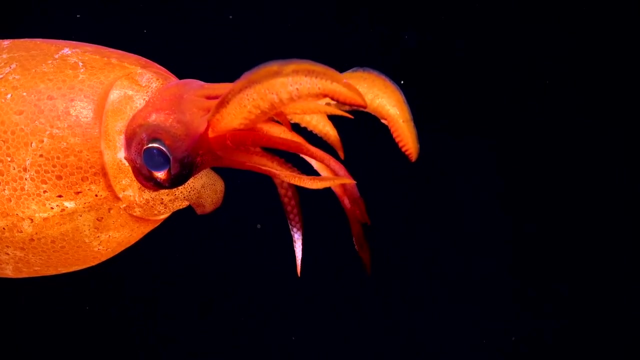 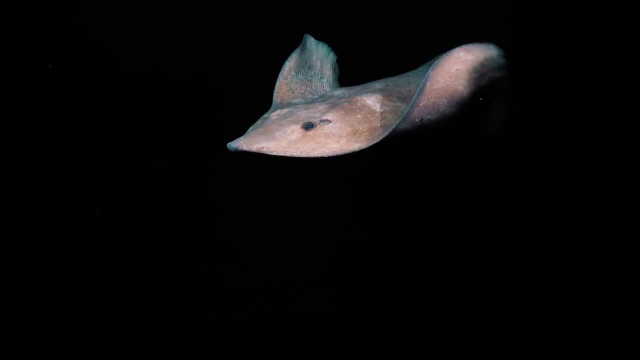 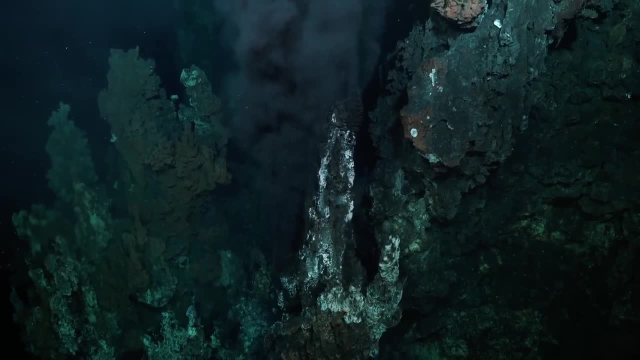 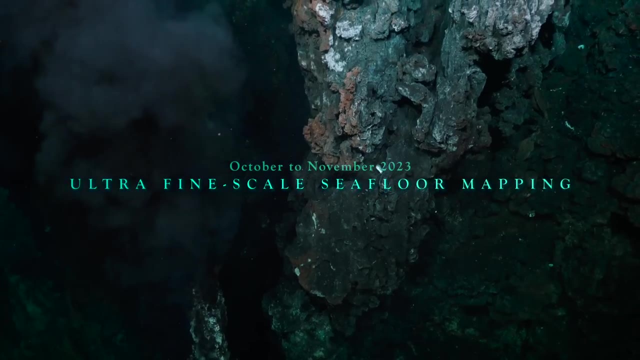 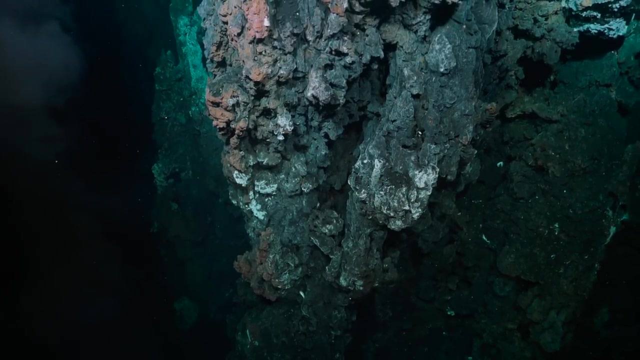 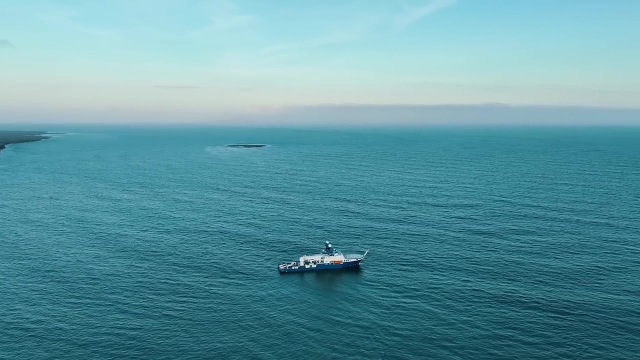 Creating high-resolution maps documents their current condition in a slice of time. In October, teams on Falkor2 tested a different approach to seafloor mapping: Interferometric Synthetic Aperture, Sonar- INSAS for short, a technology that uses sound. 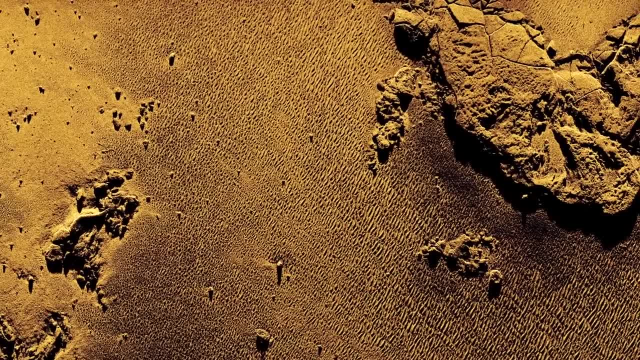 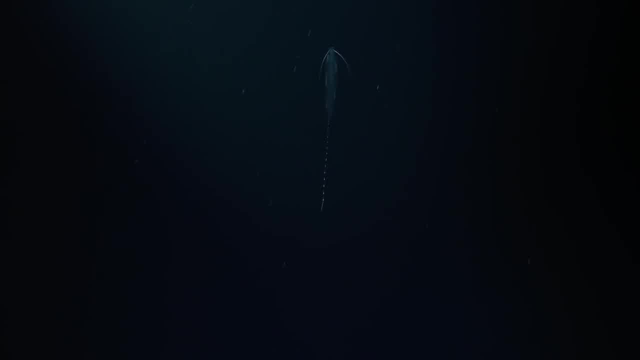 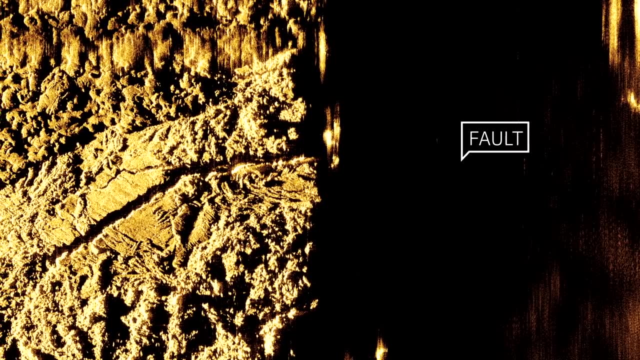 to create pictures of seafloor features at resolutions far more detailed than typical approaches to creating bathymetric maps. Normally you're often just lost and blind at the bottom of the ocean. Because we had the maps and because we had the Synthetic Aperture Sonar, we were able. 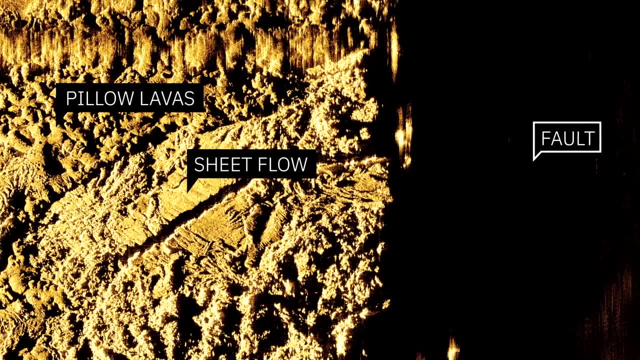 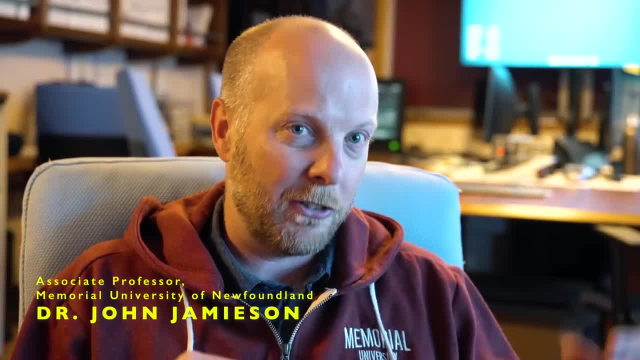 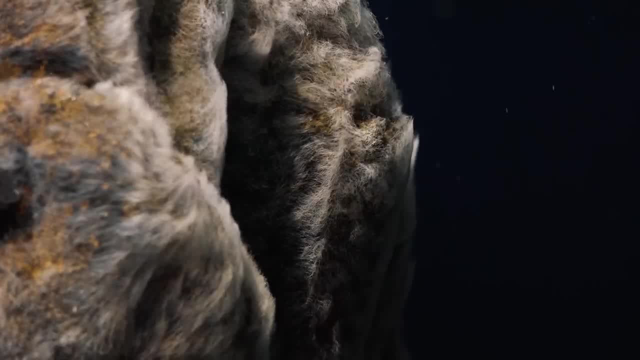 to drive with pinpoint accuracy to all the various spots we wanted to go. When you drive up to a vent with the ROV, everything is dark, but as you get closer, things start to sink. Things slowly illuminate. The first thing you always see when you approach a hydrothermal vent is the bacterial mats. 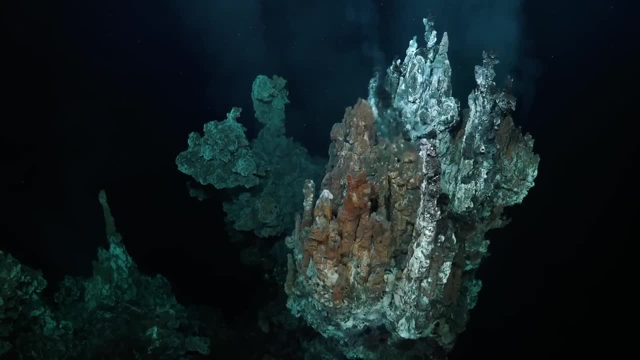 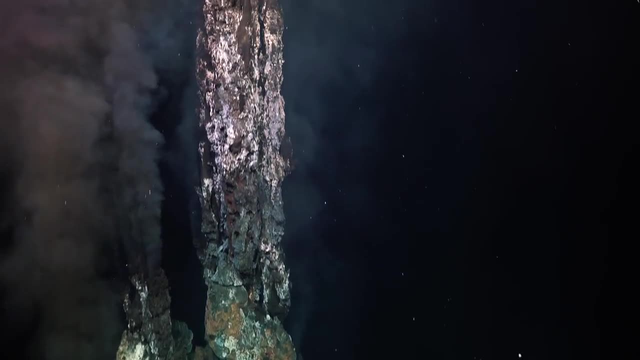 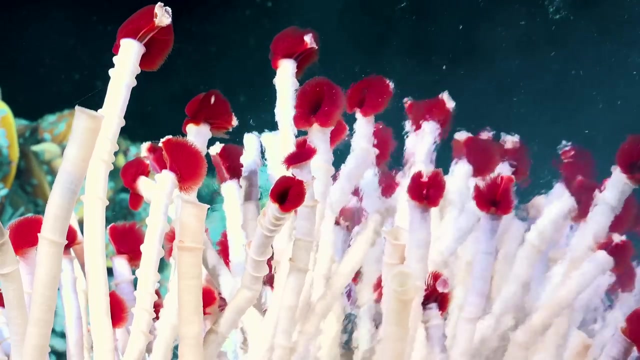 And I'm like got it Just like that. We found seven or eight actively venting complexes, towers 10, 12, 15 meters tall, The highest temperature was over 250 degrees, Two worms and all of the animals, and to me that really validated our approach. 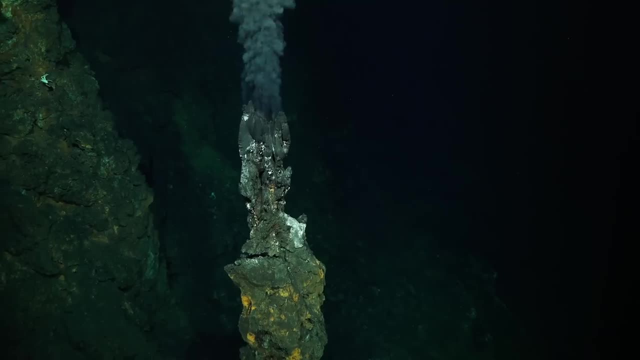 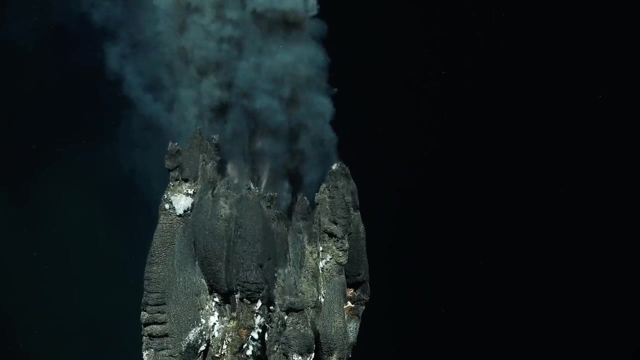 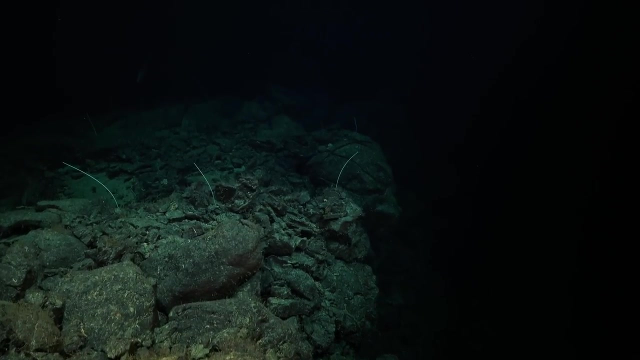 We can now see if a vent is active or inactive simply from the SAS data, Knowing the texture of the seafloor, that'll give you information on what types of animals can live there. So this could really change our understanding of you know distributions of different animals. 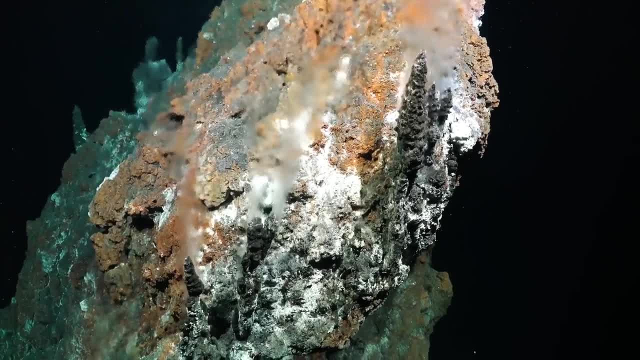 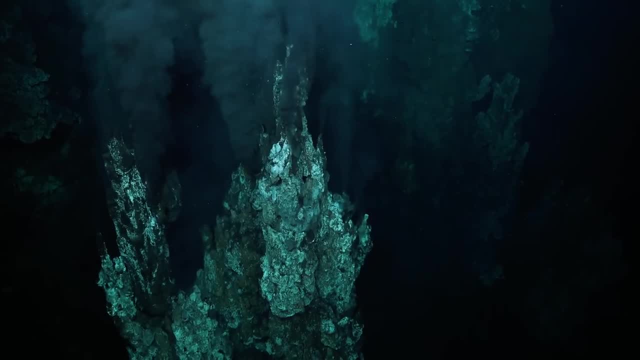 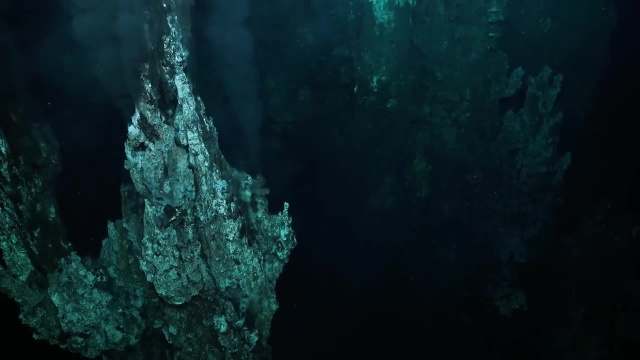 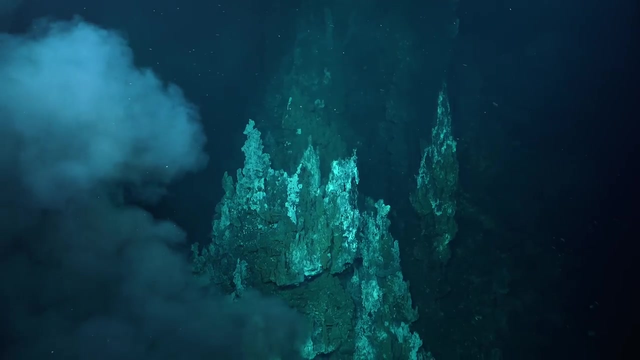 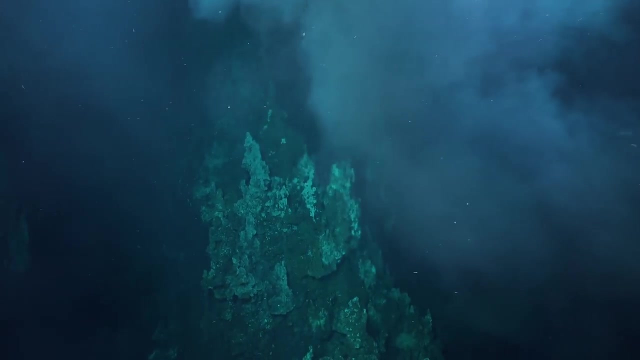 or how ecosystems function, those sorts of things. I've been in the business for 30 years and have been exploring the ocean floor for precisely these sorts of environments for 30 years, And in the early days we would spend weeks upon weeks hoping that we might encounter. 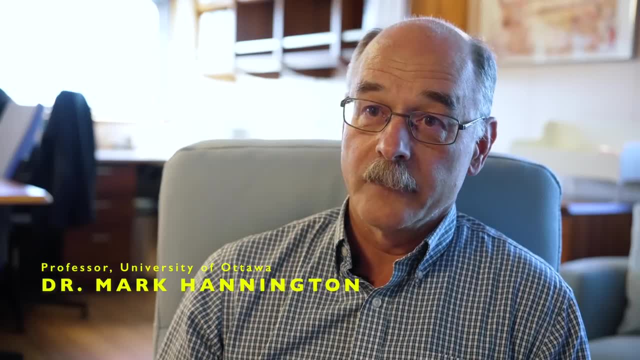 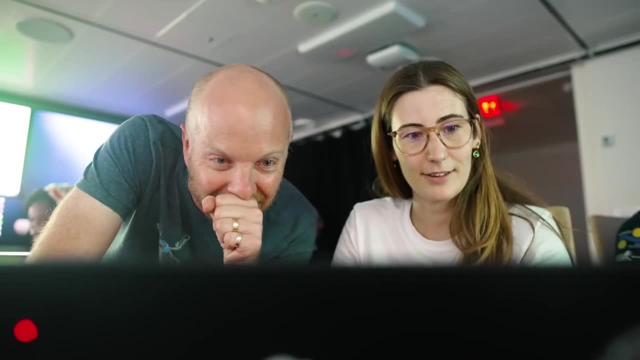 just one site, And what INSAS has done for us, And also the M3 multi-beam mapping, has allowed us to identify the targets before we even go into the water. Now that we know we can do this, there's no going back. 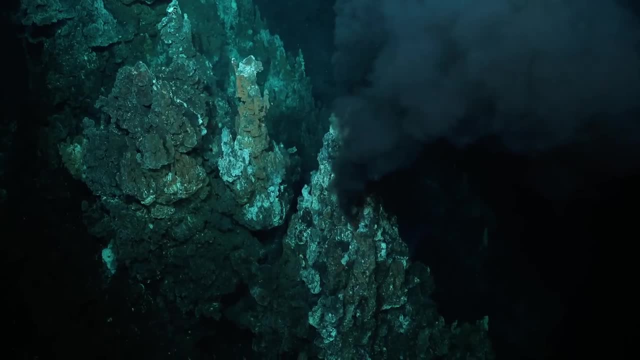 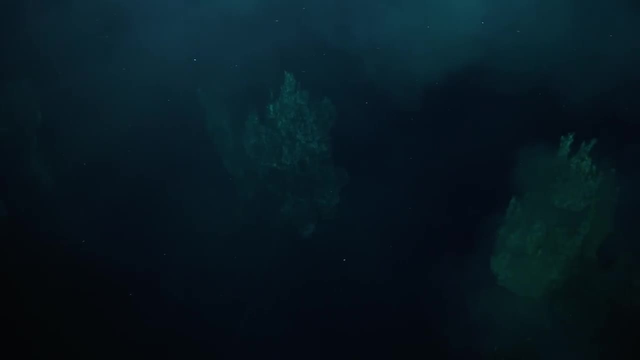 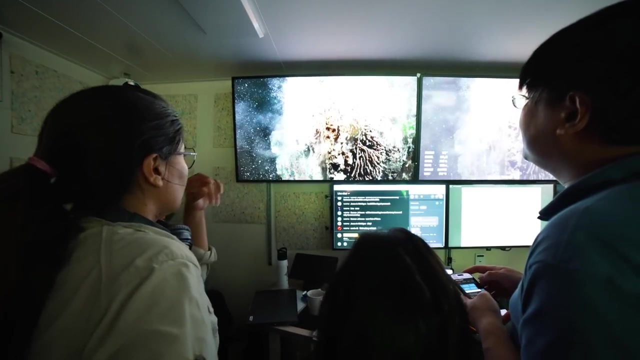 We would have discovered the value of INSAS and the M3 high resolution mapping, whether there were hydrothermal vents or not. It's just that we got the double benefit of having this technology in the right place at the right time To be able to discover that. 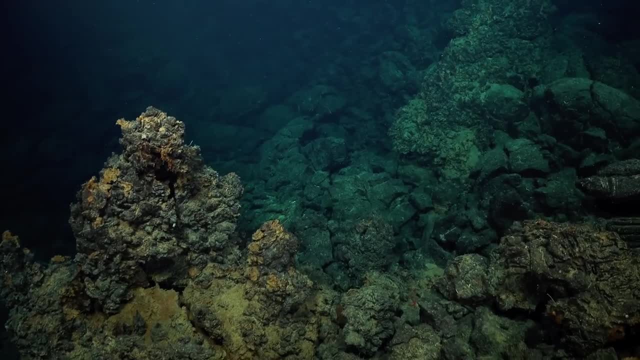 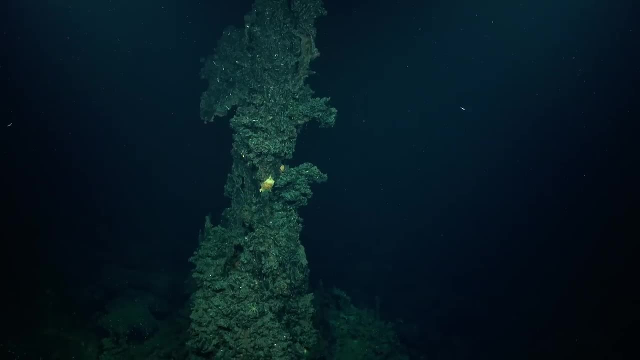 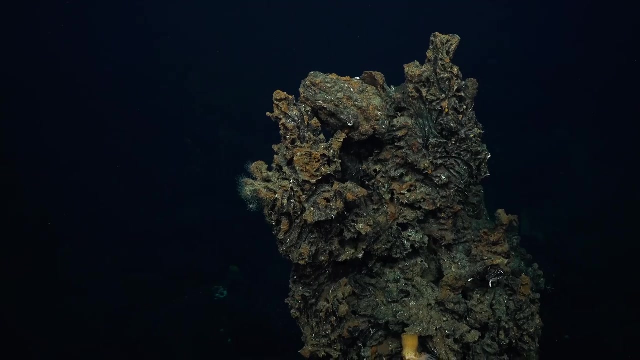 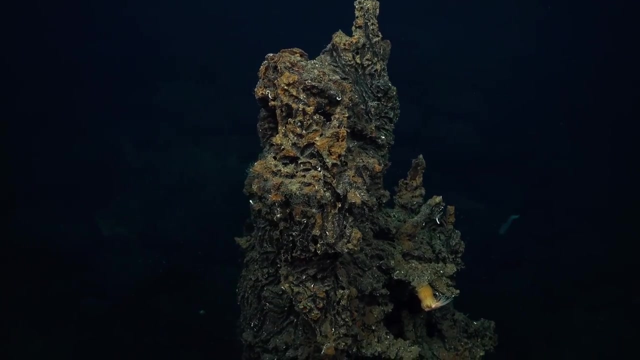 The thermal activity that we did. Creating such detailed maps of regions like inactive vents allows us to better understand the biodiversity of sites targeted by the emerging deep sea mining industry, which aims to extract valuable rare earth metals from these sites. Science and ecology has the opportunity to lead the way. 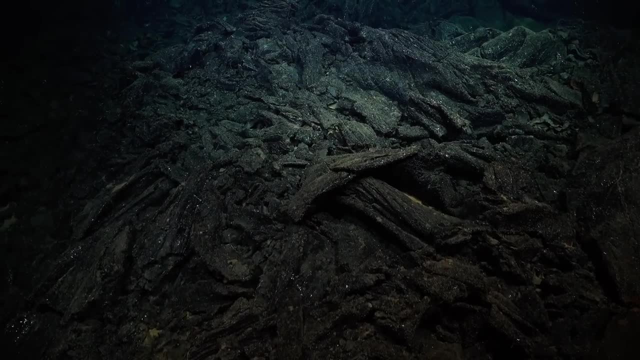 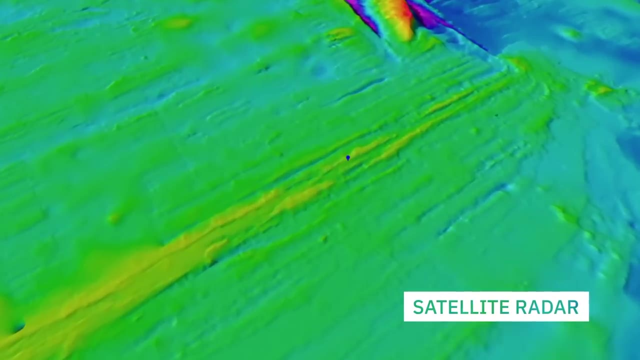 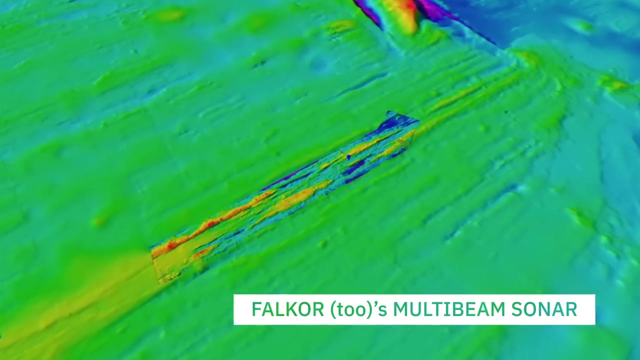 Most of the ocean has been mapped with technologies like satellite systems using radar, but those give you very coarse resolution data. We can then improve on that. We can use vessel mounted multi-beam. That gives us better data, but it's still relatively coarse. 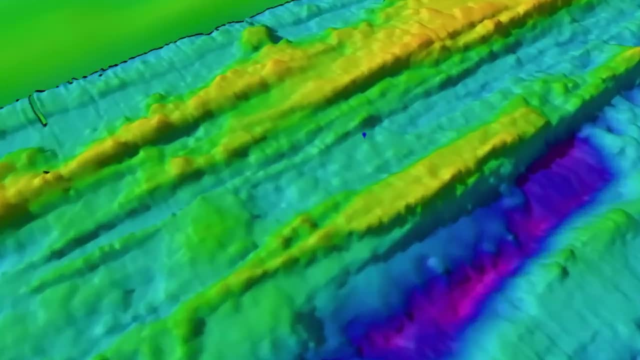 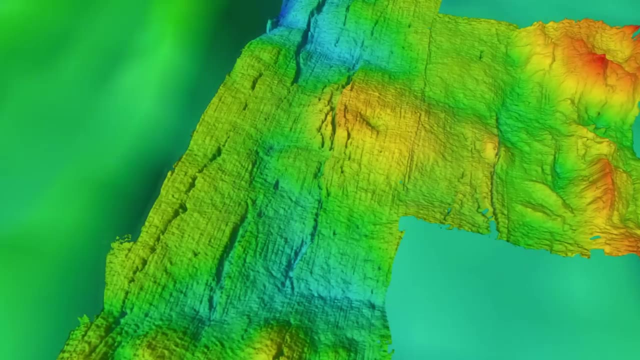 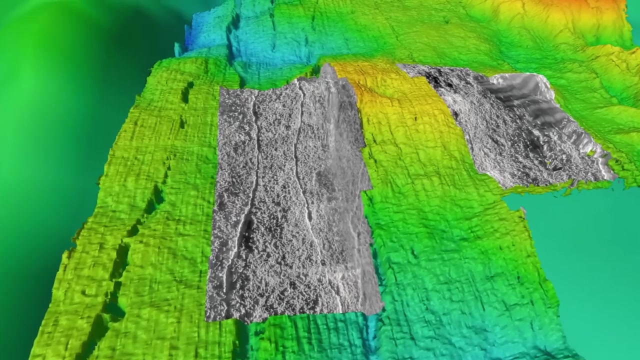 So we've been improving that. by putting systems on board the ROV, We can start to understand the morphology of the seafloor, and the SAS goes one order of magnitude more than that. So this is really high resolution. It's getting to the point where we can see some of the geological features directly in. 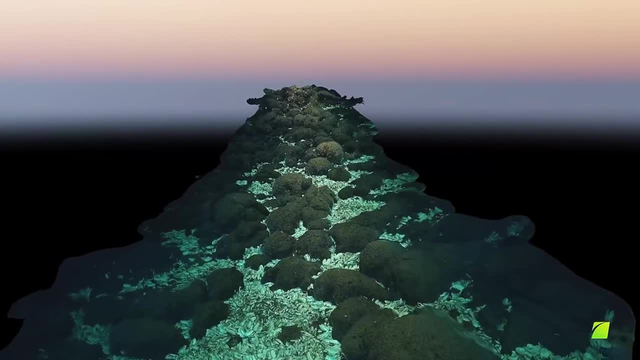 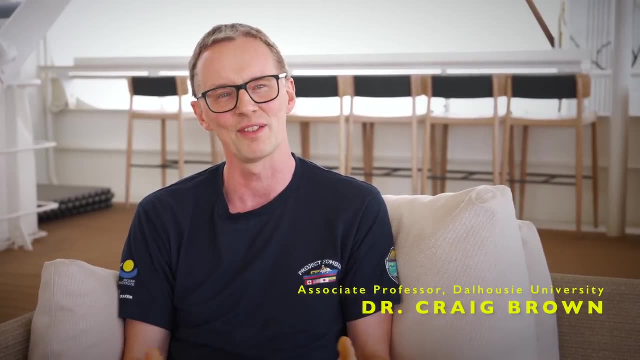 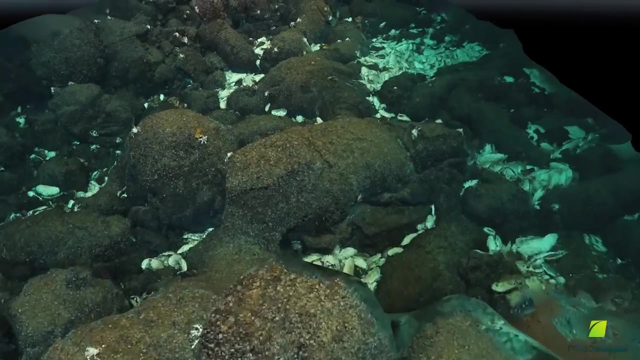 the imagery. We can then overlay photo mosaics on that and that will give us millimeter resolution, So we can start to build up a nested approach in terms of our scale and resolution, from satellite bathymetry right down to very detailed information about specific ecosystems. 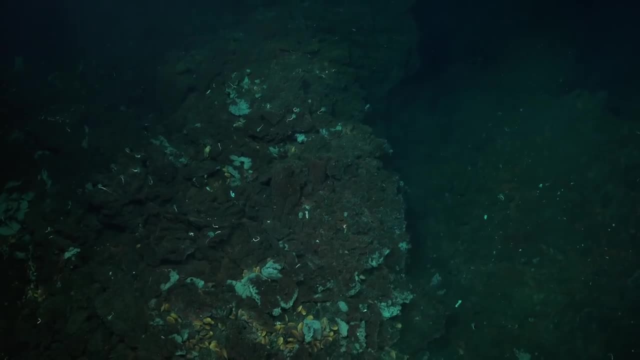 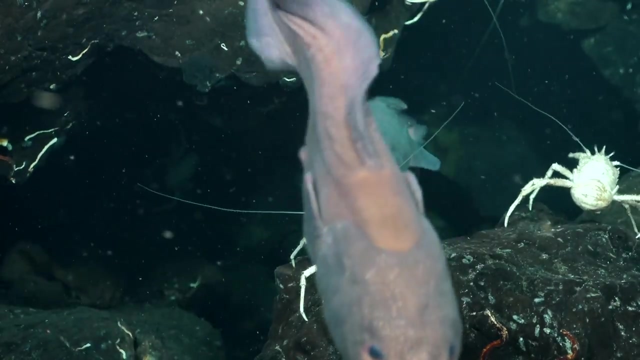 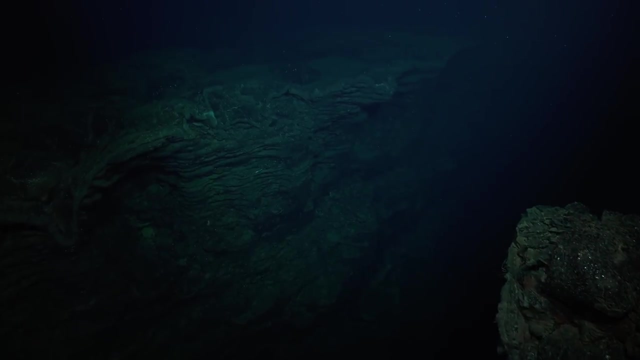 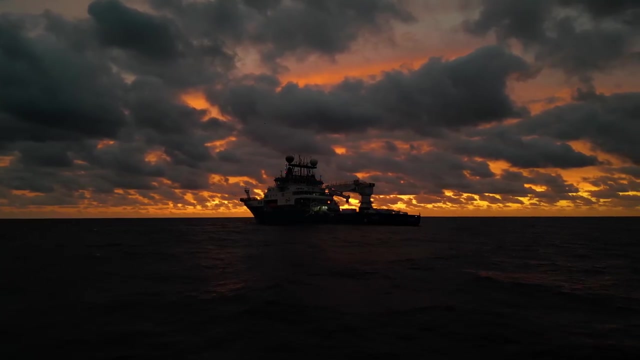 The applications of InSAS, from understanding deep biodiversity to tracking fine scale human impacts, make this a revolutionary tool in understanding the deep sea floor, But there's still a long way to go. It's a common misconception that exploring the ocean is a far simpler endeavor than space. 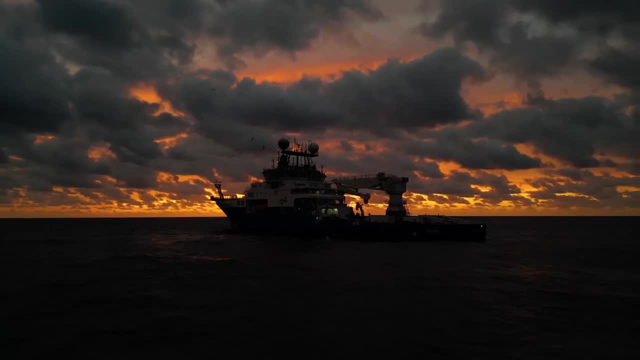 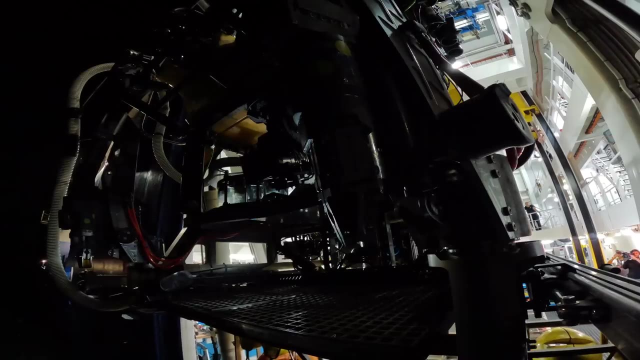 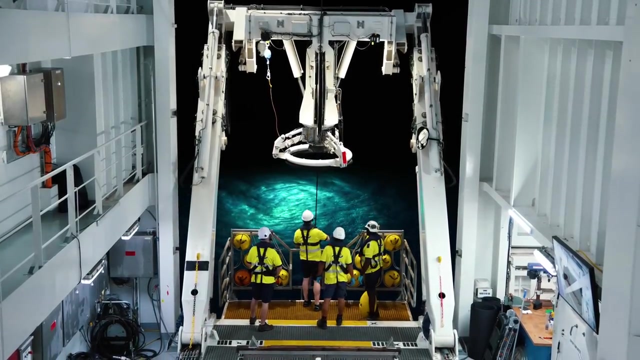 exploration. But this couldn't be further from the truth. We can't point a telescope at the waves and see what lies below, For the water conceals from view canyons and ranges that rival anything seen on land. We have to enter the depths to unlock its mysteries. 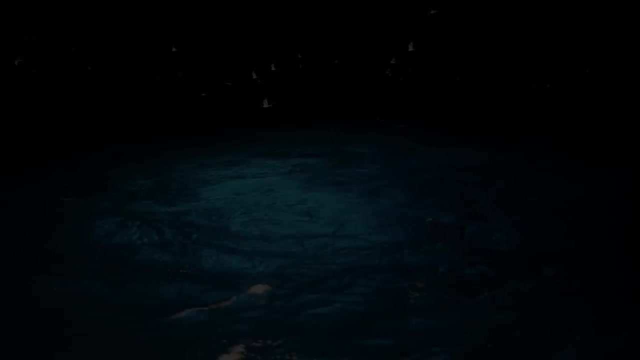 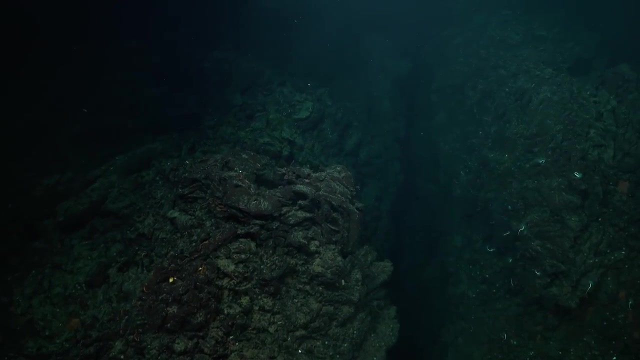 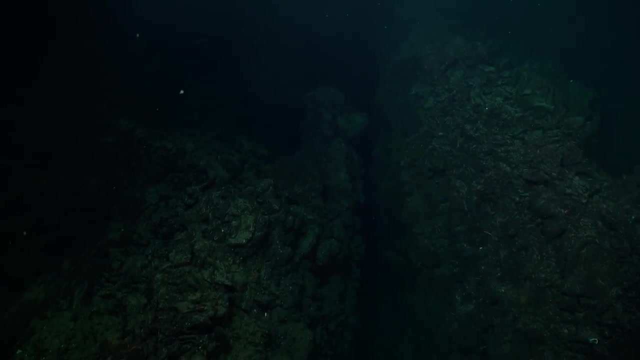 For the ocean does not give up its secrets easily. When you're exploring the deep, where the lights of an underwater robot may light up a stretch of seafloor just tens of meters ahead, You can never be certain what new discoveries lurk beyond the wall of dark. 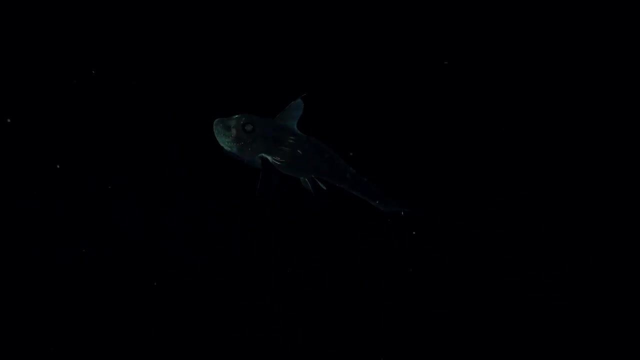 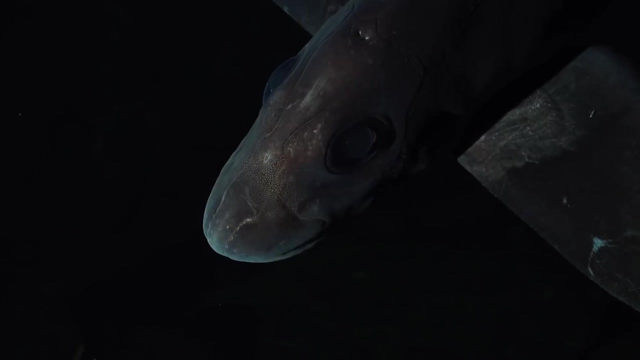 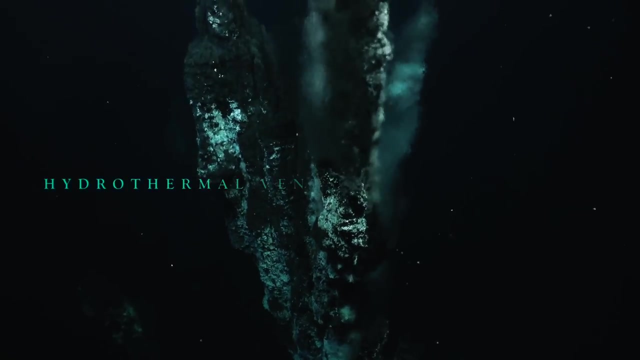 Sometimes there are clues, though it takes a keen eye and an intimate knowledge of the depths to spot them. In August, Chief Scientist Dr Roxanne Beinaert and her team were on a mission to uncover the mysteries of unexplored vents at the Western Galapagos Spring. 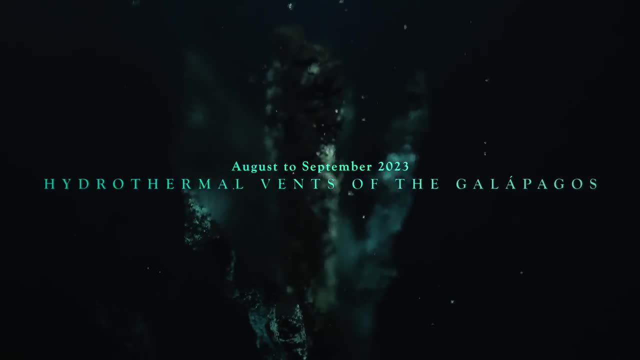 In August, Chief Scientist Dr Roxanne Beinaert and her team were on a mission to uncover the mysteries of unexplored vents at the Western Galapagos Spring. At theamic was my exposure shade and when our search looked prisoner, I saw asiit, a few hundred kilometres from the eastern side, the very region where 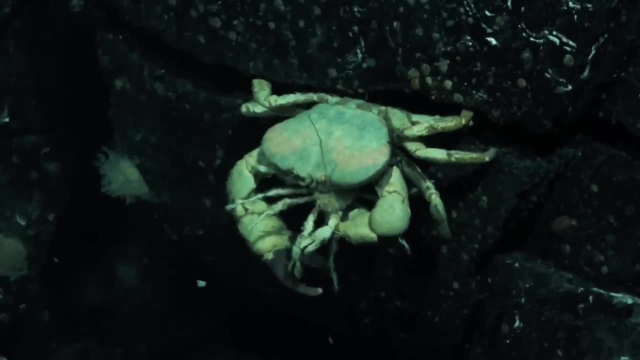 scientists first discovered hydrothermal vents in 1977.. The scientists hoped to characterise the unique communities on the western side and search for more undetected vents. After hours of searching a seemingly barren seafloor, it was the appearance of a trail. 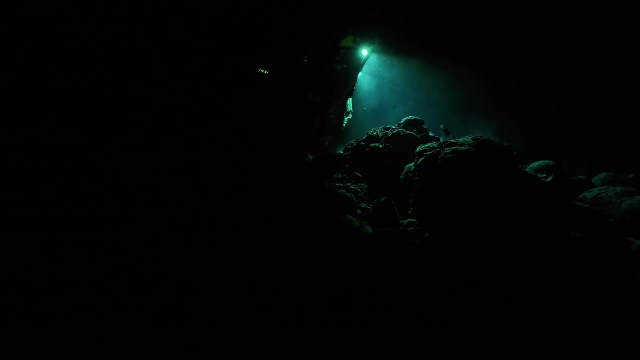 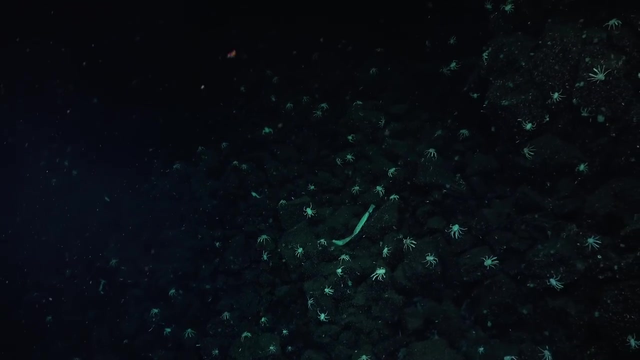 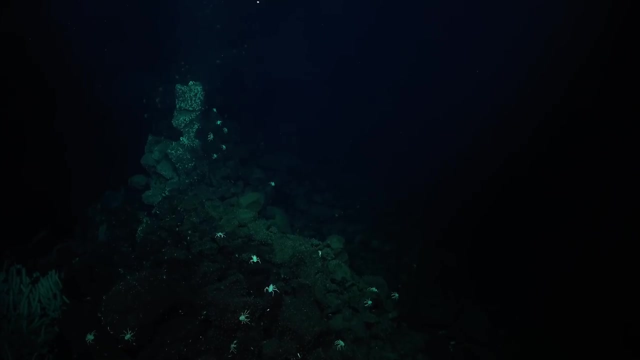 of squat lobsters that hinted at the presence of今天ness of a new vent. Finally, right before I was about to go to bed, we started seeing a lot of squat lobsters and we started noticing a lot of fissures and faulting. 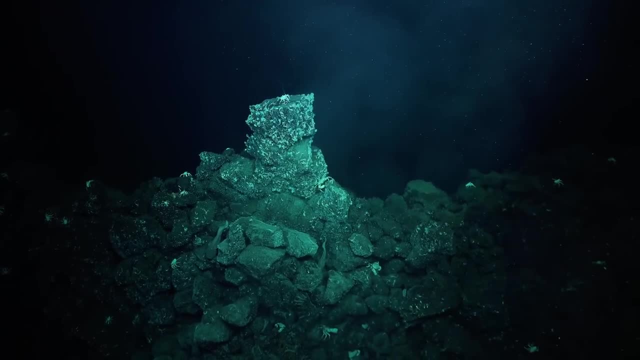 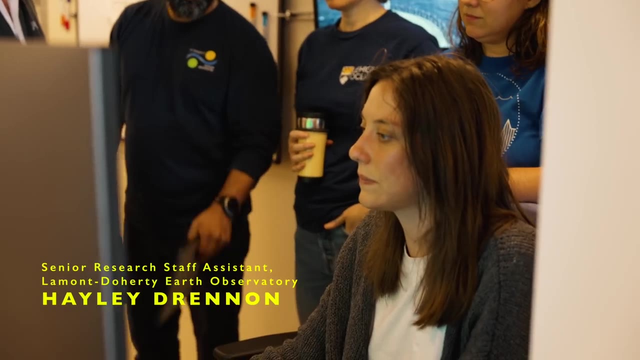 Did feel like the squat lobsters were leading us like breadcrumbs, like we were Hansel and Gretel, to the actual vent site. That's looking good now, Platform and out, When we were looking for vents from the surface, it's the equivalency of being on Mount Olympus. 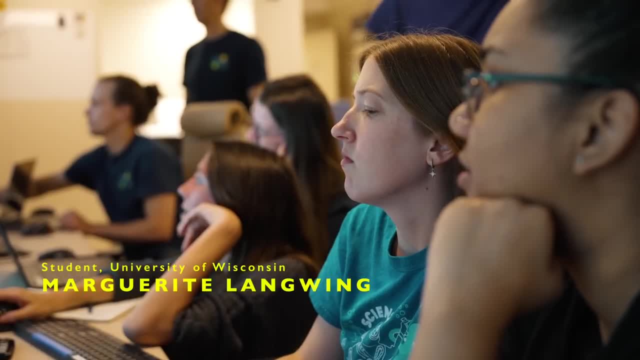 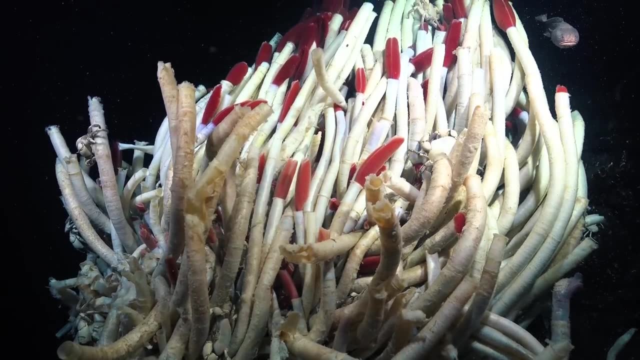 and looking for a football post. The first thing we saw was a big group of Riftia popped up on the screen, which is unmistakably a hydrothermal field. I was standing right next to Roxanne, and so we both smiled and looked at each other. 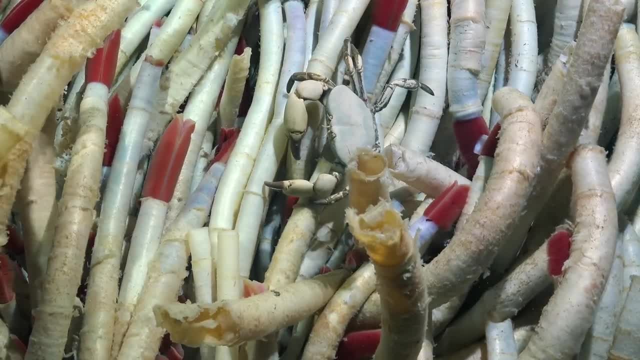 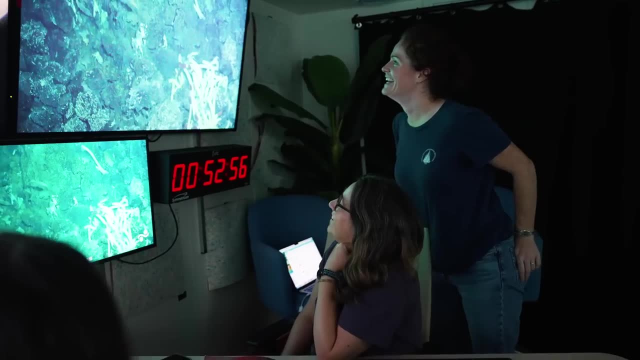 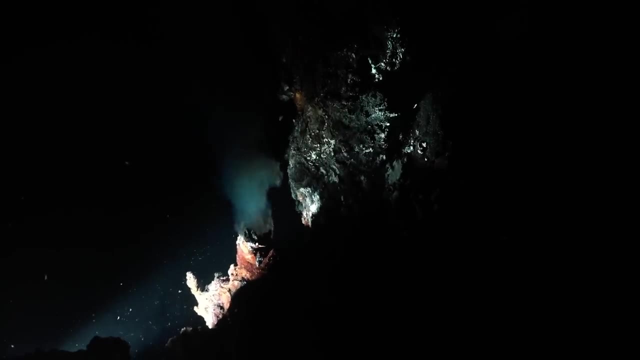 and we found it. it's right there. You know, these are unique ecosystems that are unlike anything else on Earth, and we're still only now trying to understand what shapes them. The trail led them to a vent field that was new to science. 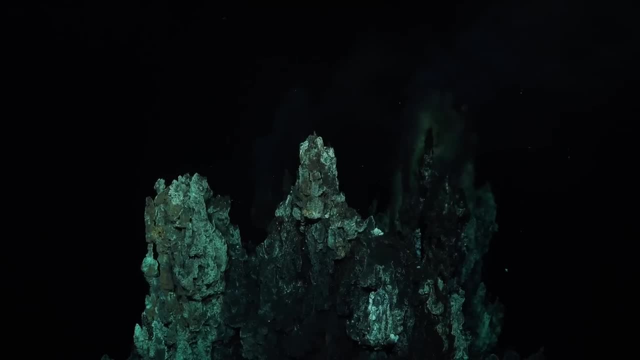 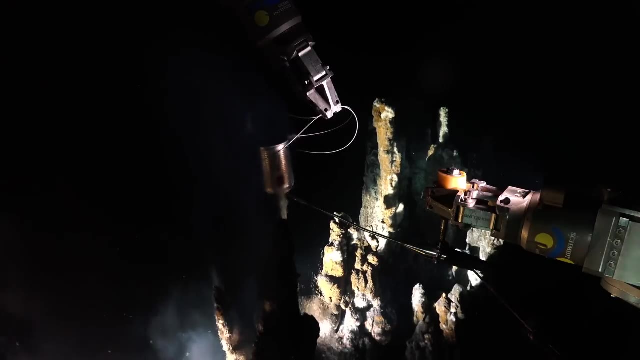 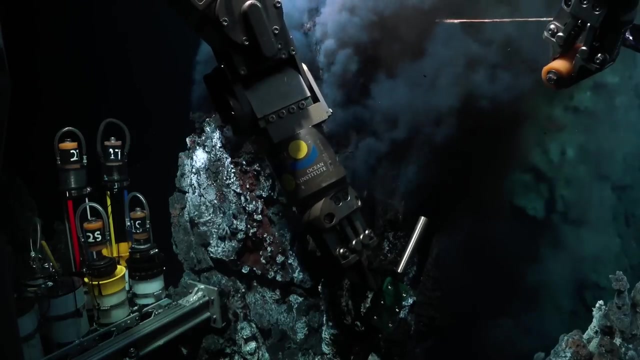 at around 2,800 meters, One of many discovered on FALCOR2. since March, We've successfully sampled across multiple disciplines at the sites, ranging from chemistry to geology to biology. We've collected the first ever high-temperature water samples. 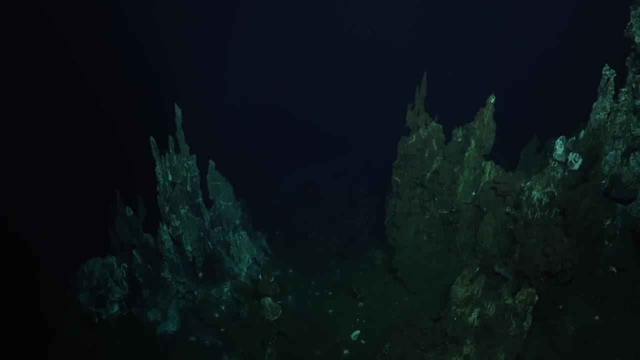 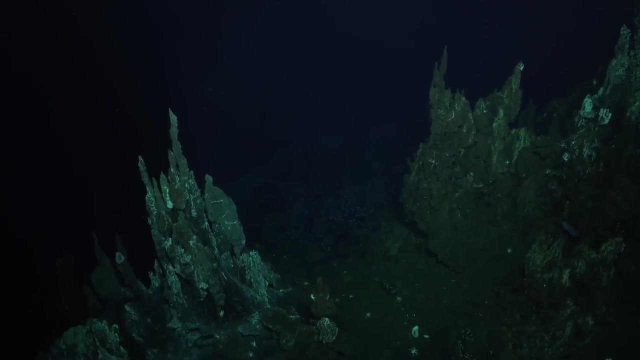 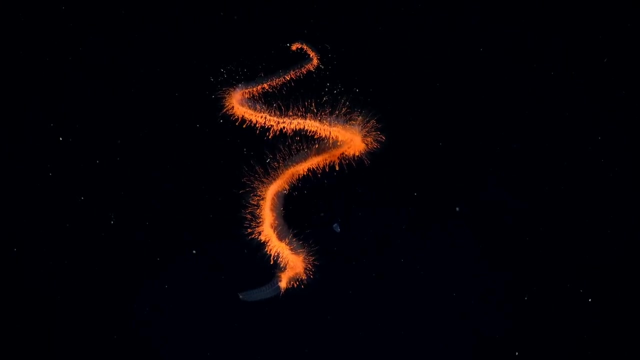 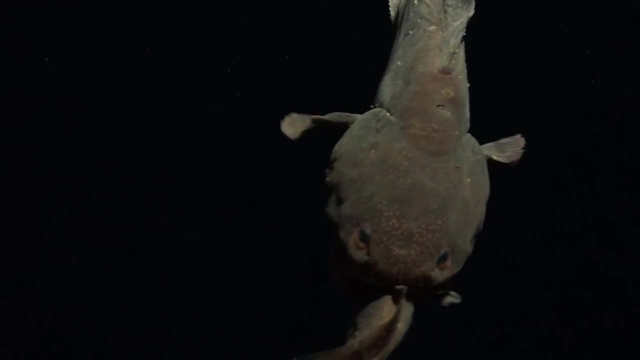 We've been able to build the most comprehensive data set ever for this location. 80% of our planet's living space is the deep sea, And that means 80% of our planet's living space never experiences sunlight, And it's astonishing to think that the other 20% 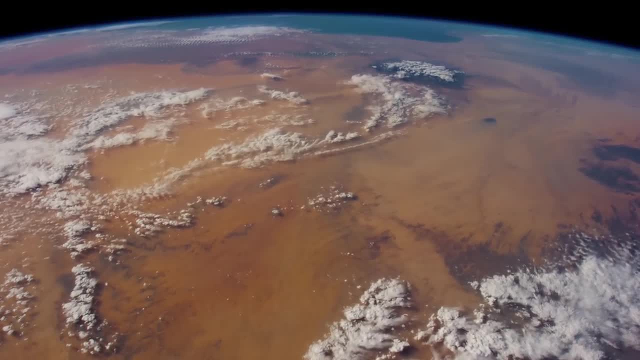 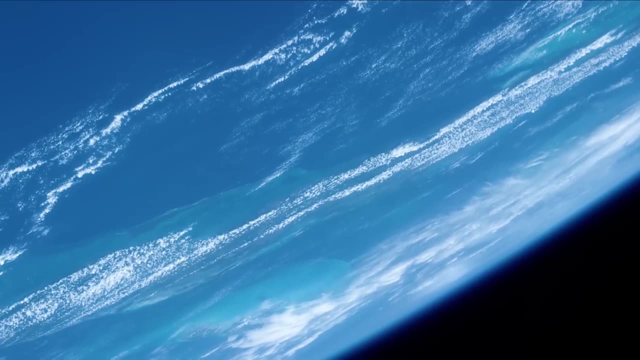 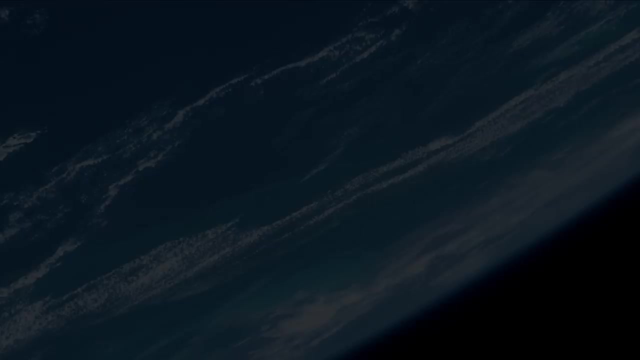 has everything else: every rainforest, every desert, Paris, Los Angeles, you name it. All of it is another 20% and it gives you a sense of just how much of our planet is deep sea. The deep ocean may be far away and out of sight. 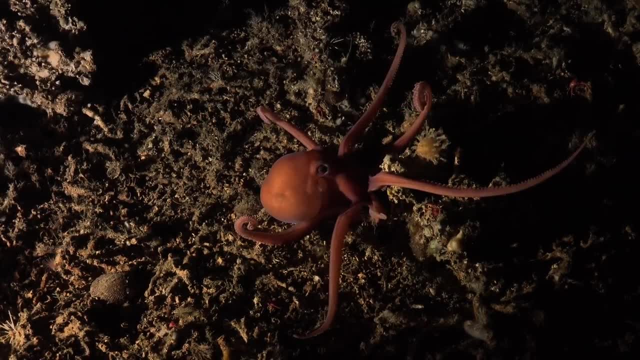 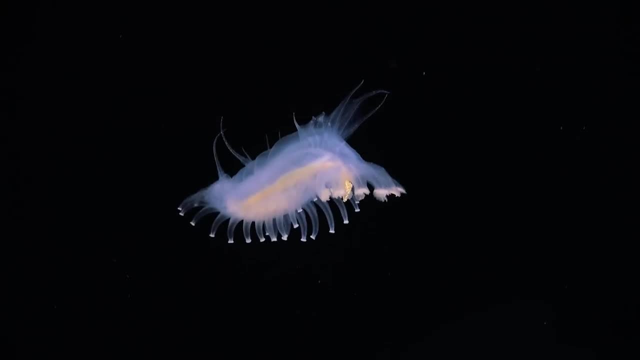 but it is not separate to our world. In fact, it is in many ways the single most important component of our planet's biosphere. Its processes shape the conditions of our climate Ecosystems, concealed away in a world of darkness. 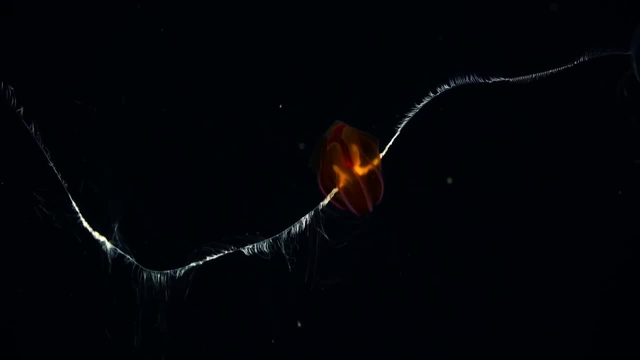 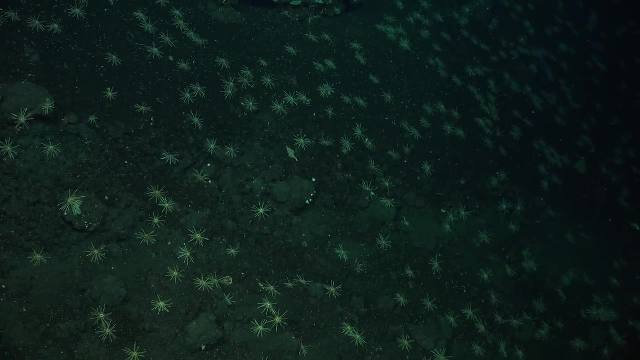 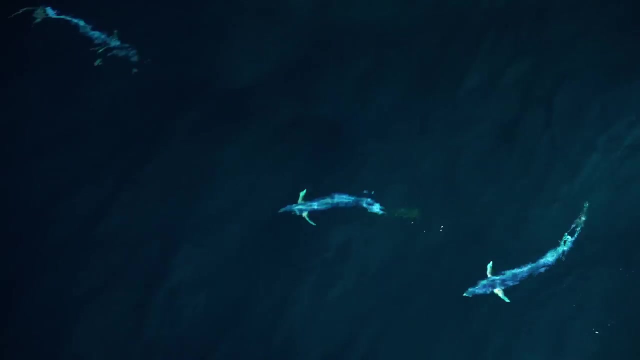 and mystery play their part in defining the ecology of entire oceans. We know more about most of the planets in our solar system than we do about the deep ocean. But the reason isn't because we haven't been curious. The reason is because we haven't had the tools. 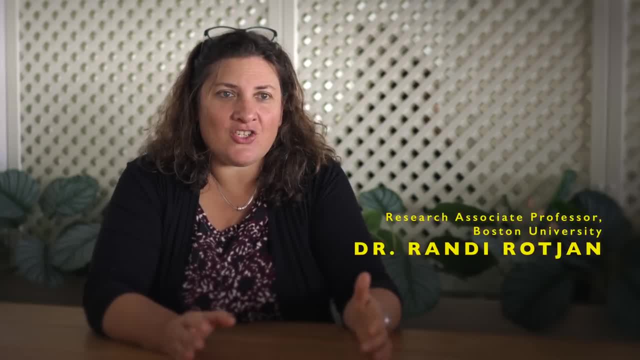 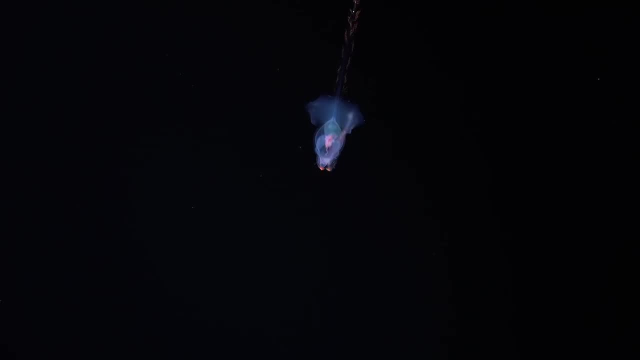 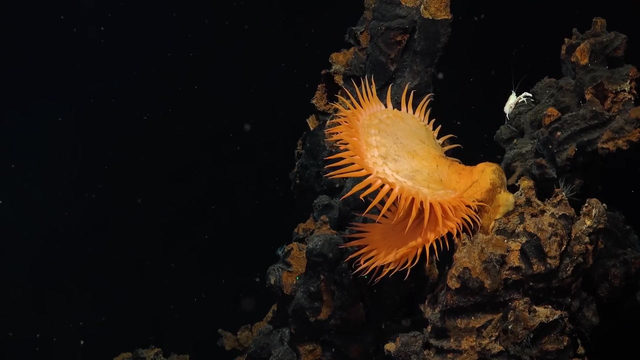 to go down and look. And we have them now. And the truth is is that every incremental step that we take to learn more about the deep ocean helps us understand more about the entire planet. What is the driver to get us to see somehow? 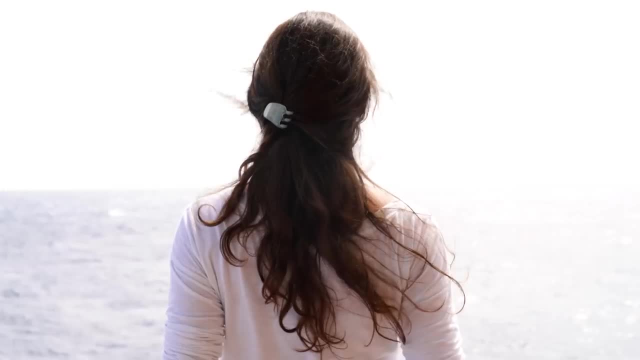 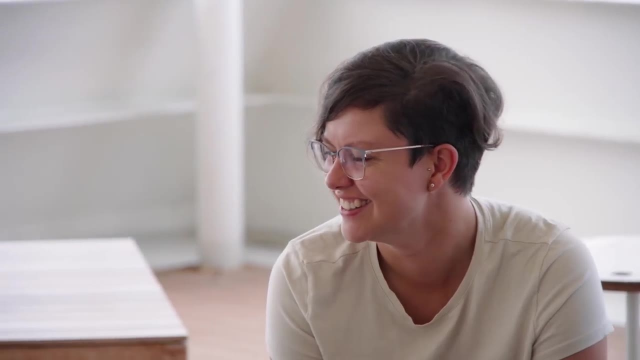 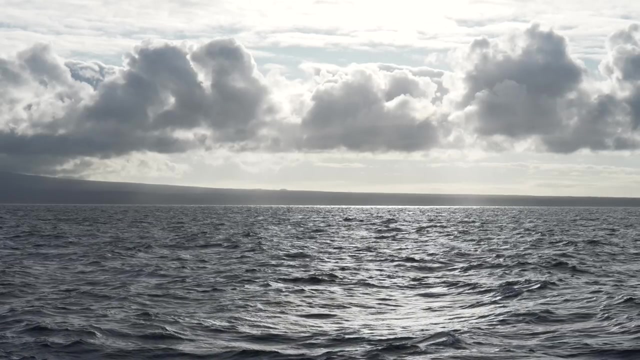 there's something about going into another world that is truly exhilarating. It's a world we don't belong in, and yet you realize how connected you are to it. We need to care about every part, from top to bottom, from what's happening in the atmosphere.